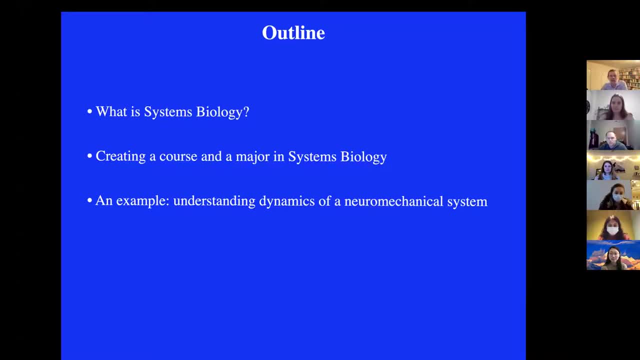 the dynamics of a neuromechanical system. so I'll talk a little bit about my own research. Then I hope you'll find this very exciting. Systems biology is really a wide open frontier. There are lots of really exciting problems, so I'll spend a few minutes talking about the ones. 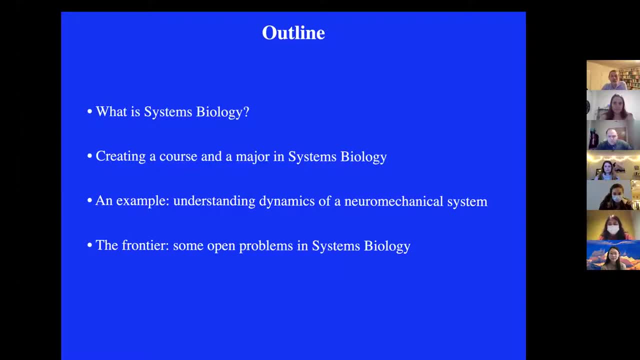 that I've thought about a lot and briefly mention a few others and then wrap up. I am highly interruptible, so if something I say isn't clear, something I say doesn't make sense, please stop. ask me a question and I will be delighted to answer. I will periodically pause. 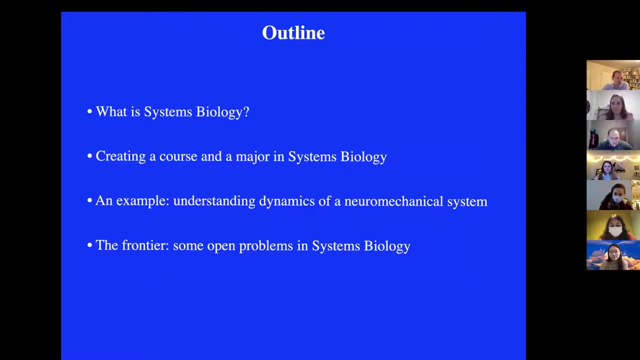 and go through the presentation, and if there are things that I think you might want to ask more questions about, I'll give you space to do that. Okay, so let's embark on this voyage here. So what is systems biology? So I looked it up. There's a nice article in Wikipedia about it. 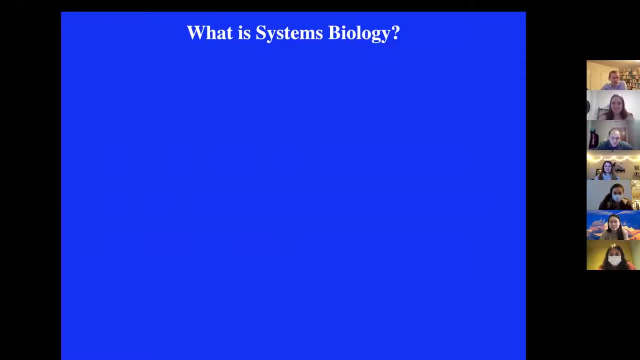 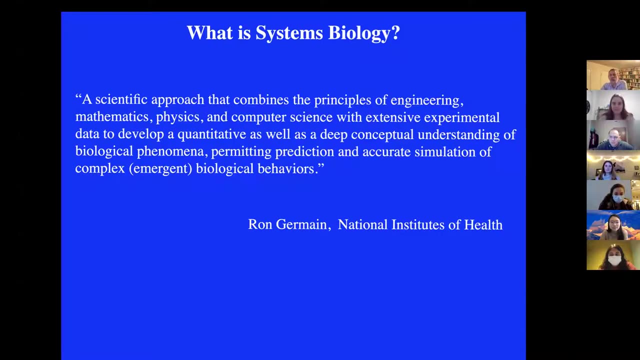 I've also read various articles. I found there was a nice quote that I liked by a guy named Ron Germain, who's at the National Institutes of Health. He actually works in immunology, but he's played a significant role in trying to get people to understand what systems biology is. So I'm going to 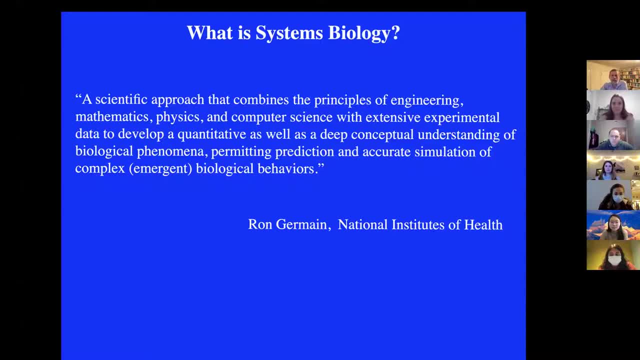 ask people to do systems biology at NIH and elsewhere. And he says the following: A scientific approach that combines the principles of engineering. Let's see, My screen here is covering part of what I want to see here. Can I move that? Let's see. Let me go back. 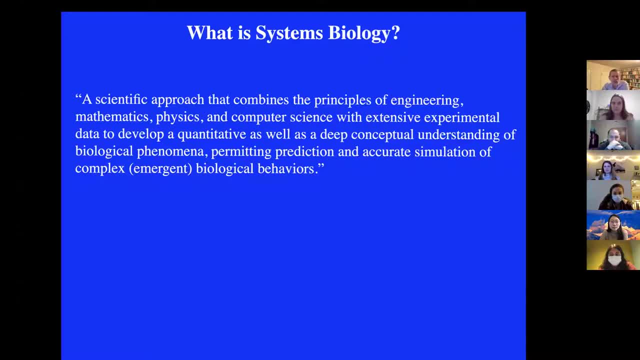 Engineering, I think- mathematics, physics and computer science. So there's several things I want to focus on here. Notice that he mentions engineering, math, physics and computer science. He also mentions experimental data. He then mentions two key things: a quantitative understanding and a conceptual understanding. 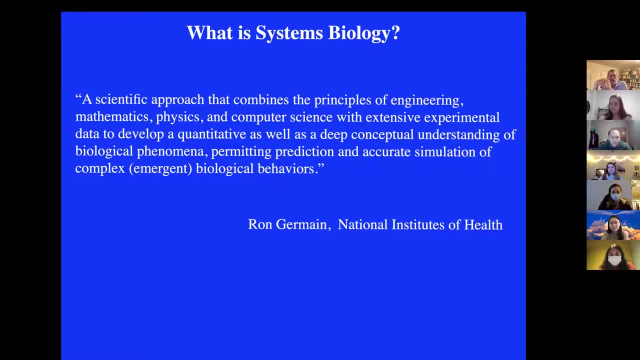 And then he sees this: the goal is to predict and accurately simulate. And then he mentions this concept of emergent biological behaviors. So I think the reason I like this quote is it actually combines a lot of different things that I've seen people talk about in systems biology and 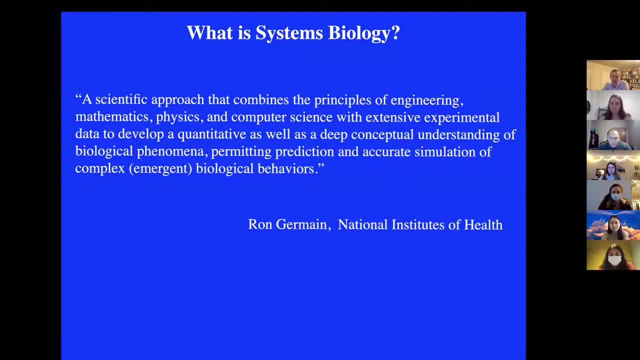 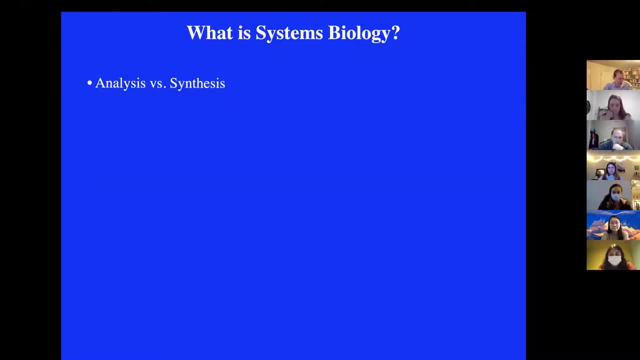 I think articulates well what the issues are. So let me talk a little bit about some of the ways of thinking about it, And the broad thing that I want to start with is in thinking about biological systems, you can take really two big approaches. One is the idea that we have to think about the 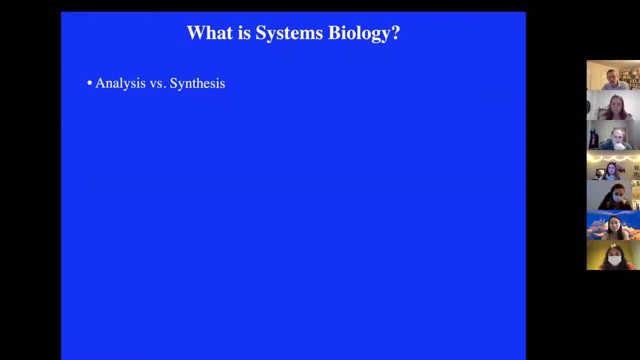 future. One is you can do analysis and the other is you can do synthesis. So let me explain The reductionist approach, which has been incredibly powerful. still very valuable and very important is: let's take pieces apart and see what they're composed of, and perhaps 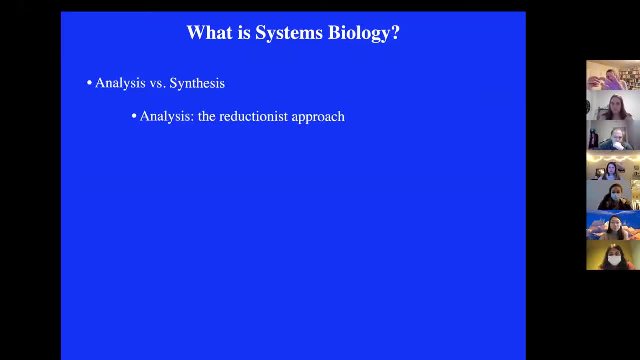 figure out all the different components and work down to the lowest possible levels. So first, as you start looking at biological organisms, you notice that they're made of organs. There's a heart, there's a kidney, there are lungs, there are liver and there are organs. 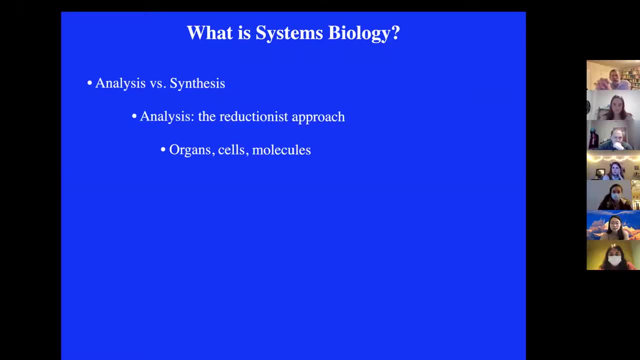 Understanding their functions is very important. They're made up of cells And, again, if you go up to your close friend and says, hey, you're made up of trillions of cells, I'm not sure how excited they'll be that you're regarding them in that particular light. but it's true And understanding. 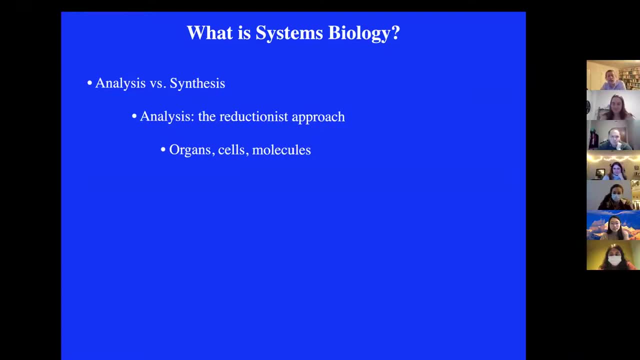 the cell is already an amazing thing, And recognizing that we are made of cells is a very important advance. But then really, the big revolution that occurred in the middle of the previous century was starting to focus on the molecules And molecular biology, which is a 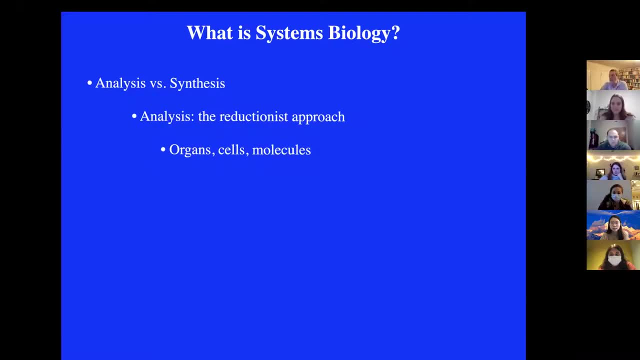 technology has been an incredibly powerful way of understanding what's going on. But the difficulty is- and anyone who has done this kind of thing knows- if you take a complicated machine apart, at the end of the day, what you have is a lot of pieces on the floor. When I was nine or 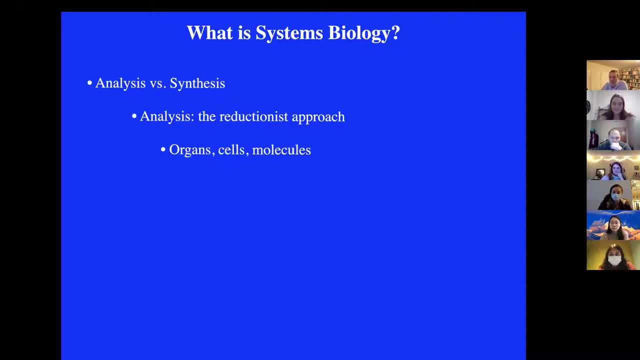 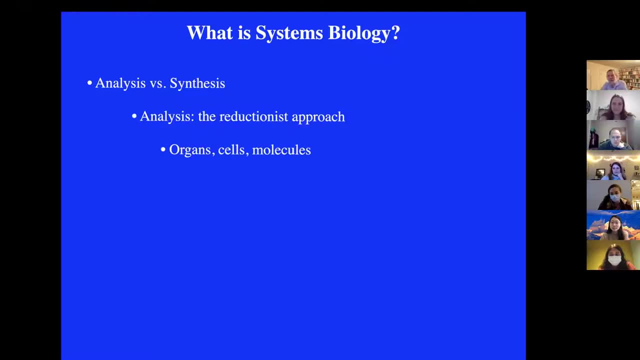 pieces of gears and I had all these pieces of gears And my dad was always okay about my taking things apart. My mom was not so enthusiastic So, with some concern that she might be upset that I had now the clock wasn't working so I felt it was all right to take it apart. I thought she 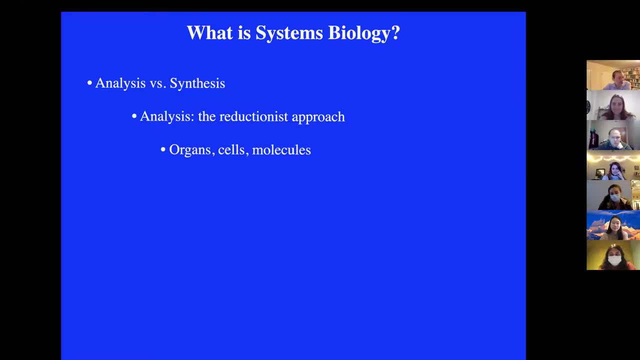 would be less likely to get upset at me, But I really felt it was really important to maybe restore it to its previous state. So I spent quite a bit of time struggling to get the mainspring back in and then put the gears back in and it actually worked. So that was a sort of a primitive example. 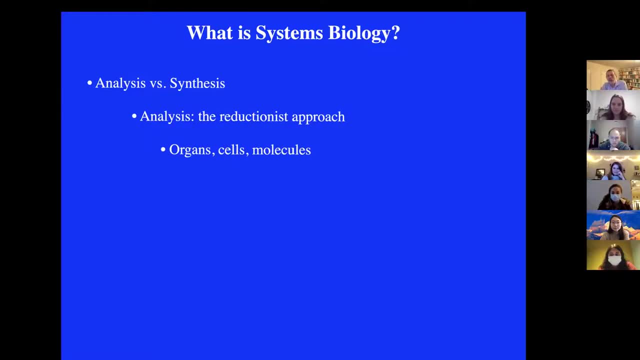 of analysis, taking it apart to pieces, and then synthesis, And again the reductionist approach has been incredibly powerful. But what's happened is people have recognized that at the systems level, even if you have a description, a listing, say, of all the cells and all the molecules, 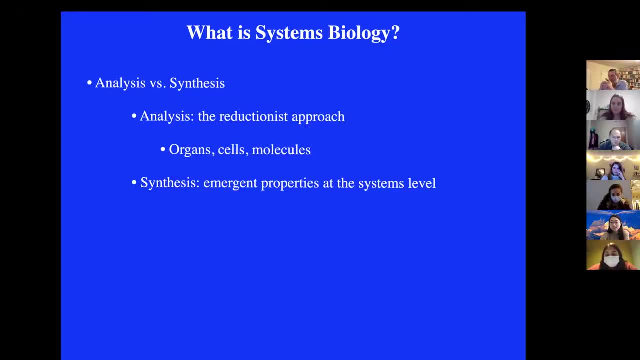 there are properties that make the functioning system very interesting that aren't captured by that listing of those components, And the question then is: how do you understand how the whole systems work? And that's where systems biology becomes very important. And just a few examples: 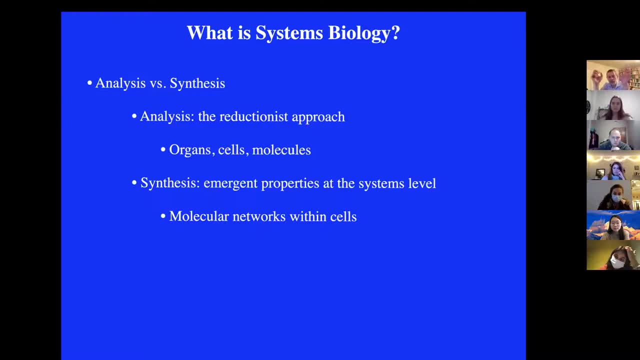 It's one thing to have worked out all of the key enzymes that are part of the Krebs cycle And very, very important to understand which cofactor is important and which enzyme and whether there is end product inhibition and all those other things, But what actually? 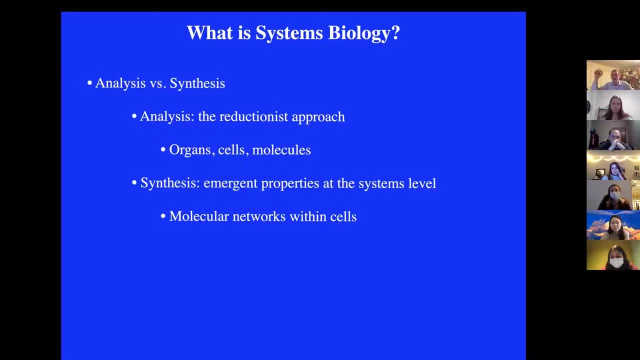 matters about the Krebs cycle, which is in the center of intermediary metabolism, is how the cycle actually works under certain conditions: When you've just eaten, when you're starving, when you're pregnant- all of these things they change, And they change in a dynamic fashion. 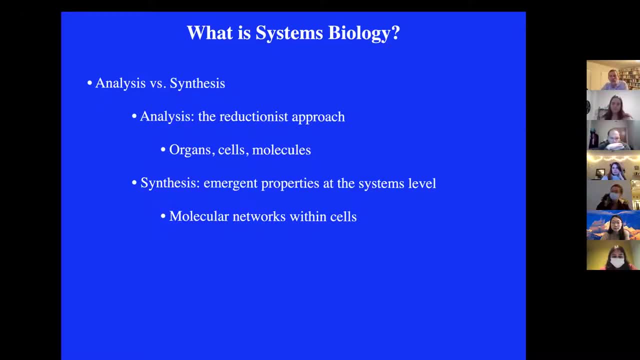 So understanding molecular networks is not going to come just from knowing the names and the properties of the individual molecules. Similarly, there are cellular networks. The immune system, of course, is a very important one, which has coordinated responses to foreign invaders, And of course, the nervous system is another example of a cellular network. 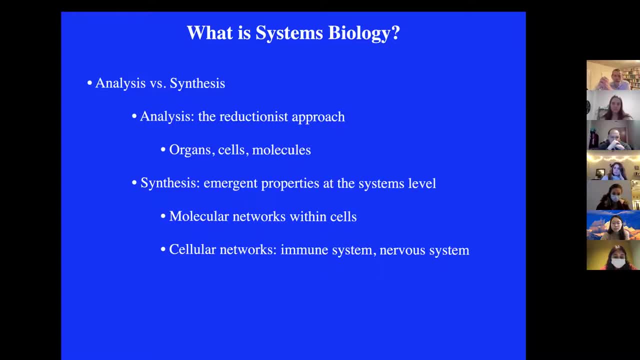 work. How do these work? Again, knowing all the molecules and even understanding the biophysics of individual ion channels doesn't tell you about the dynamics of the entire system. That somehow doesn't it's escaped your focus if you just break it down to pieces. Of course we talked about 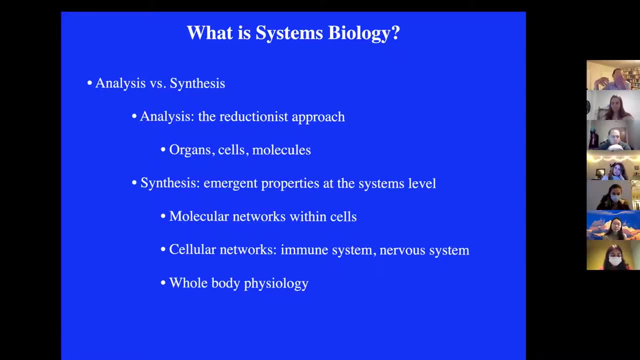 organs, but for example, how the heart and the lungs are properly regulated so that you can go from running to walking, to lying down and sleeping, and it adjusts to all the different needs seamlessly in general. How does that work? That again is a systems level kind of question. 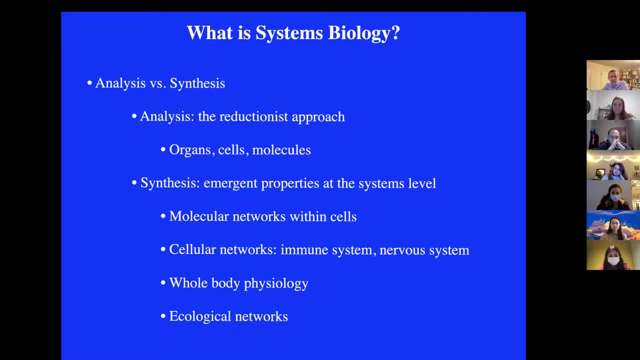 And then, of course, as you go beyond the single organism, you get to ecological networks, and you begin to realize that you're talking about these multiple, interacting, complex systems. So systems biology, then, is actually addressing the same questions that the reductionist approach did, but instead of taking things apart. 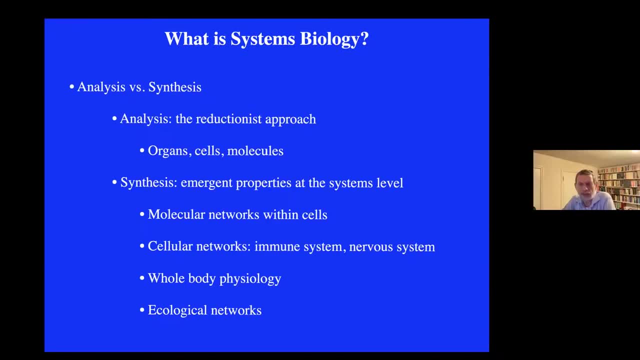 the goal is to put them back together and see how they work together. Okay, so that's the analysis versus synthesis point. Okay, now a second thing, and again here is where I'm going to warn you in advance. I have a strong prejudice, but I'm going to try to. 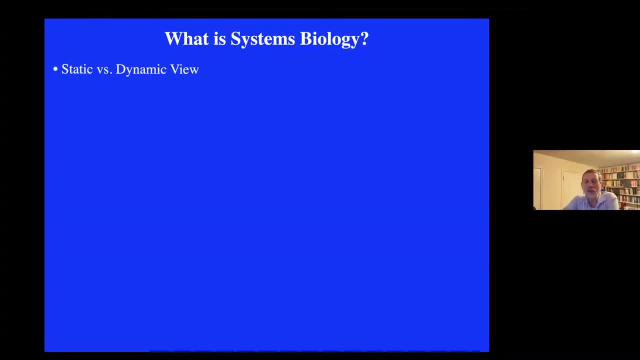 be as fair as I can. I think that the two ways in which people are talking about systems biology come down to taking static versus dynamic views. I'm very, very focused on the dynamic view, so my description of the static view may be unfair. I'm just saying that at the advance. 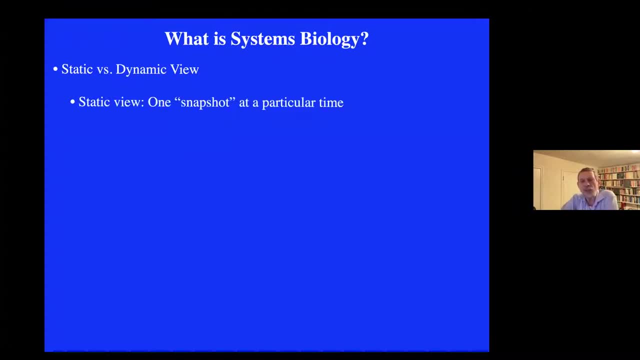 But the idea is that the two ways in which people are talking about systems biology come down to taking static views. The idea with a static view is you're trying to get a snapshot of the system at a particular time And that snapshot gives you a lot of information. What would be examples of? 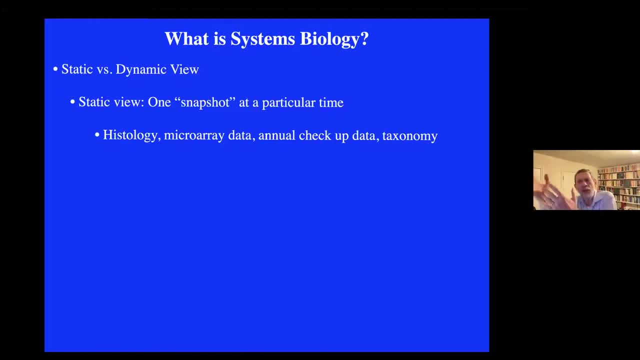 that. Well, let's say you have a histological slide of a piece of tissue. You now actually see not just individual cells, you see how the whole system is laid out, And various kinds of modern imaging techniques working on fixed tissue have taken histology to a whole new level. You can actually get fluorescence for individual molecules and you can actually get realunking and произ soybeans in individual molecules And you can see the example of tissue number. You know, sometimes tissue numbers then get backwards again And there are different順. 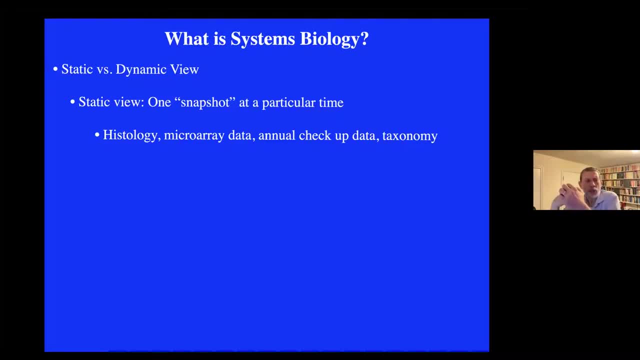 distributions of vostal cell levels. and this is because tissue matters here often And we may have to use evaluative medicine here now, but we need the data. So we are trying to look at just vitally seeming and and you can see expressions that are changing and so forth. but you have to see it at one point in. 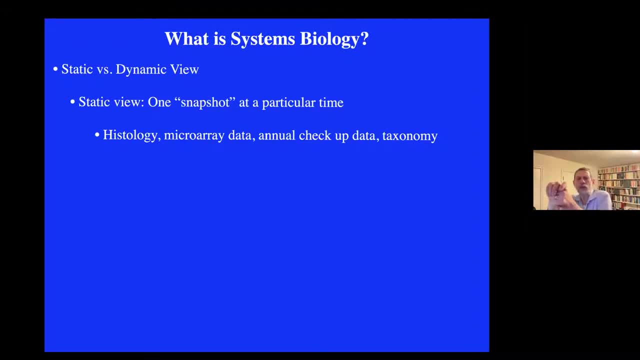 time. Similarly, if you get microarray data, that gives you very important information about levels of different key molecules in the cell, but it's a snapshot at one time. Another example that we may all experience is that when the doctor takes you in for your annual 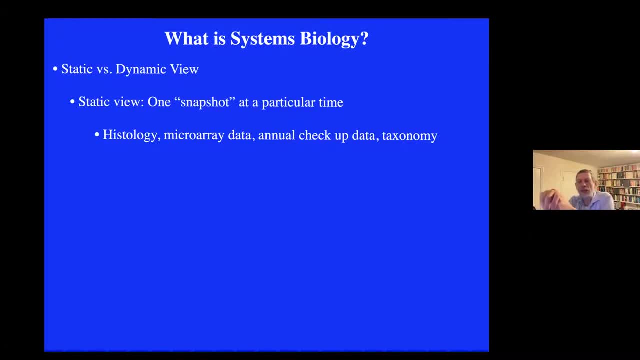 checkup and gets your blood pressure and your weight and your height and all those other things. the truth is, those things fluctuate from moment to moment, from day to day, from month to month, but that gives you a snapshot of how you're doing and that's useful. And then, finally, 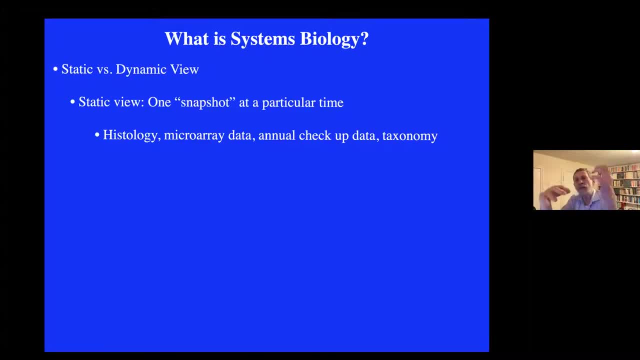 when people talk about taxonomic relationships. again, that's a very important evolutionary view of how different things may have evolved, but generally they're represented as trees or bushes and the things are relatively static. Now, of course, as new information comes in, they may 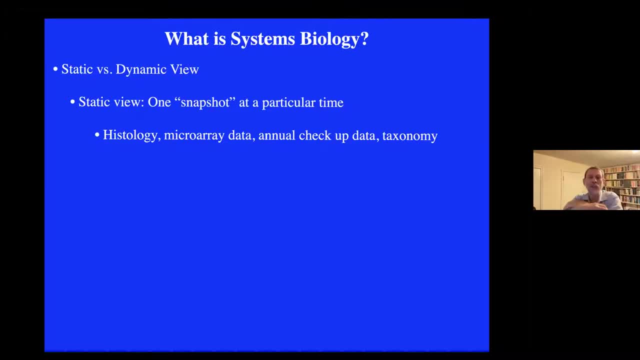 get adjusted, but the whole idea is that you're trying to come up with, in a certain sense, a relationship that is fixed Now. a similar example, I think, are studies of the genome, proteome and connectome, So let me briefly define each one of them. So, genome, the Human Genome. 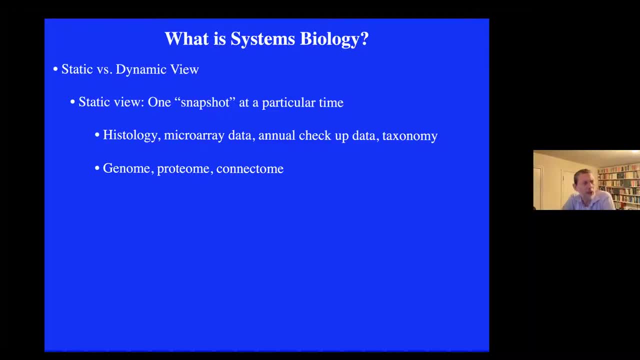 Project, for example, was to find a particular human being and find every single nucleotide in the sequence of DNA in that person's entire set of genes. So it's a whole bunch of ACTG letters over and over again and that constituted the genome. Now the point is that when you get that 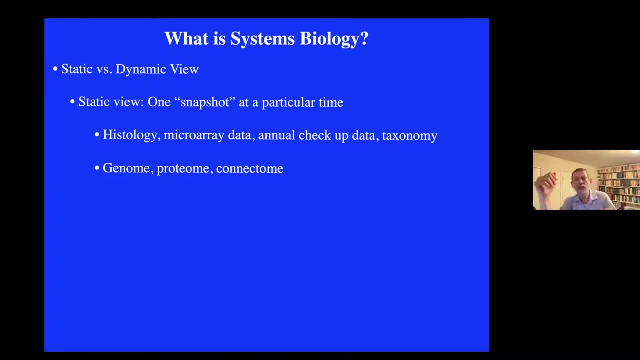 you have a genome, but it's not dynamic, it's not changing in time, it's the genome. Now you can use that as a reference to talk about how other genomes vary or are different from it, and that's very important, and you can then start to do classification. But the genome itself just 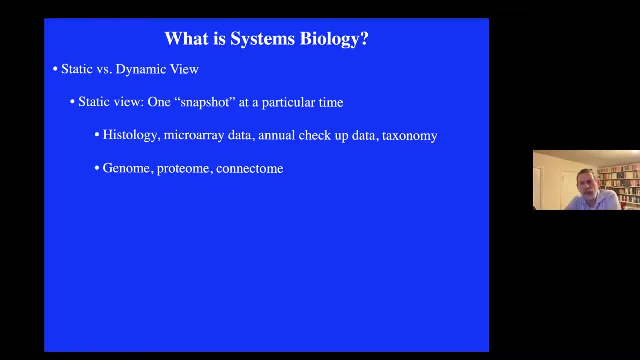 sits there. it's just a listing of those letters. Proteome is similar. it's all the proteins that might be expressed at a particular time, So you can use that as a reference to talk about how, in a particular setting, in a cell or in an organ, And the connectome, which is something 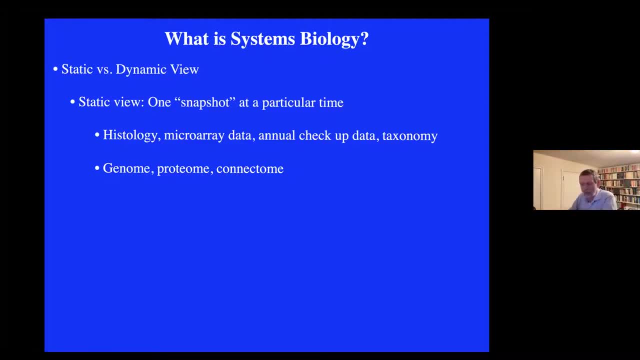 that's very people who are studying the nervous system are very excited about is by using things like electron microscopy and other techniques to reconstruct every single possible connection between neurons in a neural network. The problem, of course, again, is it's a static picture. 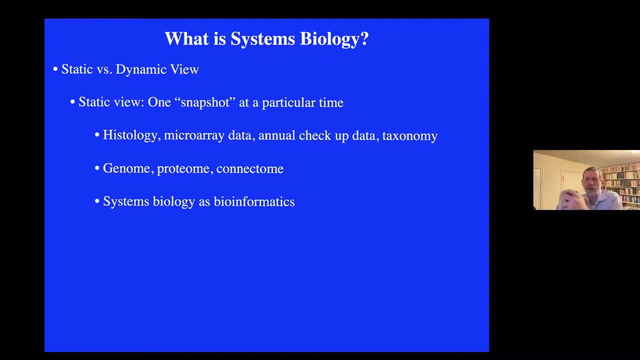 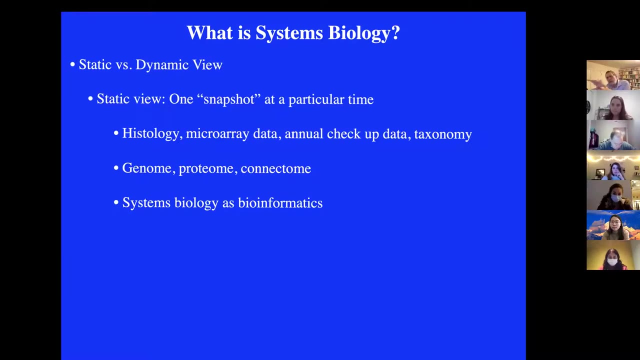 And the way I would summarize this is: if you're looking for a gene, you're looking for a gene, you're looking for a gene and you do a blast search and you can find that there's enough similarity that it might be similar to this other. 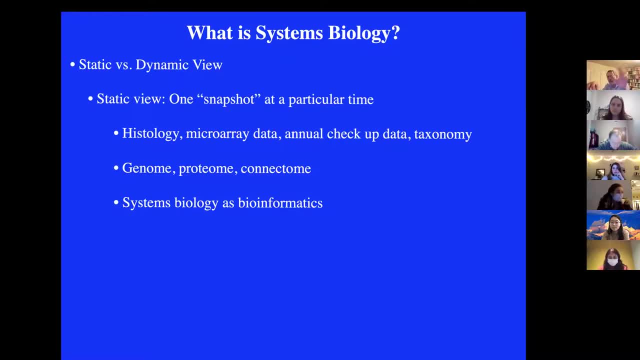 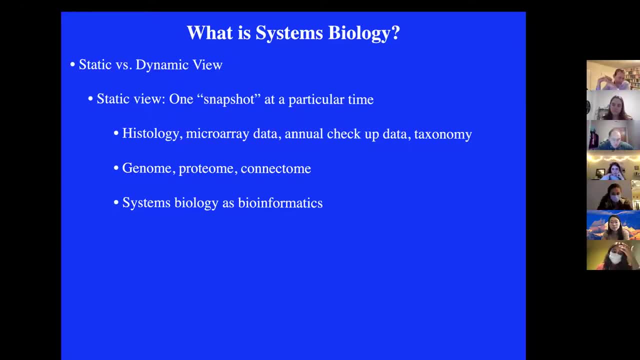 often with static snapshots. That's my way of thinking about it. It doesn't mean that it can't be dynamic, but that's not what the focus usually is. Now, in contrast- and this is, of course, where I get more excited- there's a dynamic view, which is that biology and many other things- 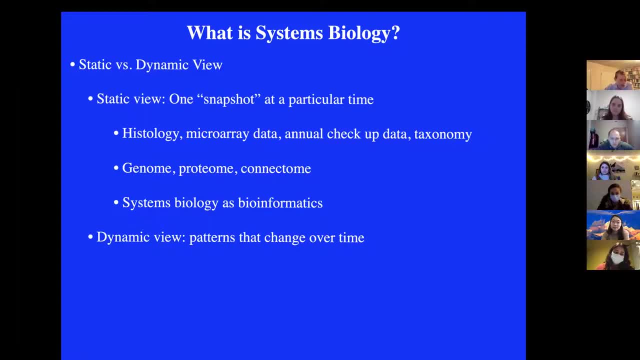 but especially biological organisms and groups, are about patterns that change over time. So it could be patterns of movement, It could be patterns of gene expression, It could be patterns of activity in the nervous system, It could be patterns of activity of populations rising and 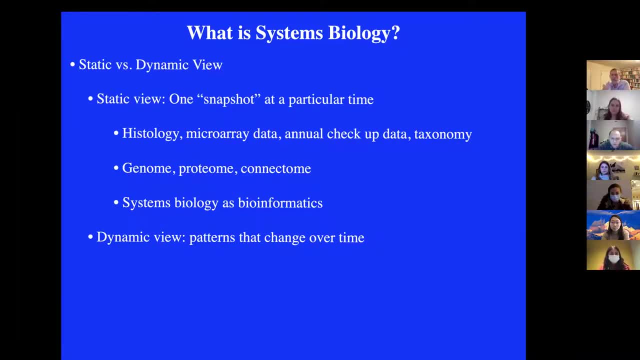 falling. But these are dynamic patterns that change over time, and that was why I put this in my title, because that's how I think about systems biology. Now, in order to get a handle on that, that requires that you develop mathematical and computational models There. 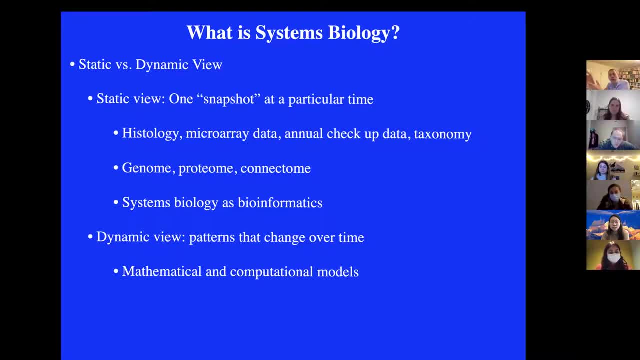 simply listing what's there doesn't tell you how A goes to B. You have to have rules for transformation. That could be differential equations, It could be agent-based models, Whole variety of different possibilities. But the critical thing is that you are looking at. 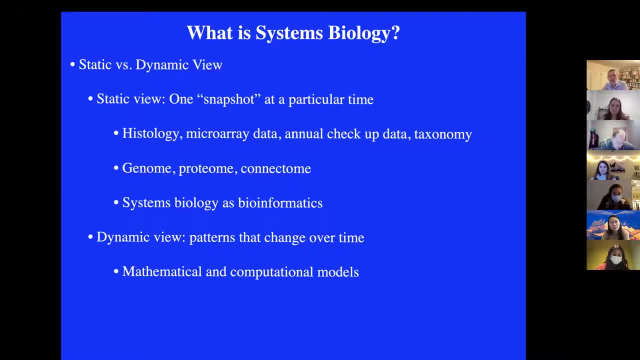 something that changes with time. You're trying to understand these dynamic patterns. That's the focus And, in general, when you do things like that, your focus is going to be more on what I think of as normal physiology rather than pathology. Now, pathology is very important. 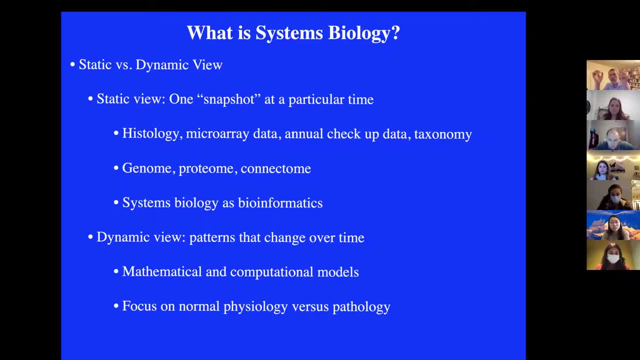 Of course we want to get to translational and medical applications, But understanding the delicate interactions of the different components under ordinary circumstances, I believe, is fundamental to actually get to pathology, And pathology is often a case where the system is being run up against the rails. 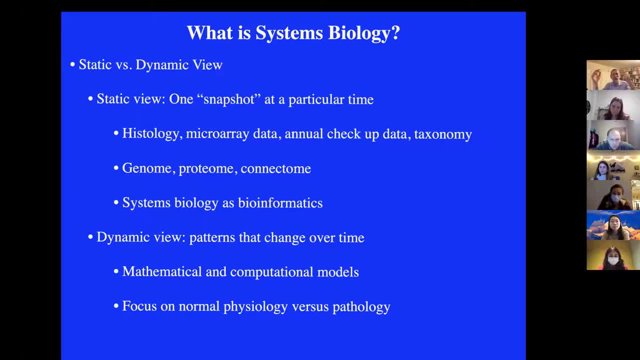 It's in saturation or it's down at zero and the rest of it is trying desperately to compensate for those problems. So you don't learn a lot about what the normal physiology is when you focus so much on pathology. So again, if you're actually looking for dynamic patterns, 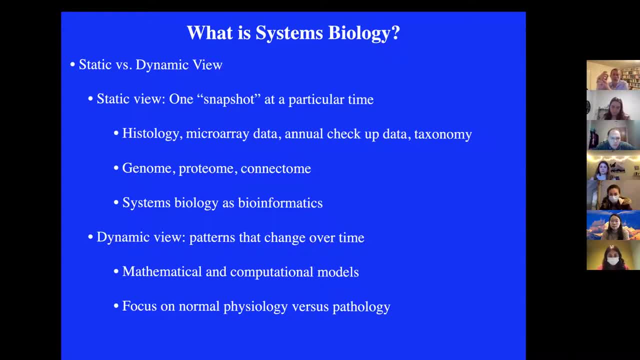 I think it's better to look in the situation when you're looking at normal physiology and learn from that- what to do with pathology, rather than start with pathology. People who are medically oriented will disagree with me. I know that because I've disagreed with. 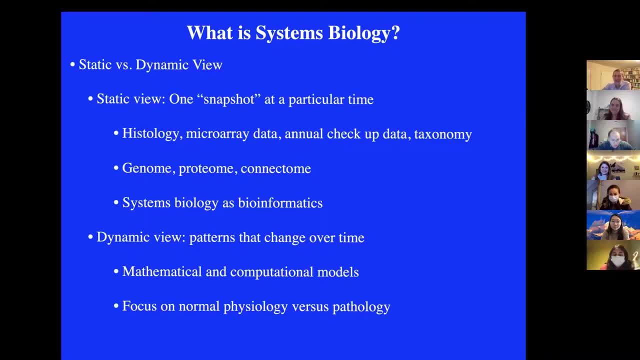 them in the past and will, I'm sure, in the future. But I think this is an important viewpoint to express and articulate, especially to impressionable young minds who are going out there and maybe encountering that other viewpoint repeatedly. So that creates the notion of systems. 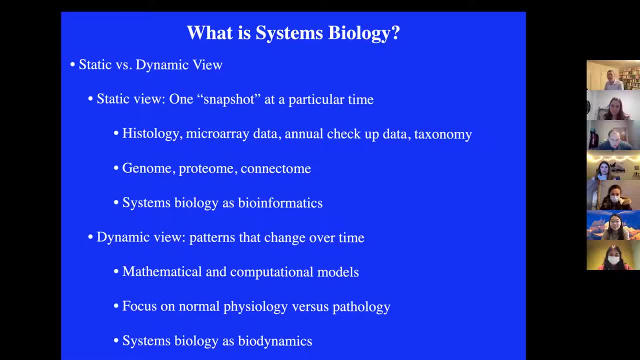 biology as what I would call biodynamics. You're really interested in how things change over time. So that's all I had to say about what is systems biology. Are there any questions that people have at this point? Okay, that's fine. I often have the brilliant question just after the person has disappeared. 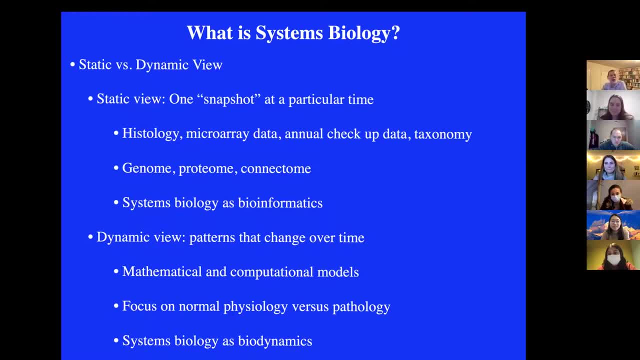 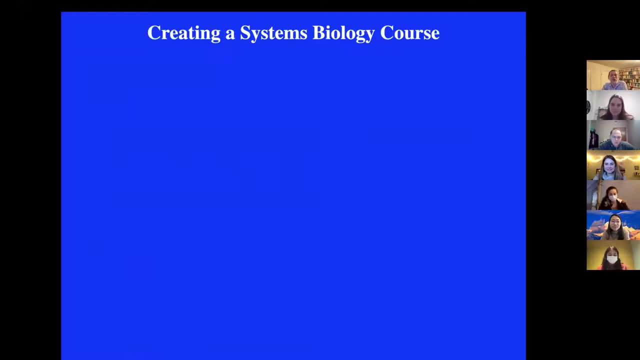 off my screen and I can no longer talk to them. But you can always send me an email and I will respond- Maybe not instantly, but sooner or later, And I will always be interested in what you have to say. Okay, so let me give you a little bit of background of what gave rise to BIO 300,. 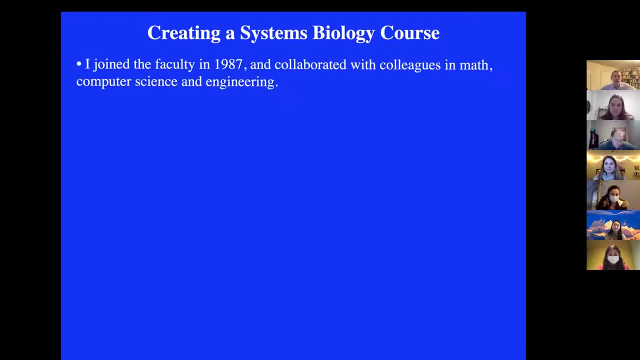 Dynamics of Biological Systems and the Systems Biology major. So I joined the faculty in 1987, and I regularly collaborated with colleagues in mathematics, computer science and engineering, And one of the things that was critical for doing an effective collaboration was to share students. 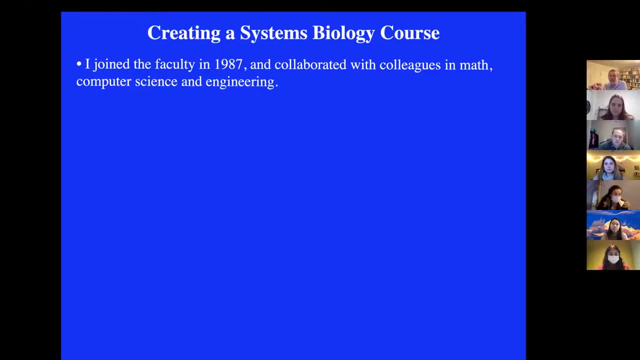 And the difficulty was the math students knew math and the biology students knew biology, But there weren't students who had in the same head both knowledge of mathematics and biology. How do you get such students? Well, you can teach them that material and then those students become 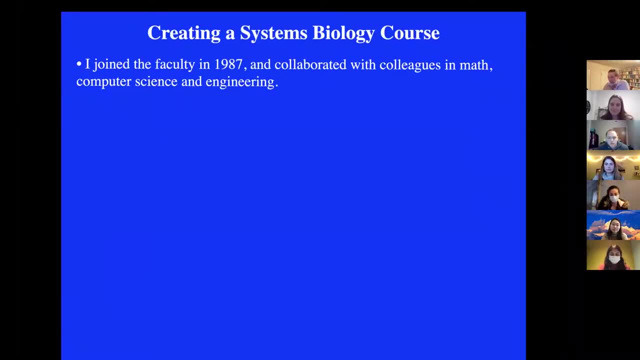 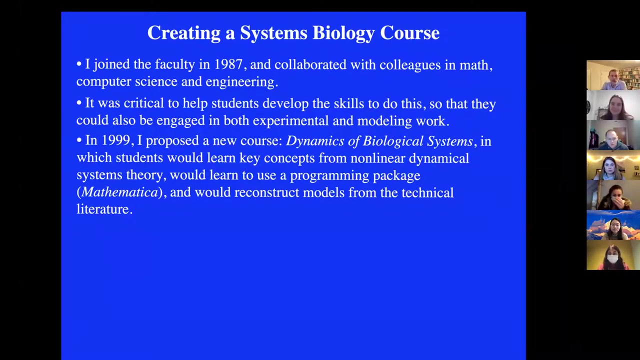 part of the group that can be focused on these questions, not necessarily just for me but for anybody else. So, because I felt it was critical to help students develop the skills so they could be doing experimental and modeling work, in 1999, I proposed a new course, Dynamics of Biological Systems, and in that course students 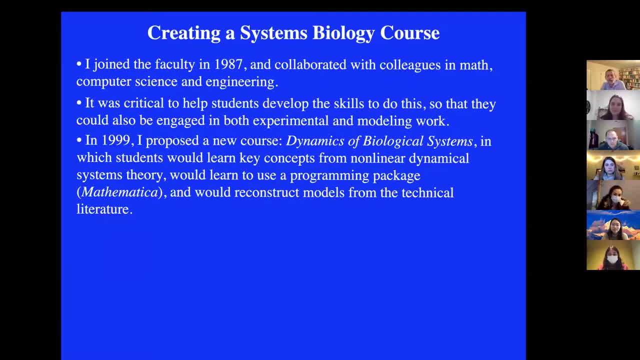 would learn key concepts from non-linear dynamical systems theory and would learn to use a programming package, Mathematica, and would reconstruct models from the technical literature. so that's how that course came to be, and those of you who've gone through it now realize that that was not something. 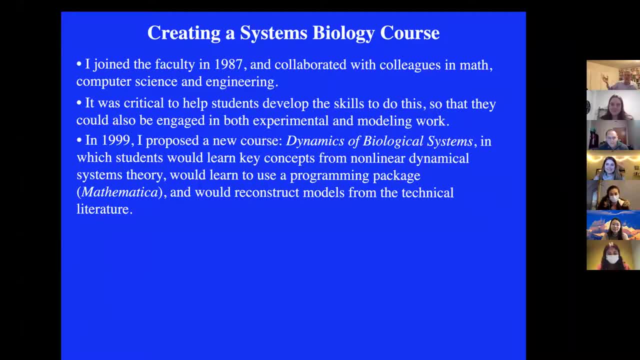 that was, magically, you know, present from the time that people I actually said we need a course like this, I was able to convince my chairman at the time, Norm Rushforth, that we should do it. he was willing to let me try. it took me about a year of preparation to get started. initially, I 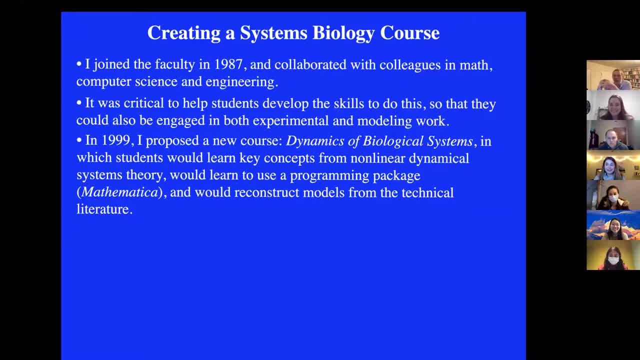 had two students- those of you taking it with you know 36 or 25 or whatever. it started very small and I taught it every semester for the first two or three semesters to try to get people out there and interested in it. and it kept on growing and growing and growing until it got to the size that 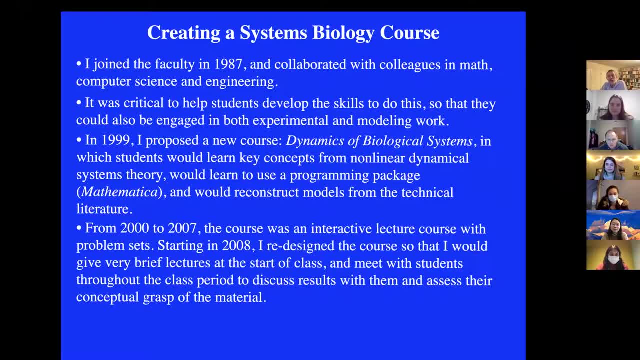 you're more familiar with, and then from 2000 to 2007,, the course was an interactive lecture course with problem sets. so what I would do is I would take a course. I would take a course and I would do is I'd have everyone sitting in front of the computer with Mathematica open. I'd be projecting. 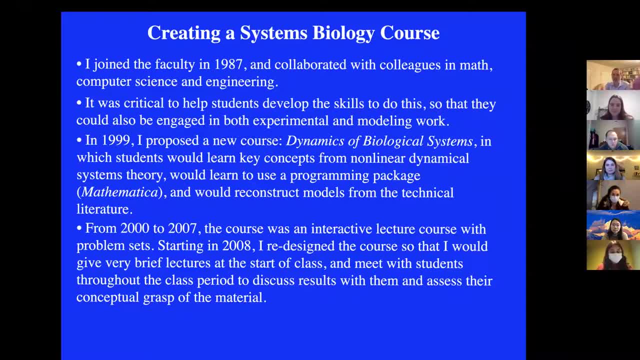 my computer on the screen and I would type things and have them type and then it was like blindfold chess, because the students would raise their hand when something didn't work and I'd run around and say, oh, you forgot a bracket, you missed this parentheses. oh, that needs a curly brace. 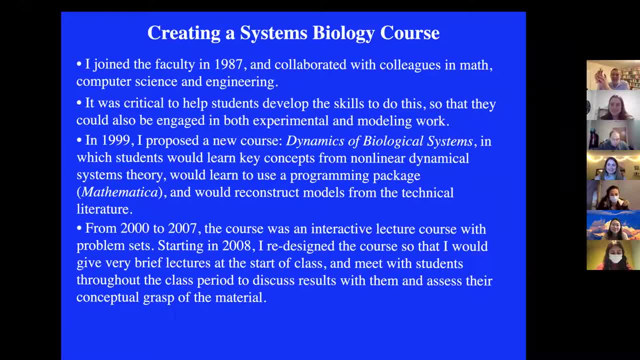 lots of fun anyhow. and then there were problem sets that we're doing. the students would go crazy trying to get the problem sets done and they made some progress. I had them reconstruct the models, but I found it was really frustrating. 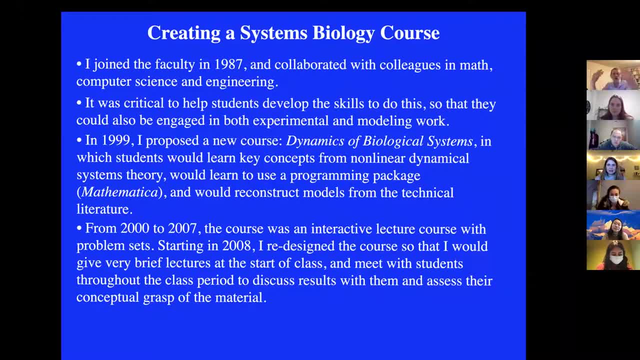 They didn't seem to really be able to do very much, even though I'd spent all this time and I'd show them how to do it and I'd have them suggest to me what I should type next, and all this sort of stuff. so in 2008, I made a decision, with the help of a very talented 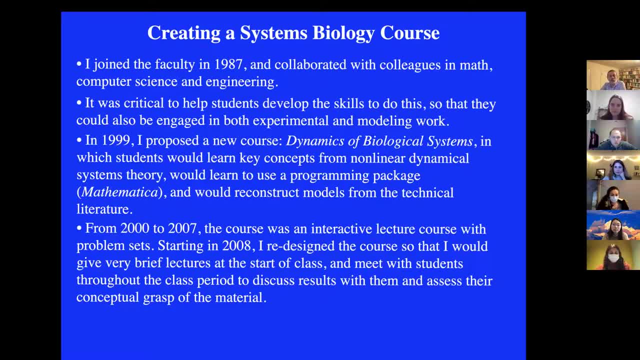 graduate student, Kendrick Shaw, to totally redesign the course, where I would just talk very briefly at the beginning of class- five minutes, maybe 10 minutes if I was, you know, had lots to say- And then the rest of it I would just meet with students throughout the class period to discuss. 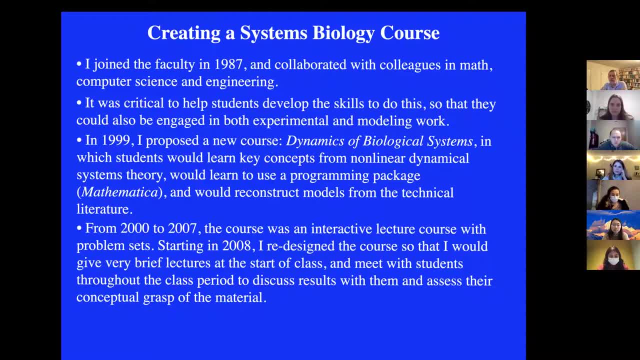 results with them and assess their conceptual grasp of the material. so I'd sit down, I'd look at what they did, I would make a few comments, then I'd do that very quickly just to get a sense of where they were in terms of problems, and then I'd come back and then we would talk. 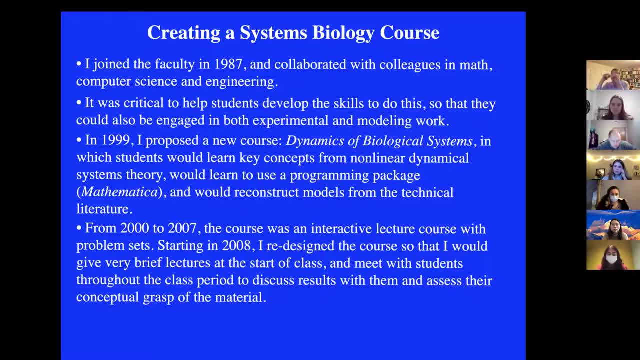 in more detail and what I found was this had a radical, radical effect on the students' ability to do the material in the second half of the class, because they were the ones who were in charge and they were making the stuff work and I was just giving them some suggestions. 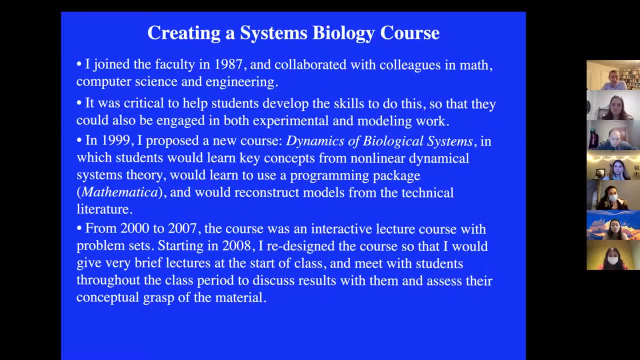 but they were making it happen By the second half. when they had to use ND, Solve or other tools to visualize and to implement the models, like Manipulate, they knew how to do it. and so the second half of the semester, instead of being this sort of huge ramp up, it was a much more gradual slope. 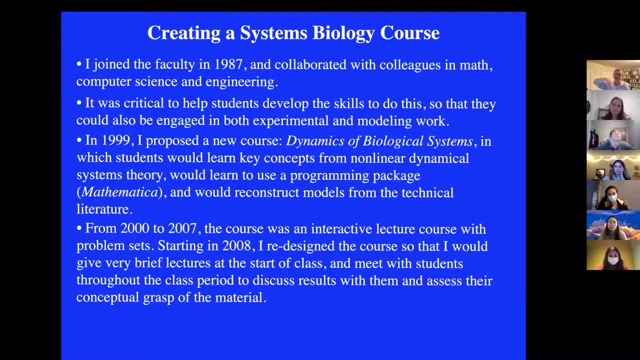 The first part of the course was very hard for the students because mastering Mathematica and understanding concepts, The nonlinear dynamical systems theory, is not trivial, but I tried to get the on-ramp as gently as I could. and then the second half, which is going up to really expert level. 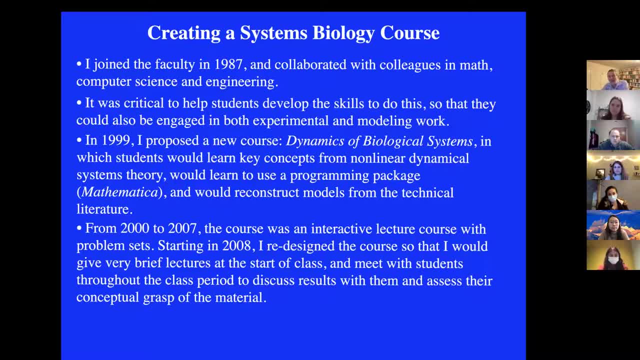 in one semester, because building a model from scratch is really hard and even reproducing a model is hard. the students had a much easier time, so that was a very effective change. It's just very labor-intensive and one of the ways I dealt with that was I was able. 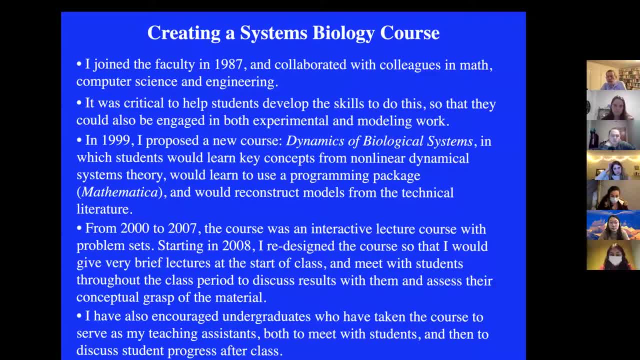 to encourage undergraduates who take the course to serve as my teaching assistants. and so now in the classroom, basically during the class session, I'm meeting with the students. the fellow instructors are meeting with students. that's all we're doing. 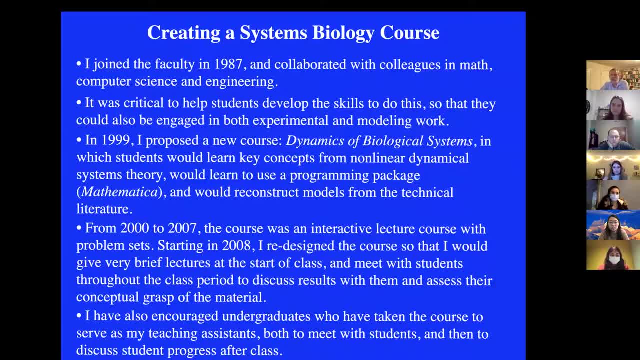 So again, I give a brief lecture at the beginning and the rest of it is I'm just talking to the students And then the students generally when I'm not talking with them. if they are wise students- some of them are- are spending time on the next problems and talking to their teammate. 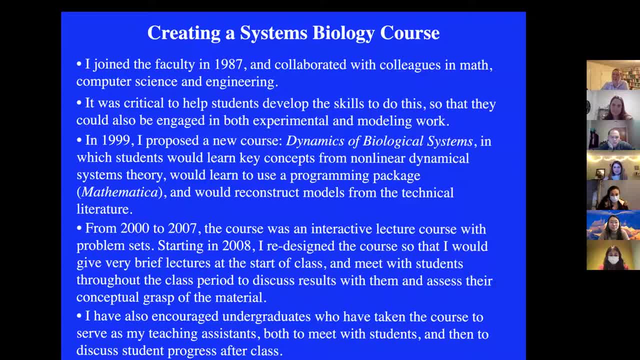 and working hard and they're not on Facebook and or checking their email and or whatever, or seeing what the latest sports results are, latest news. they're actually working and on task And generally that's worked very, very well. So that's the course I developed and in fact, I took the same design after getting into 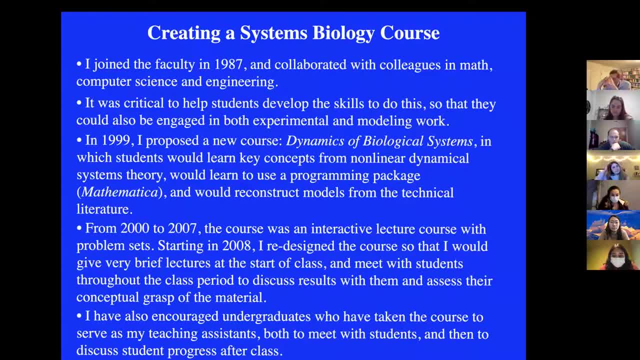 work in this course where it was more natural, and I shifted what had been a lecture course introduction to neurobiology to work more or less the same way, using simulations of neural components. So those people have been subjected to introduction to neurobiology. 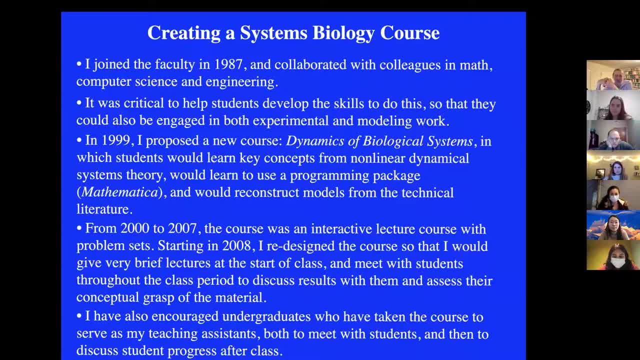 They've been subjected to introduction to neurobiology. They can blame Bile 300 for why I teach the course the way I do And the students don't necessarily love it while they're going through it. but in retrospect- and this is unsolicited testimonials- I don't go out seeking this. I get emails regularly. 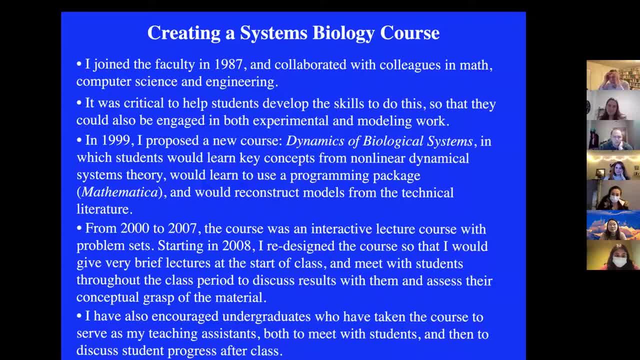 over the years from students who said: you know that course was incredibly helpful and now I can do things I never thought I was able to do and I really learned much more than I would have if I'd had a standard, had a percent necessity. 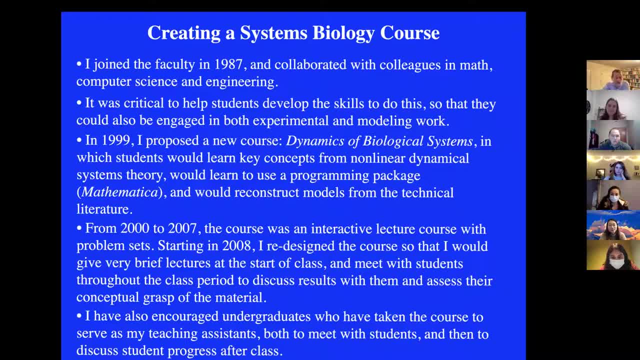 Yeah, So that's given me the reinforcement. I mean, some students don't like it And there's some students it doesn't matter what I do. There's some students who are so good that I could just show up in class say hi, here's. 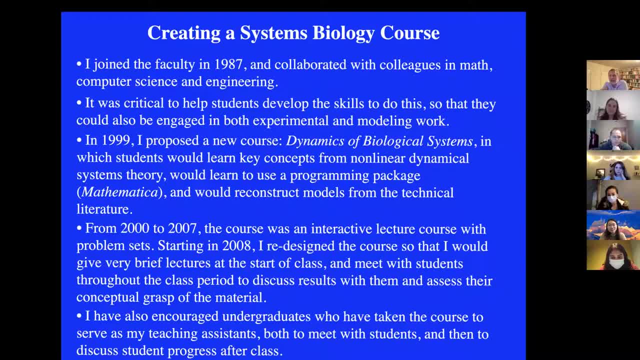 the textbook. here's some problems. Good luck. And at the end of the semester I could look over their shoulders and say, yeah, you got an A, But that's a very rare kind of student. For the majority of students, this has really been very helpful to them. 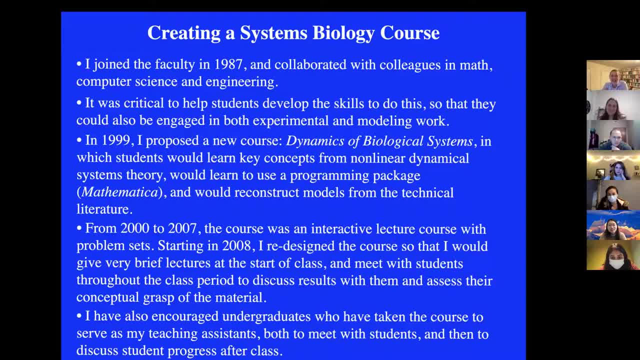 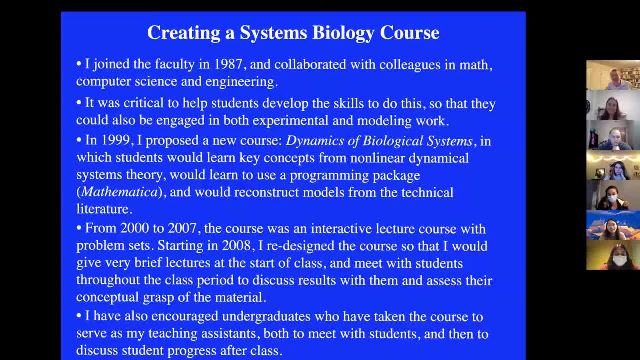 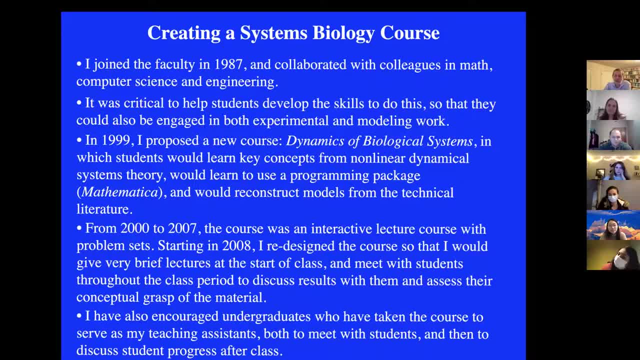 And so they were very helpful to. this is again common sense to me. Well, did you have any issues that took place at all, specifically with the解 folic illegal access? But it's again, very rare to see this study. 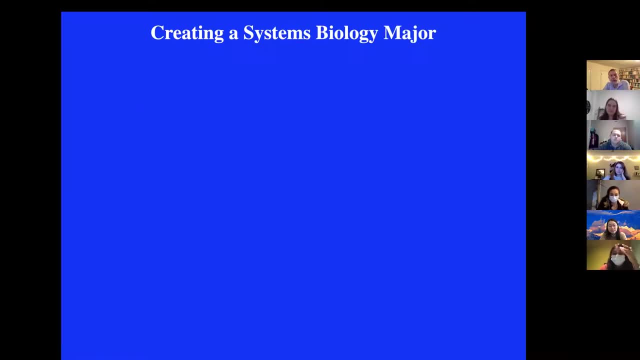 We've seen pretty many cases of a colorectal scareside in this study. aus em: ja, Yeah, That was very good. I didn't know what thoughts I was making. You talked about again this is prefabricated and the augmentation of instances, from defining a trauma for a problem. 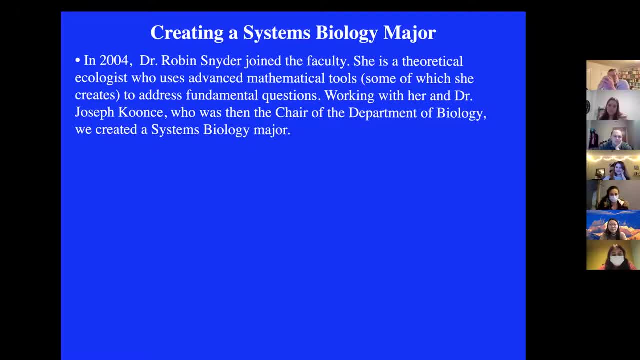 And that was that: mathematical tools, some of which she creates- her background is in physics- to address fundamental questions in ecology. So, working with her and Dr Joseph Kunz, who was then the chair of the Department of Biology, we created a systems biology major, And the major has not been huge. 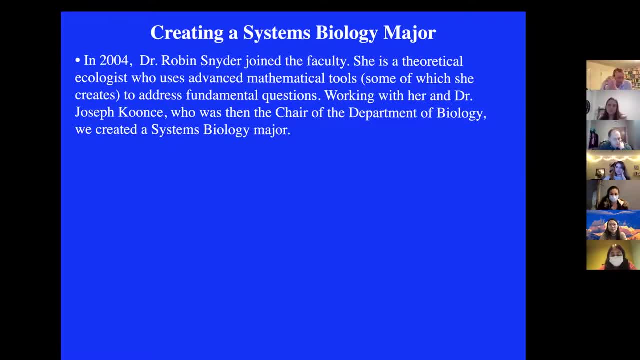 The number of people coming through is usually a fairly small number, but I like to think that, on the whole, the quality is very high, And that's what I've been very impressed with. We've managed to attract students who have a very wide range of backgrounds. 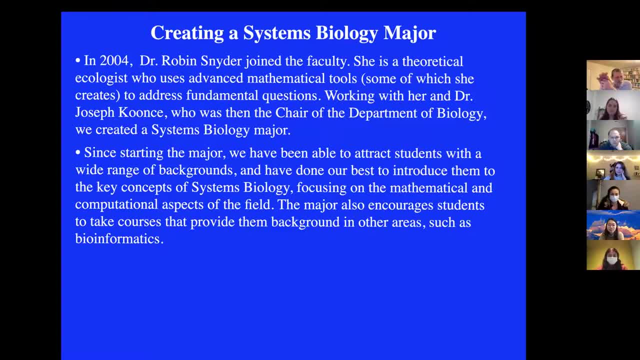 and often these are students who have more interest in math or physics or engineering, but they don't want to be a biomedical engineer and they don't want to be a computer scientist. They really want to be a biologist. but they've got these additional skill sets and 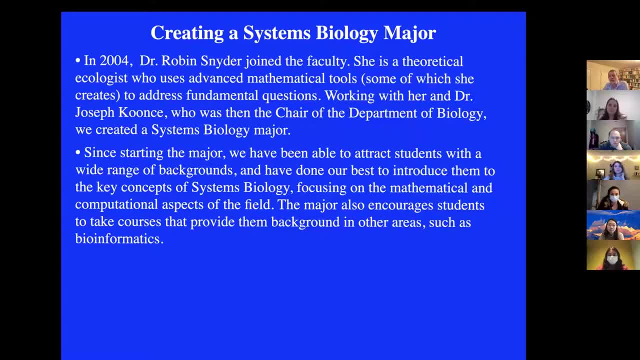 most biology courses don't address them. They don't use them at all. There's a lot of memorization, short answer questions and so forth, But having this major allows those students to really flourish and to reach their full potential, And so this allows us to teach the mathematical and computational aspects of systems biology. 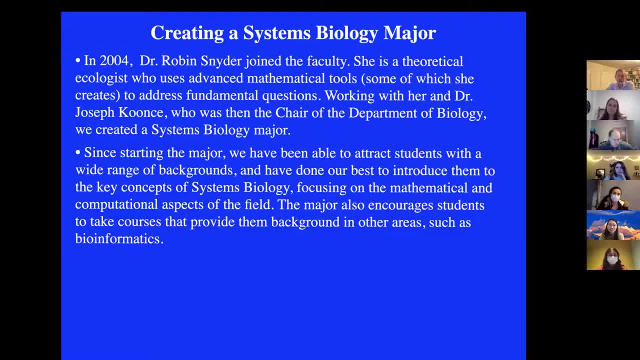 And part of the major, of course- also encourages students to take courses to give them background in areas such as bioinformatics, databases, computer science and so on. And I just at this point, and this, perhaps, is the only thing you'll take away from the entire hour- 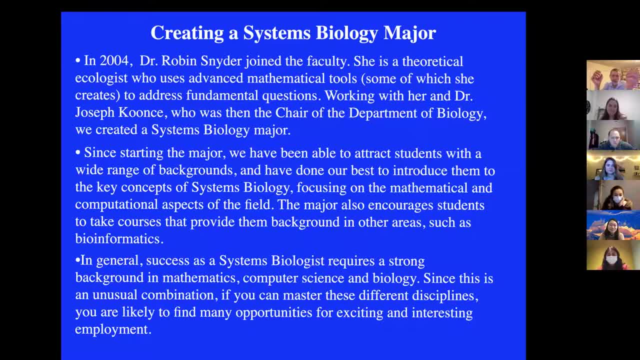 but I want to emphasize that if you want to be successful as a systems biologist, you need a strong background in math, computer science and biology. And it doesn't hurt to know physics and it doesn't hurt to know engineering as well, but those are fairly critical math. 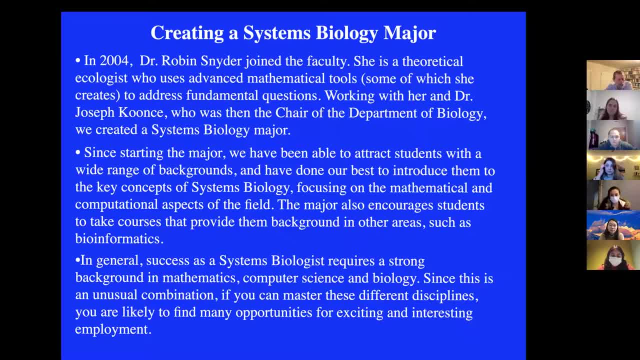 computer science and biology. Now I want to emphasize that, since most biology majors, if you start talking about mathematics or even computer programming, run screaming from the room and that's not much of an exaggeration- that if you really can combine all of these together and in your head, 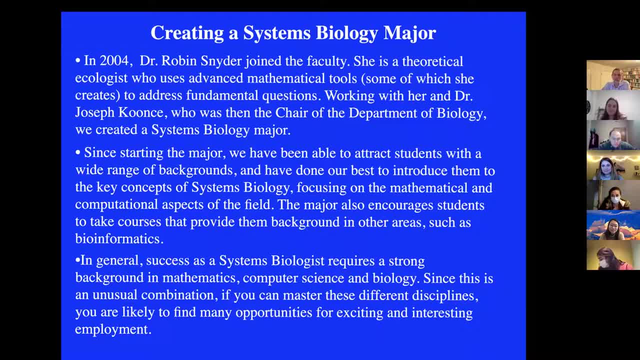 and know them, you will have an incredible advantage over many, many others for employment because you'll have that skill set. And similarly it is the case that most mathematicians and computer scientists- if you start giving them detailed biological information, they also run screaming from the room, And so, again, it's very unusual and difficult to get. 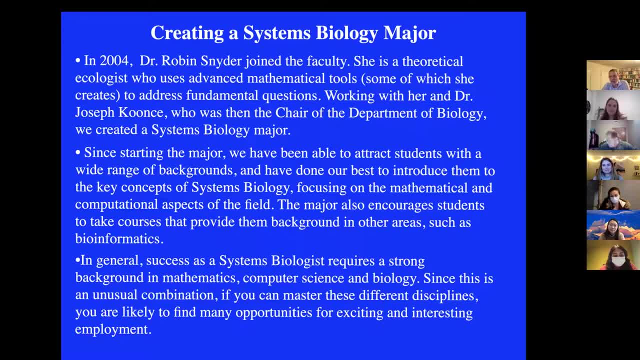 in the same head all of these different skills, And if you can succeed in that, it is incredibly powerful. So that's what I wanted to say: Thank you. That's why the major is there, and I hope that gives you some sense of the rationale. 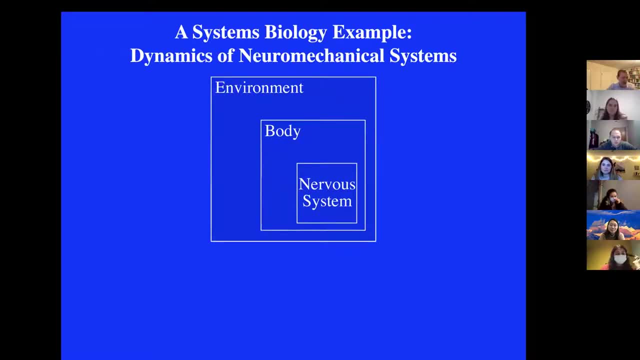 All right. So now, one of the things Smaranda asked me to do is ask: well, you seem to have this systems biology perspective. How does it affect your own research? So the next few minutes, if you choose to doze off because you're not interested, I will understand and then I'll come. 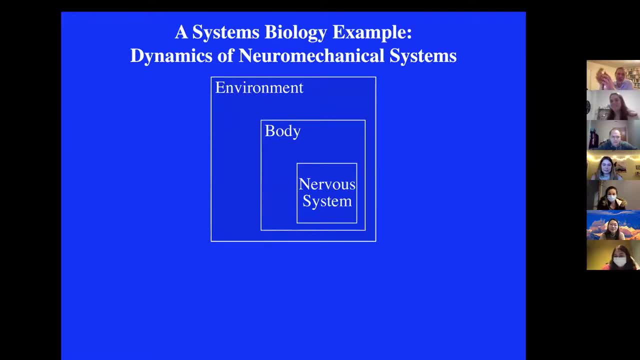 back to talk about more interesting things perhaps, But this is the stuff I do on a daily basis. This is what I wake up in the morning and I'm excited to spend time on, So I thought I'd share a little bit of that with you. 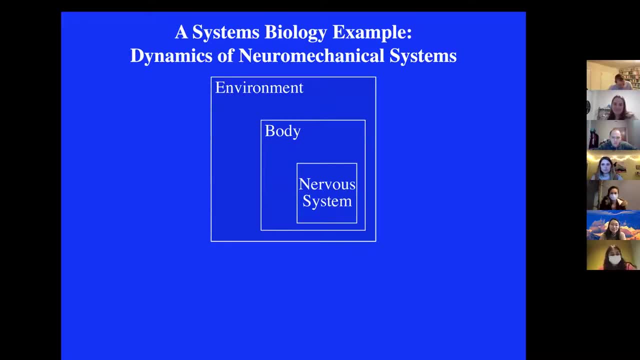 So what the broad question I asked is- and I'm very interested in- is adaptive behavior. This is behavior that allows us to survive and reproduce and therefore is pretty important from an evolutionary standpoint. Things like being able to walk around the world, find mates. 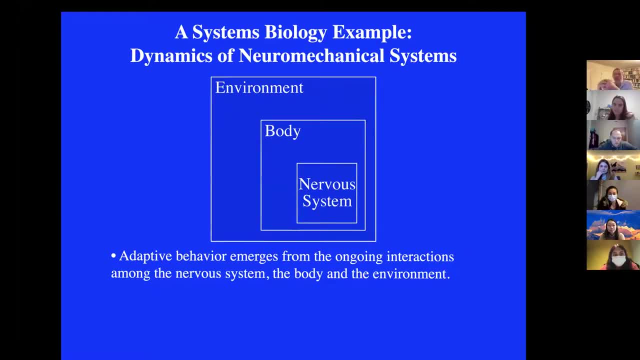 food, avoid predators. In college, finding food and finding potential mates is a very sort of a major activity and perhaps more important than class, And indeed the professors may be seen as the predators who we were trying to avoid. I don't. 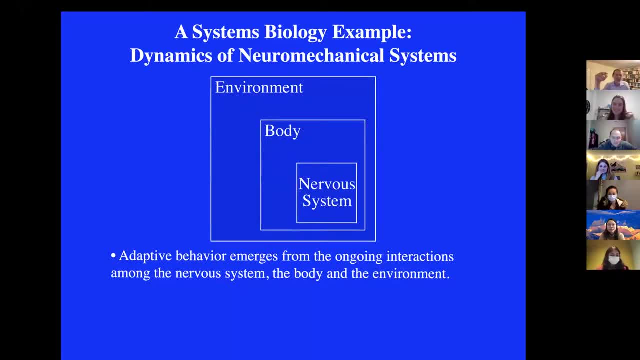 know, But in any case, the idea is that this is something that is very critical and this is what the evolution works on, Because if you fail to survive, of course you can't reproduce, And if you don't reproduce you don't leave anything in the population that will have impact later on. 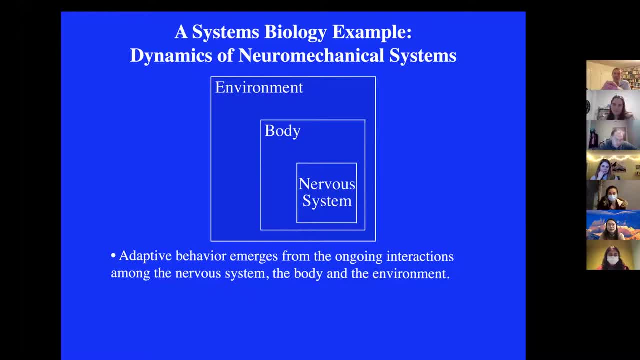 So you may have been very successful in your own life, but if you leave no offspring, from an evolutionary standpoint- I'm not saying in terms of your moral or ethical worth as a human being, But from an evolutionary standpoint- not leaving offspring means that you're. 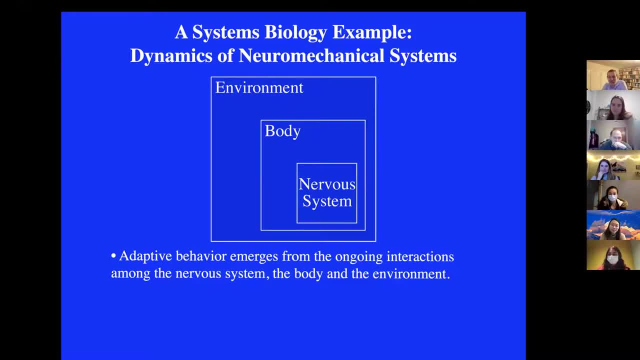 no longer representative of the gene pool. So this is really very important And that's what evolution selects for. It's this whole package And that system's viewpoint requires that you study the nervous system not in isolation, but embodied within the context of the body. 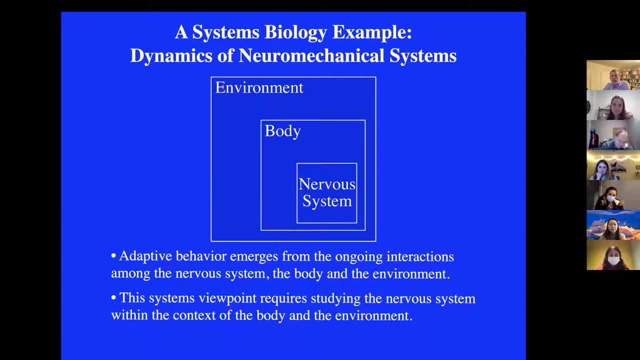 and then situated in a particular environment, And all three of these can be thought of as complex, nonlinear, dynamical systems in constant interaction with each other, And it's that whole interaction that is selected for by evolution. So this is a rather tall order. It's hard enough to try to imagine studying the nervous system. 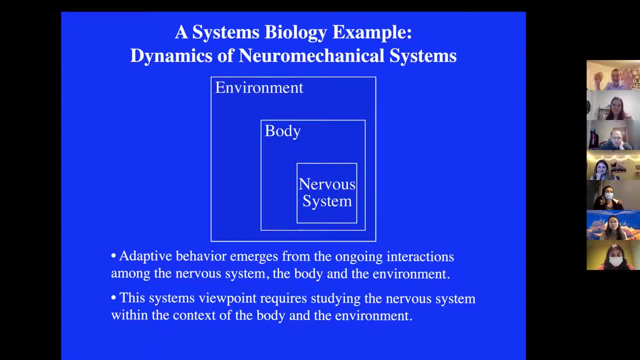 and now you want to talk about the body and you're also interested in the environment. That's really a lot, which is why not everybody is going to be engaged in doing it, But if you could somehow take a slice through this and get at it, it would be very, very interesting. 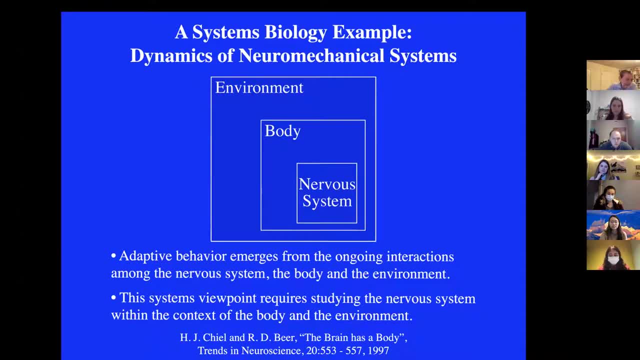 So, if you're interested, there's a review I wrote with a colleague, Randy Beer, who is now at the University of Illinois at Bloomington, But this is a very influential review that we wrote. The Brain Has a Body. It's easy to look up And it still actually after all these years. 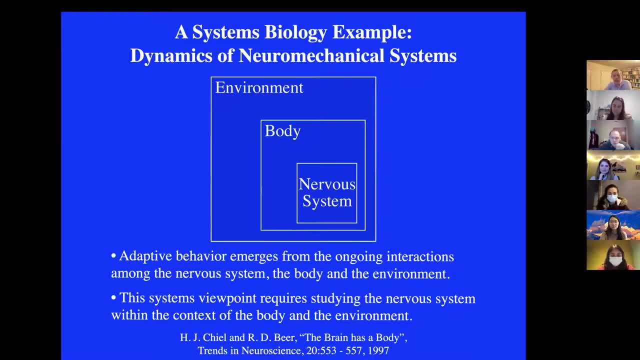 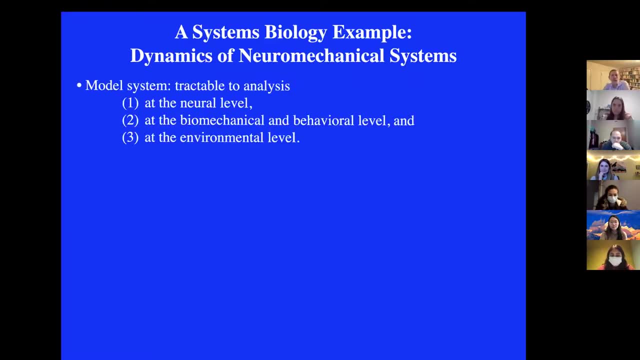 still has lots of relevant points that are worth knowing about, So let's see what that involves. What you want, then, is a model system which is tractable to analysis at the neural level, at the biomechanical and behavioral level and at the environmental level. So that means 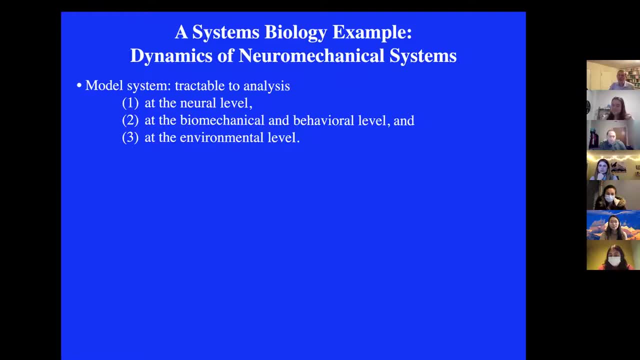 you're probably not going to be focused on humans. if you do that, In fact, even mice and rats are really complicated. Maybe you want to go down to the level of- I don't know, a roundworm like the nematode C elegans, It turns out. however, its nervous system is somewhat hard to. 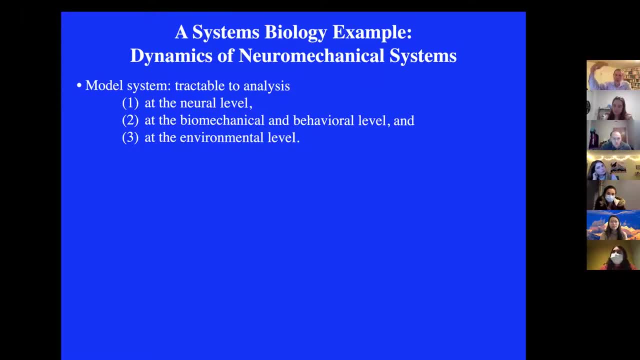 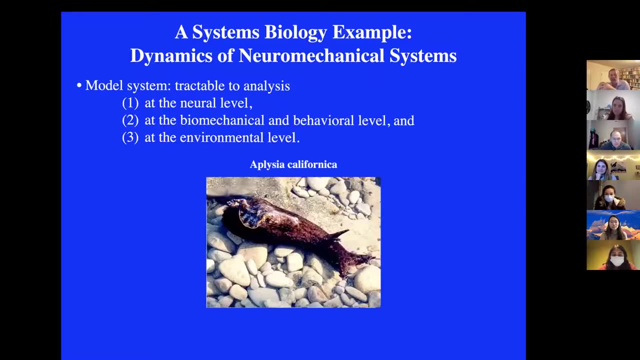 study. So maybe you stop a little bit earlier than that. You do something intermediate, not down to the level of a 600-cell worm, maybe something a little more complex, And that's the reason I've chosen to study this model system, which is the brain has a body. It's easy to look up, It's 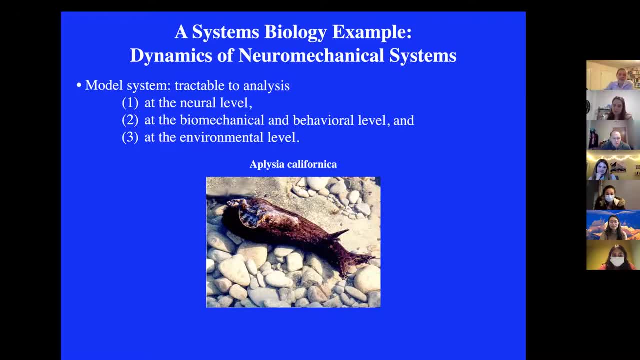 marine mollusk, Aplysia californica. And let's see, can you see my? I can't see my own cursor. All right, so the right hand shows the head of the animal and the left hand shows the tail of. 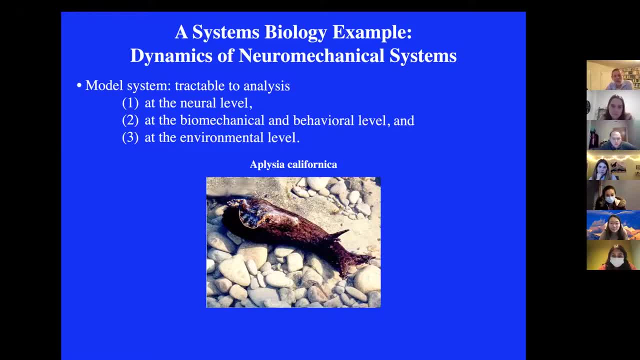 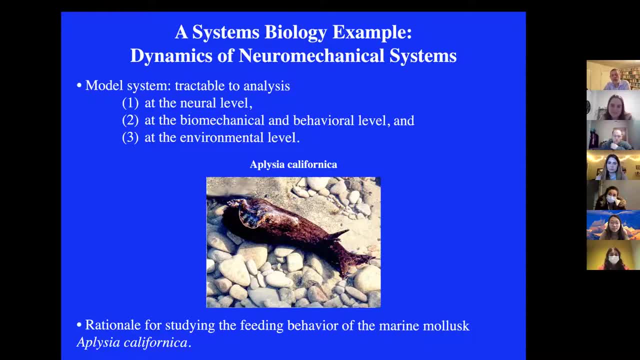 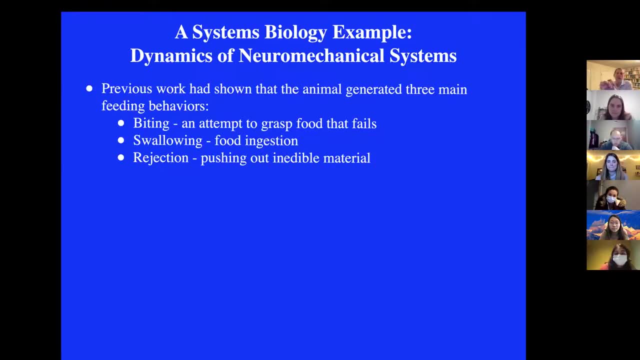 show you, creating models of its behavior is not that difficult. At least we've shown that we can make progress on that. Okay, so previous work has shown that the animal generated three main feeding behaviors. One is an attempt to grasp food. that fails, and that's called biting. 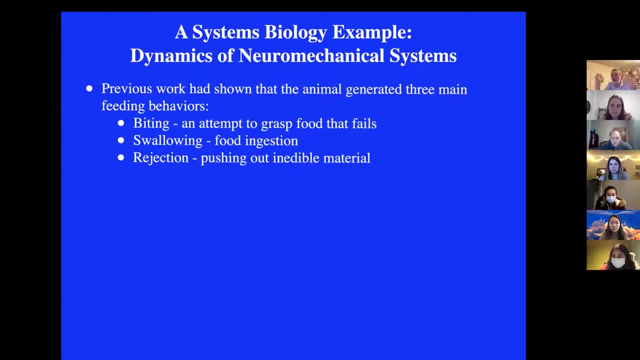 which is confusing, because when we bite something, we actually bring it into our mouths, But the person who studied this, Irv Kaufferman, called the attempt to feed biting. So that's what we're stuck with: Swallowing is when you actually pull food in, and rejection is when the animal 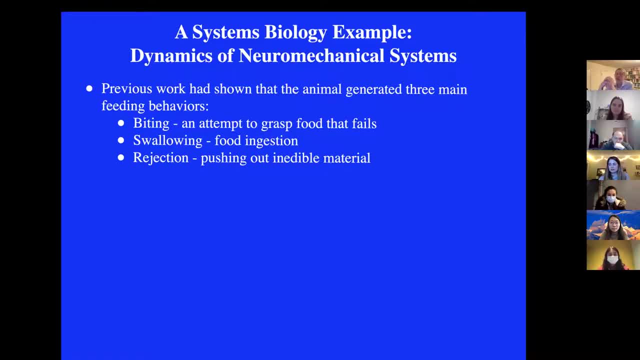 encounters something that's not edible, it pushes out. I should mention that this animal is also capable of learning that certain foods are edible and some are inedible. So it's complex enough to do some of the things that we take for granted, but it's tractable enough to analysis that we 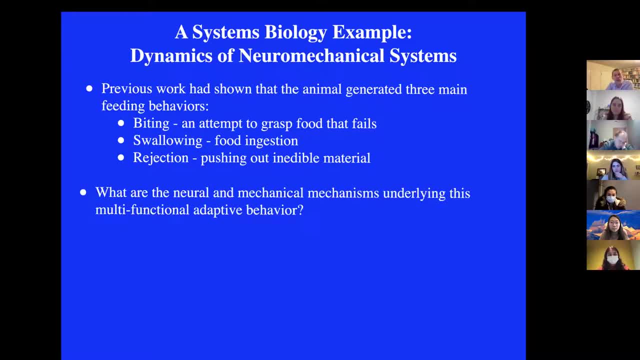 can understand how it's doing it, And that's what we'll be focusing on. So the question that I've been focused on are: what are the neural mechanical mechanisms underlying this multifunctional adaptive behavior? And so we address this question, both experimentally and by 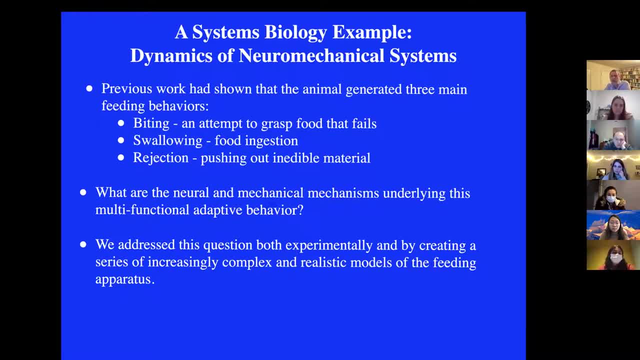 creating a series of increasingly complex and realistic models of feeding apparatus. So usually at this point I just jump to the latest model and I talk about what we've learned. Instead, what I'm going to do for you is show you the iterative process that we went through. 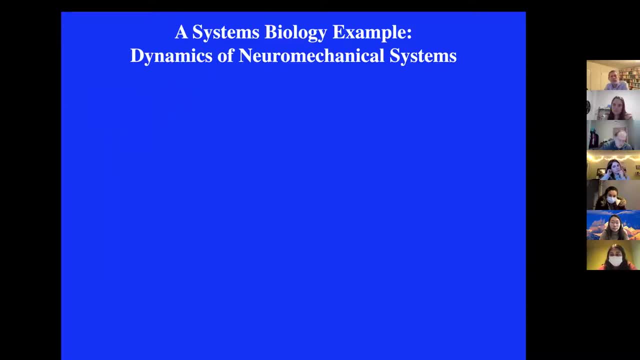 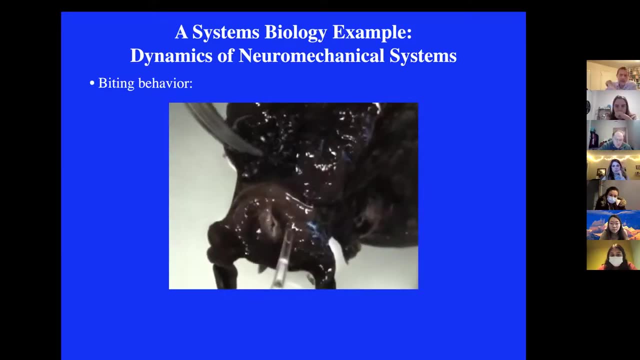 to actually understand more about this system. So here's an example of the biting behavior. Okay, you see that there's this thing that comes out and see if I can play that again. There's this horseshoe-shaped structure that came out and went. 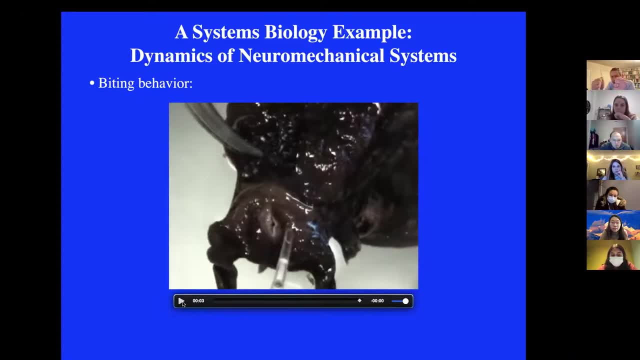 back in. So this is an example of a bite, with the animals attempting to get food and is not succeeding. And the question that we were confronted with, before even talking about multifunctionality, was: you know just how does it work? How does the animal do that? So 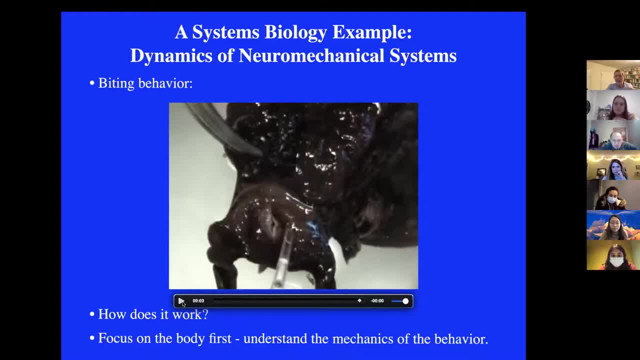 what we wanted to do was to focus first on the body and understand the mechanics of the behavior. Now you have to understand how unusual that is. Most people would immediately get to the nervous system: throw the body out of the animal's body. throw the body out of the animal's body. throw the. 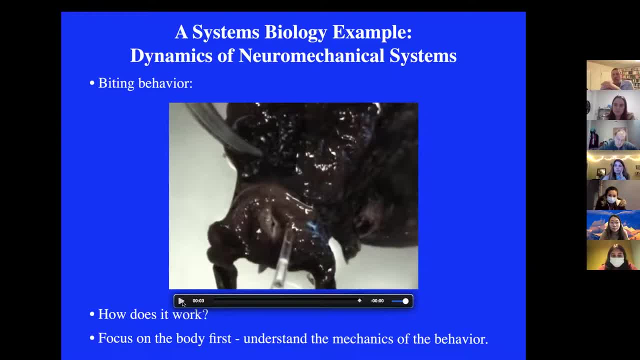 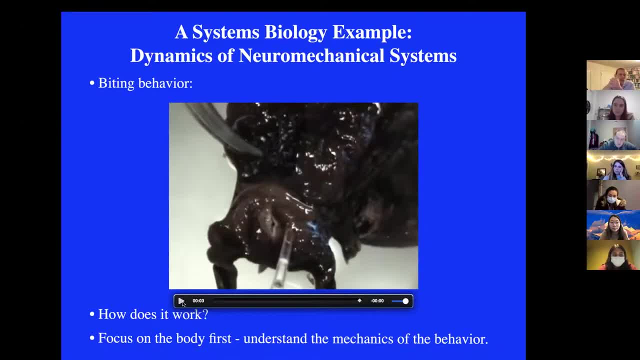 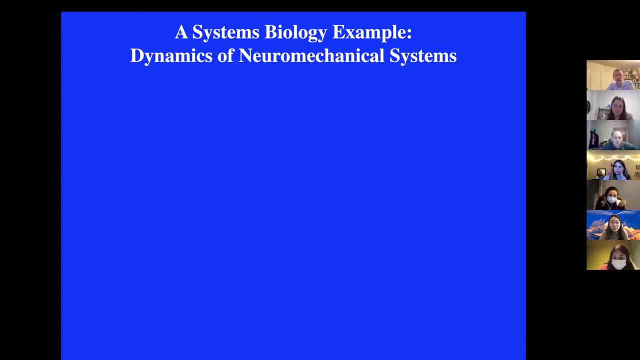 this have done, But we were the rather weird group that instead said no, the behavior is how the body and the behavior how you interact with the environment. So we really need to understand the biomechanics, the mechanical properties, the musculature and so on. Now a little. 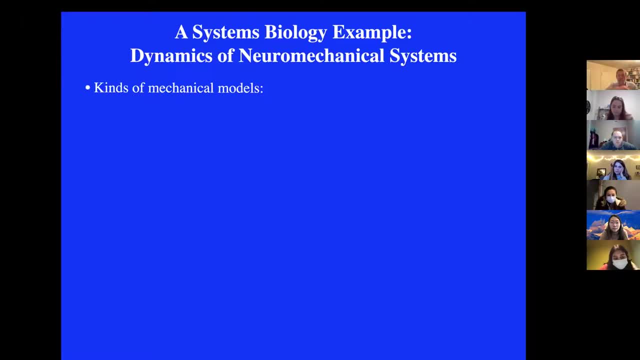 background is necessary because probably not all of you think about mechanical models on a daily basis. I mean, maybe some of you do, but it's certainly not so something I knew about until I came to Cayce and started to interact with people in mechanical and. 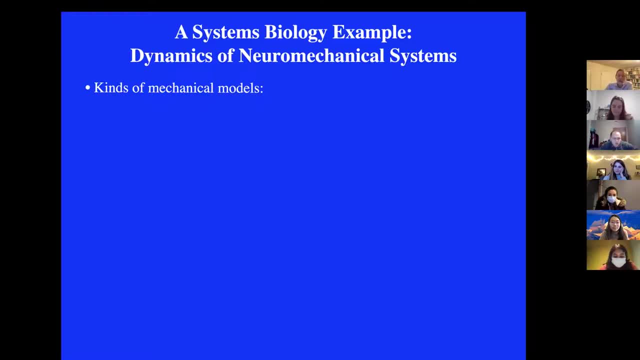 biomedical engineering, like Pat Krakow and Joe Mansoor. So some models are basically what are called kinematic models, And there the movements are constrained by geometry. So if you had a limb and what you wanted to do as a kinematic model, you would have a pin joint and you would ask if I 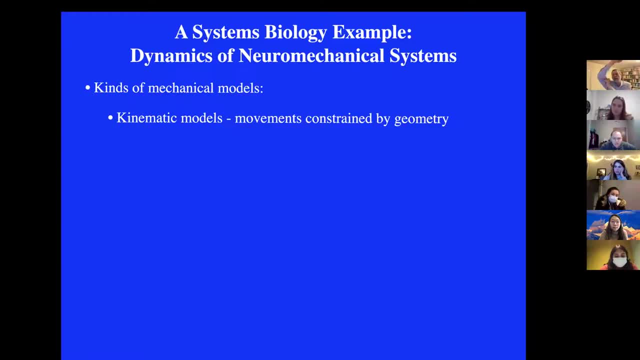 have a length here and a length here and I have a joint here. write down the equations that involve some science, And then you would have a pin joint and you would ask if I have a length here and a length here. And then you would have a pin joint and you would ask if I have a length here and a length here. 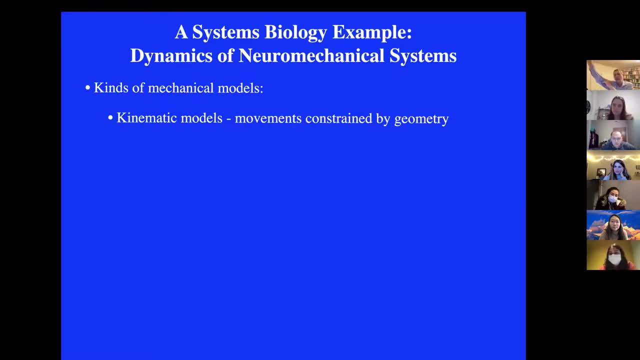 And then you would have a pin joint and you would ask if I have a length here and a length here For how this part of the limb would move relative to that point. Now, the problem with a kinematic model is it doesn't have any forces, So your model could easily have this part of the arm go right. 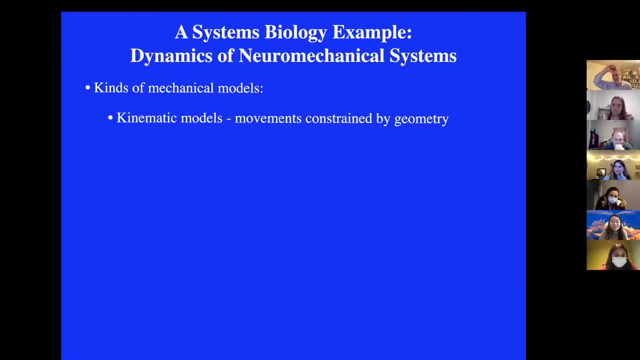 through this part of the arm, this upper part of the arm, go through the lower part of the arm, because there's no constraints in terms of forces unless you impose them, But you can get a sense of the geometry, how things move, and that's very important. Now, if you have a limb and you want to, 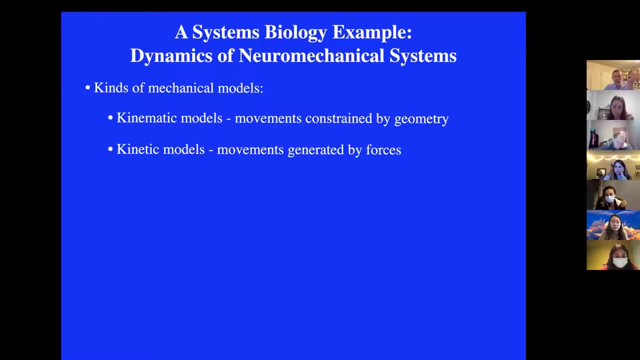 now the alternative- and often people build on this- are kinetic models, And these are models where you actually have the force generating muscle and you would have a joint and then you would activate the muscle And because of the mechanics of the joint and its relationship to 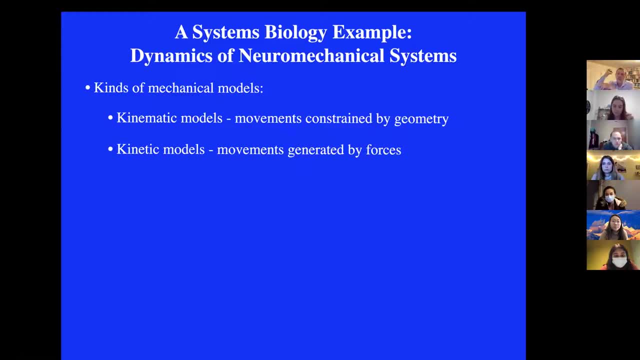 the forces, you would get a torque which would then move the other part of the limb and you would actually see movement. So you get kinematics out of the kinetic model. but the kinetic model actually represents the underlying forces and it usually has an equation of motion. 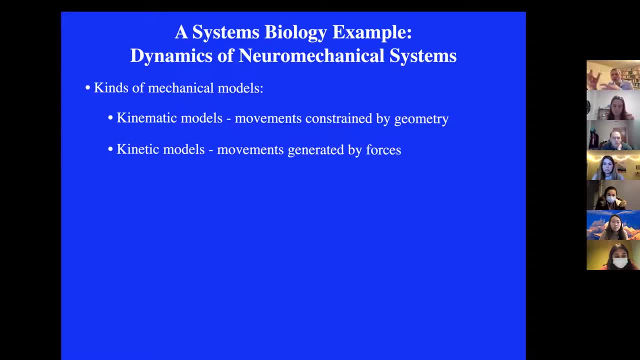 Again based on Newton's laws describing how those forces are applied, where they're applied and so on. So this is what mechanical engineers do: to understand things, And both statics or kinematics and kinetics are very important If you're building a bridge. 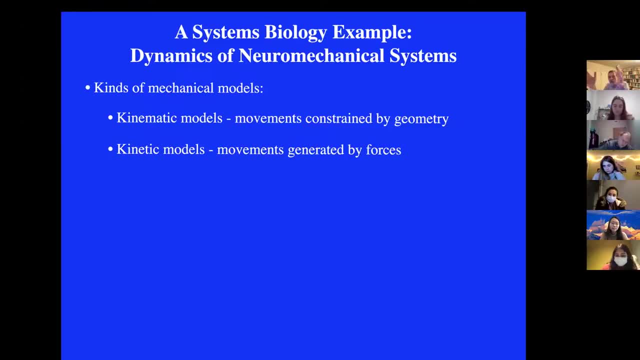 you obviously want it to be statically stable, but if the wind comes and starts swaying the cables back and forth, you also have to make sure that the forces that are generated are ones that the bridge can withstand, And when you have traffic pounding on it and the bridge 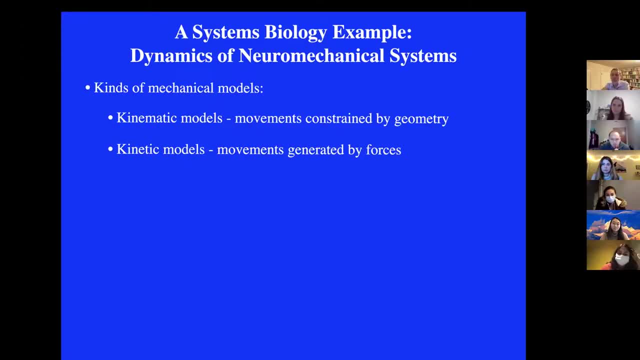 the bed of the bridge starts moving up and down, either in the wind or in the traffic. you don't want to have what's happened in rare cases. I don't know if any of you have seen their movies- You can look it up- called Galloping Gertie. There was a bridge where they hadn't done. 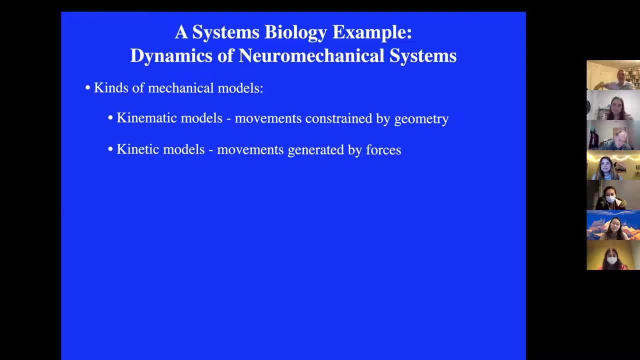 this properly, and it started to resonate at frequencies that actually destroyed the entire bridge. It fell apart. So you really have to know both, But these are the kinds of things that engineers spend a lot of time worrying about. The other thing that you can deal with is the animal's. 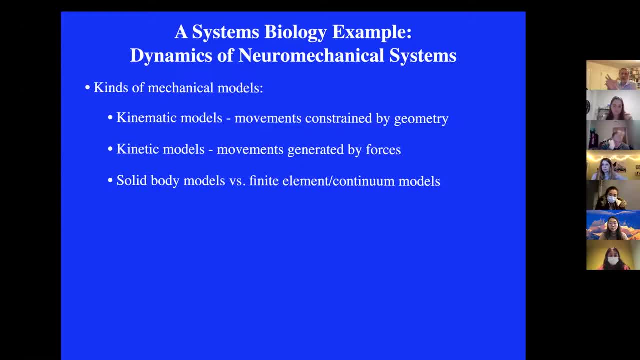 soft. It's soft bodied And you could, for that to get the soft body, use a finite element or continuum model. But the way most models are made is you start with solid bodies and that's much easier to deal with. There's much less computation. So we decided, after thinking about it, that our 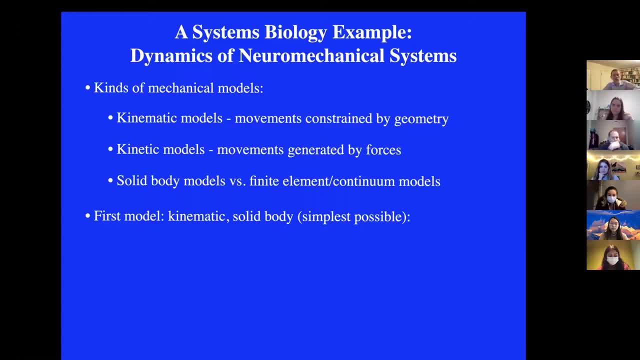 first model should be purely kinematic and it should use solid bodies, And this is essentially the simplest possible model. So this is our first model of the feeding apparatus right here, So I'll let it run and then I'll talk about it. Now there's a muscle back here which is represented by the line, And what your mind tells you is the. 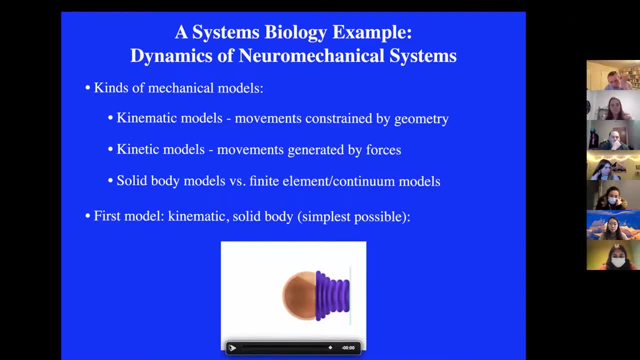 following. I'll just run it now, As this contracts. it pushes this forward, Then it's going through these rings which are kind of like donuts, And then, after it relaxes, the donuts start to squeeze and they push it all the way back And then it relaxes back to its original position. Seeing this, 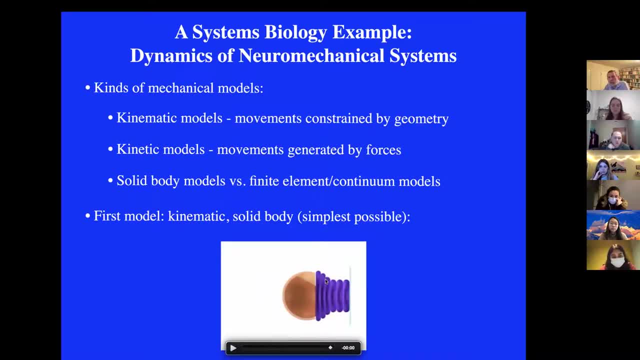 allows you to kind of intuit what the different muscle forces must be. But that's not actually how this model is working at all. This model is taking this ball, moving it backwards and forwards and forcing the geometry to stay constrained. So as I move it backwards, each of these rings 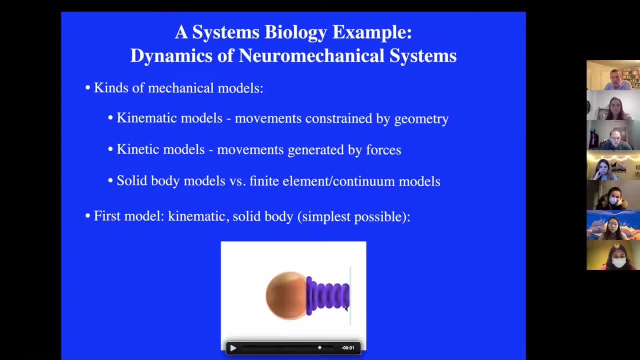 has to stay in touch with the previous one. And if it gets shorter, because its volume is constant, it gets fatter. Okay, and then I'm just drawing on top of this the rotation of the surface that you saw coming out to grab it. So I'm only moving the ball back. 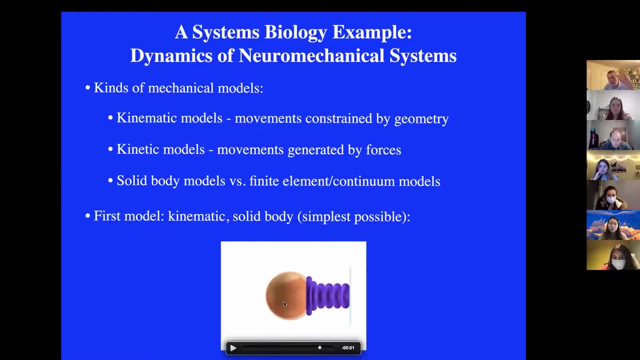 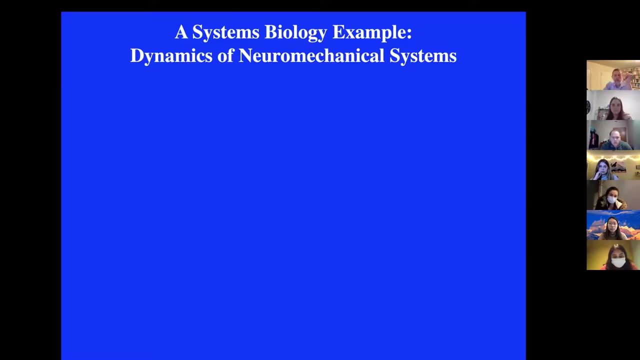 and forth. It's a pure kinematic model, but our minds are able to look at something like this and intuit what the forces might well be. So this is very interesting. It was very exciting And it made predictions about what we should see in terms of the shape. Let me just go back for a 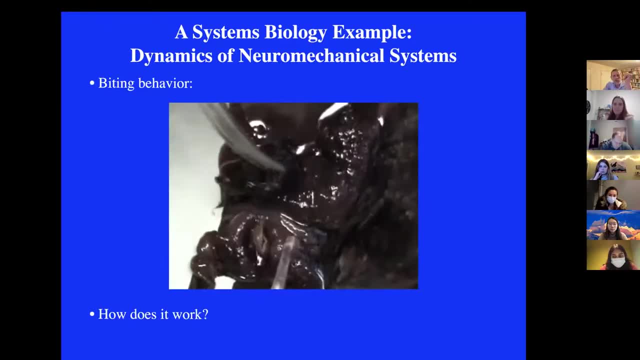 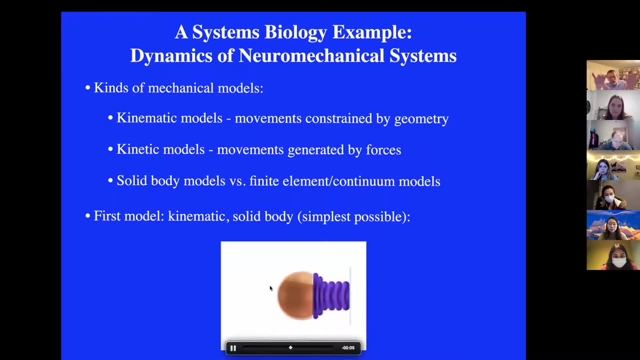 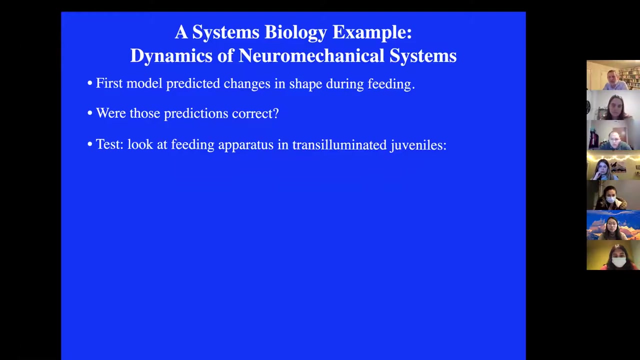 second. Let's see. So here it should look like a bull, And then, when it's at the peak of going backwards retraction, it should be very thin and skinny. So that was a prediction that this model made. So were the predictions correct? Now it turns out that when these slugs are really tiny, 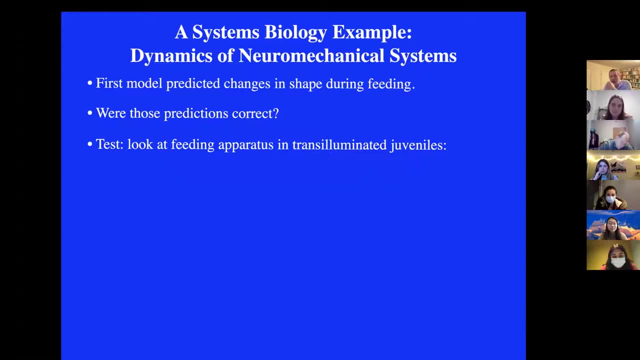 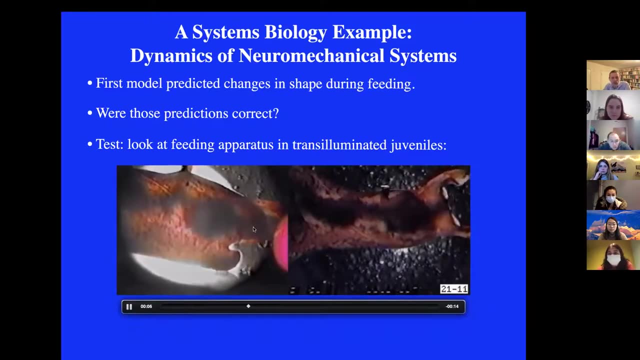 like 10 millimeters in length. they're almost transparent. You can trans-illuminate them And this is what you see when you do that. So you're watching the side and top view of this animal Chugging away on a little piece of seaweed over here. So this tiny, this is a you know. 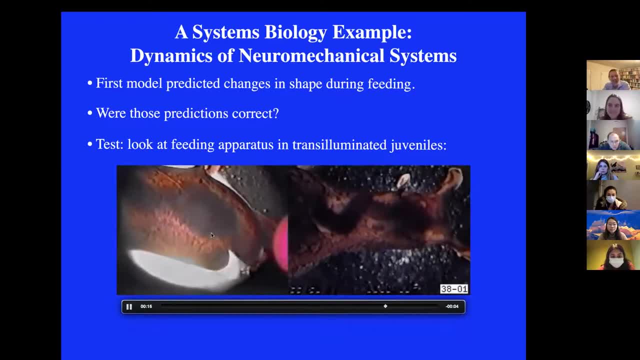 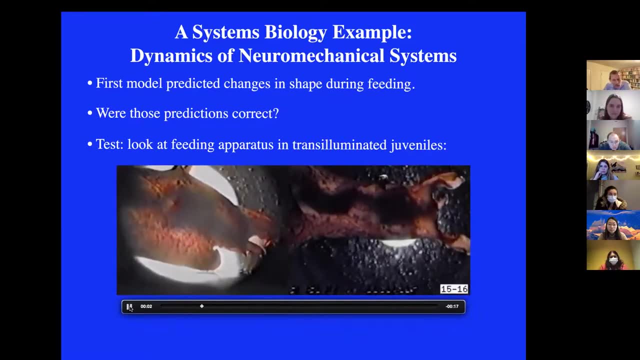 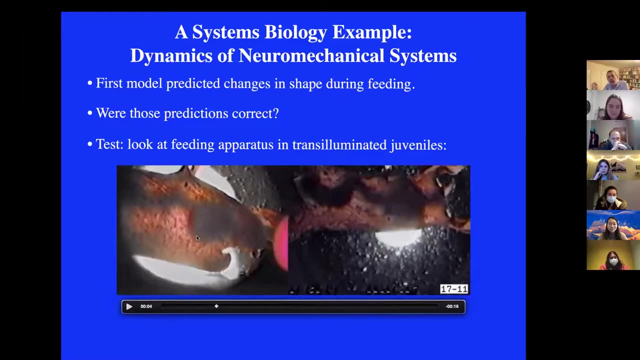 hugely magnified, because this thing is about this size. And the thing I'll draw your attention to is this: When this gets to the peak, let's see you're looking at the shadow it's casting. So here it is at the peak And look that looks like a ball. So that's peak protraction and it really 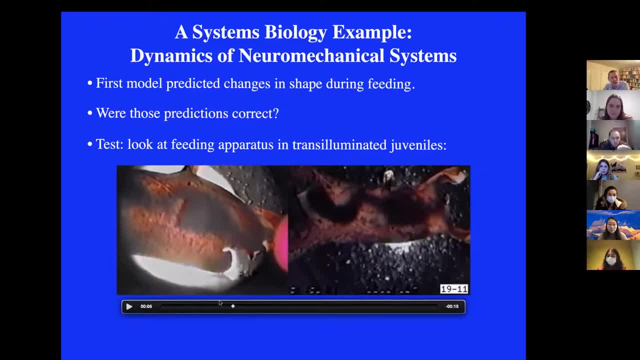 does look like a ball. But then let's look at what happens in retraction. Oh, let's see. You see how there's this thing sticking out the back. So the model did not predict that change in shape at all. So what we can say is the following: that the model was very successful for peak protraction. 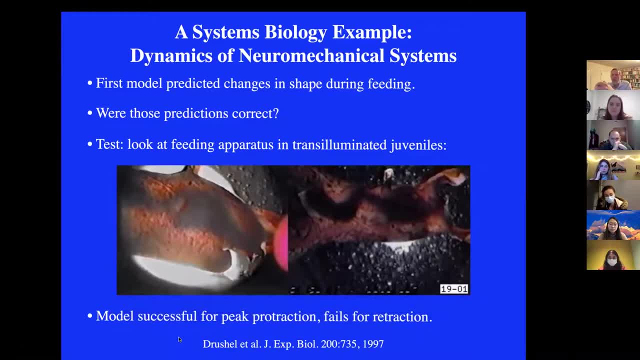 and it essentially failed for retraction. Now, ordinarily when you get a failing grade on something, you do not rejoice and jump around and say that's a wonderful thing. But when a model fails, if you know how to do modeling, you say, oh, that means we really don't. 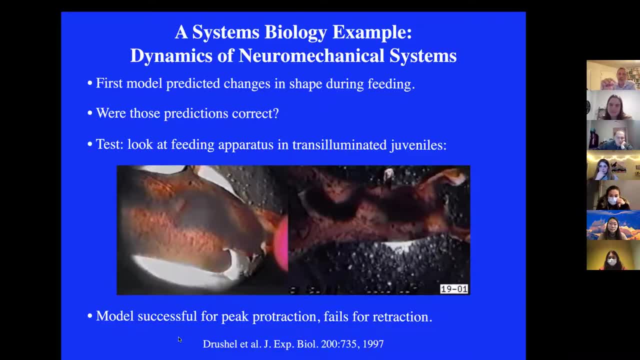 understand how to do modeling, You say, oh, that means we really don't understand how to do modeling. But that's where we don't understand it. Before we didn't even know what we didn't understand. So we're way ahead of the game. 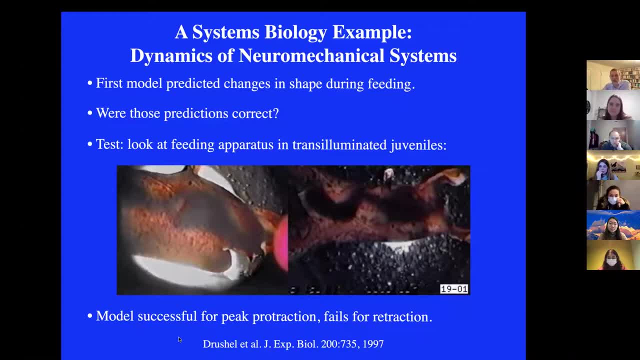 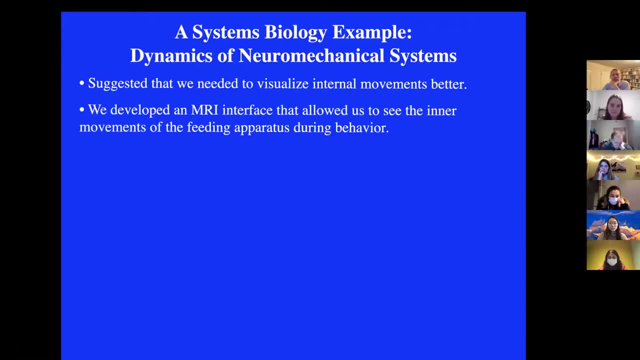 because now we understand something, and now we know better about what we don't understand. That's really very valuable. So that meant we should visualize the internal movements better, And so we developed an MRI interface that allowed us to see the inner movements of the feeding apparatus during behavior. This is work of David Neustadter for his PhD thesis. 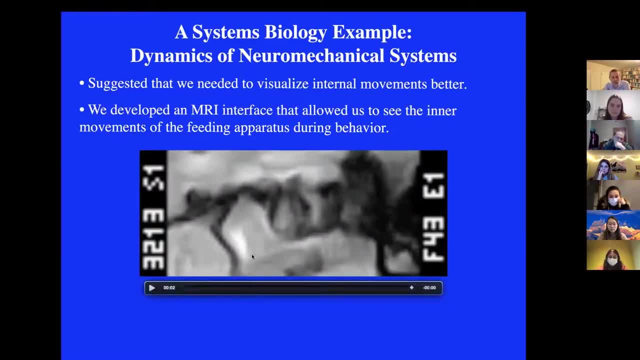 And this is the inside of a Colorado trail. This is a picture of the inside of the feed changes. So here are some pieces of the process. the Chinese graphically see themselves moving along the gap slug as it's biting using MRI. Here's the lumen of the gut, here's the esophagus, here's that. 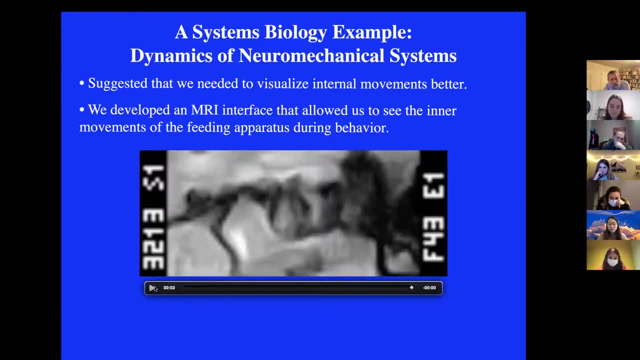 grasper that you saw from the outside. here's the jaws and here the grasper is whoops. let me see if I can grab this and do it more slowly. Okay, here the grasper comes forward all the way Now. 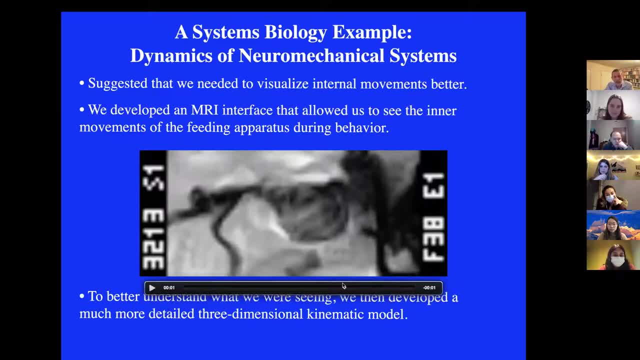 there you see the ball shape and then it goes back and you see how it changes shape and that gives you much more of that protrusion that we saw. And in swallowing, when there's a load here, that protrusion gets even bigger. That's because the halves of the grasper are closing and the 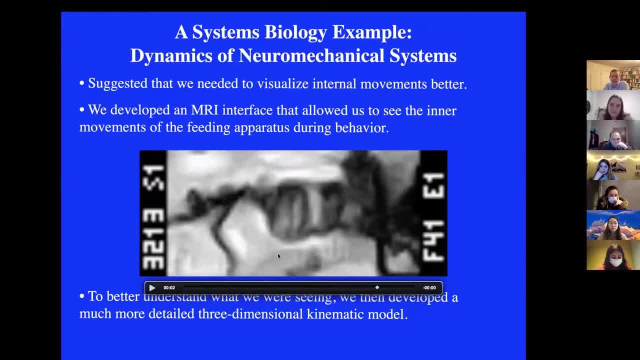 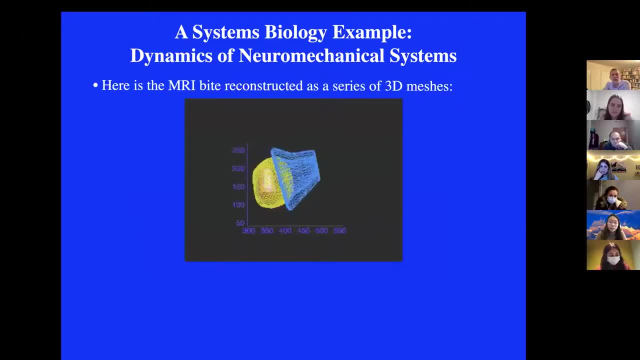 shape of the entire thing changes and protrudes out. So this led us to develop a much more detailed three-dimensional kinematic model, which I'll show you now. So this is reconstructing what you just saw as a series of meshes And again, just very briefly, what we're seeing here again. so the 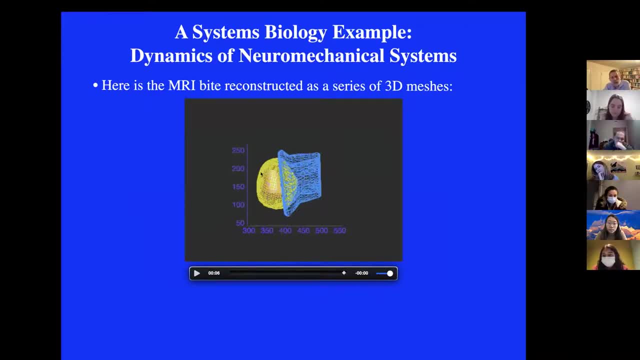 back muscle I talked about, and then the back muscle I talked about, and then the back muscle is not even shown here for clarity, but you can imagine that it's pushing this whole thing forward And these in front you can imagine push it back. And here this internal structure. 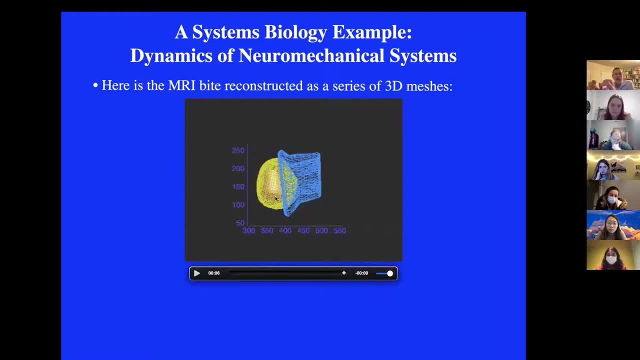 that you can see. this sort of reddish thing is actually the base of the grasper, And when the grasper is closing it comes out, And when it's open it's within it, So we can tell when it's. 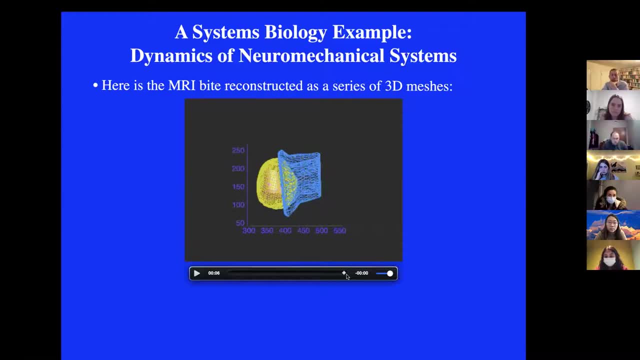 open and when it's closed, and we can use that to give us information. that's incredibly valuable Because this model tells us- it usefully predicts- which muscles are activated at different times to generate like swallowing behavior, But this also provided us understanding of how the muscles are. 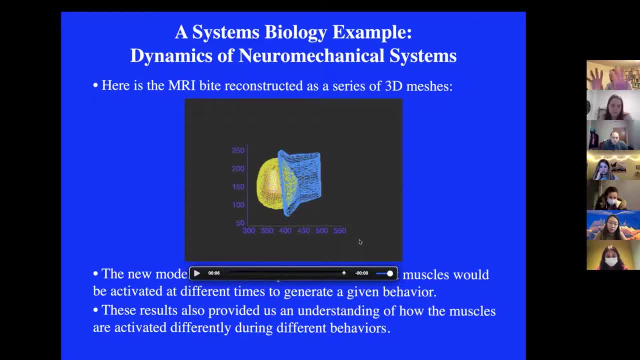 activated differently during those different behaviors- biting, swallowing and rejection. So now I'm going to take the time. You could hear me speak about this. If you type in Cheel Lab in YouTube, there is actually a series of videos that I put together where I go through an excruciating 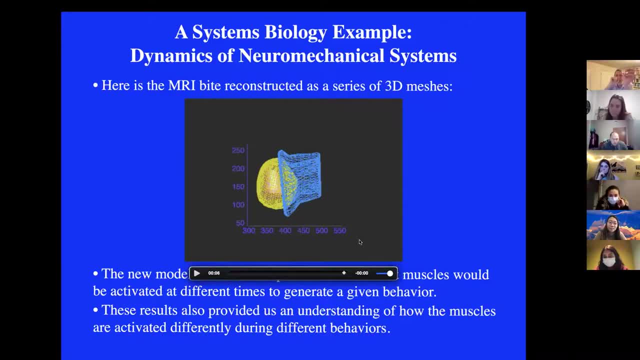 detail how biting, swallowing and rejection work both mechanically and neurally, and give you all the references if you're interested in that. I'm not going to take the time here. I wanted to show you an iteration of models that led to deeper insight, And then what I've left out, of course. 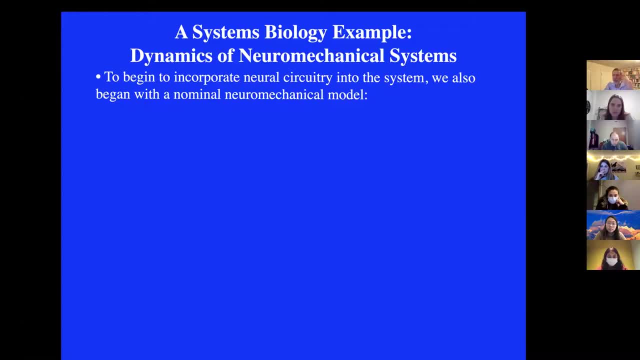 is the neural part. But we do the same cycle. Instead of putting in super detailed, very, very elaborate neural models, we started off with a much, much, much more nominal neuromechanical model. So the neuron pools represented by these three brightly colored circles there. 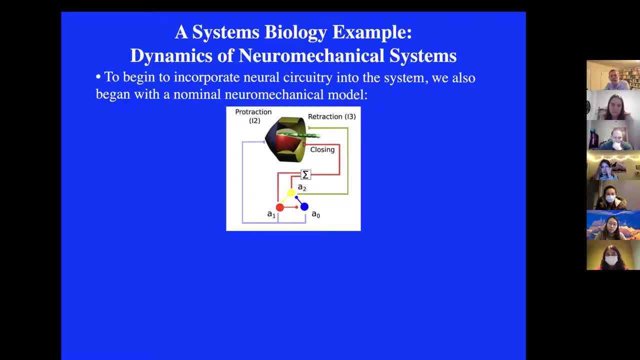 A0,, A1, and A2, and you can see a very simplified representation of the feeding apparatus which can open, close or move forward and back. Okay, so we have simplified mechanics, and then there are these three pools. 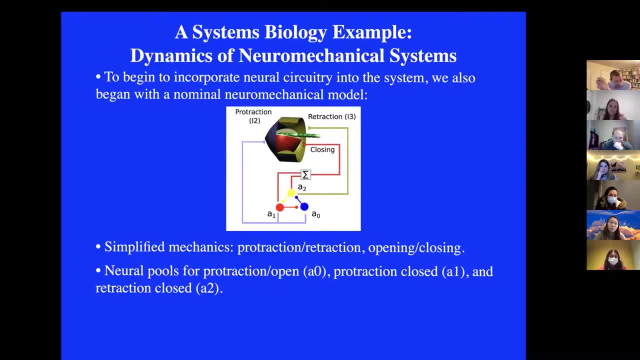 one for protracting, moving forward open, being closed as you protract and then retracting closed, And we set up inhibitory interactions between the neural pools using, basically Lotka-Volterra dynamics, and this created something called the stable hetero-clinic channel. 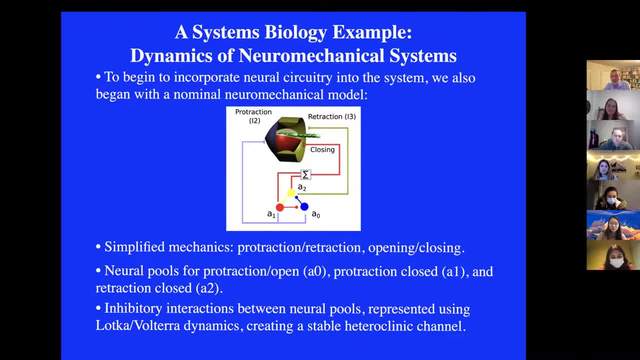 Now those of you who've taken Bio300, look at Lotka-Volterra. instead of freaking out, they say, oh yeah, a predator-prey. I've seen that kind of stuff before, And so this is super simple. 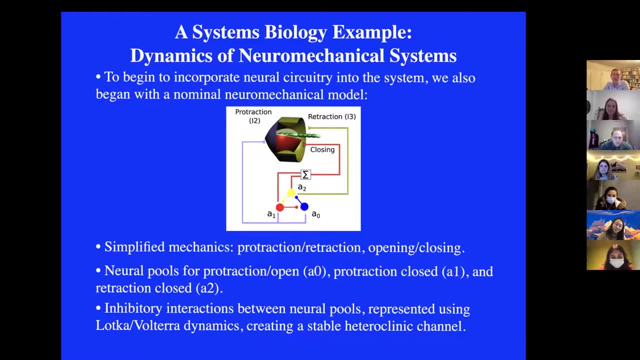 Now stable hetero-clinic channels again. for those of you who don't understand what I say in the next few sentences, don't worry, just take Bio300 and it'll all be clear. So a saddle equilibrium point is one in which, in one direction, 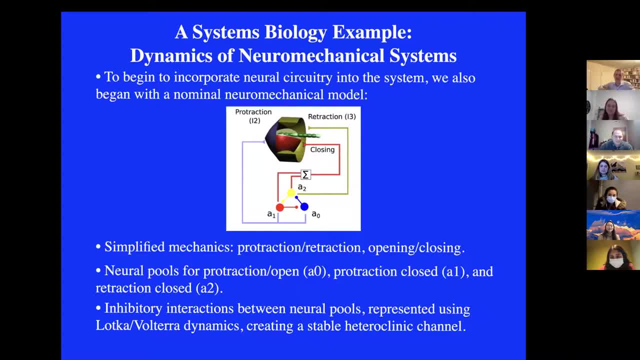 you are stable and you're pulled in in another direction. you're unstable and you go away. Now, if you take three saddles and you take the unstable part of one and let it go to the stable part of the second and then take the unstable of the second, 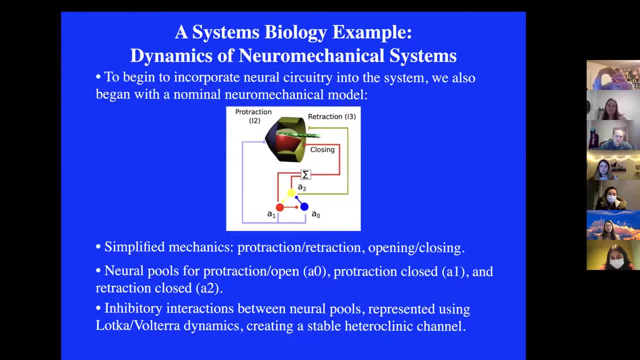 and let it go to the stable of the third and take the unstable of the third and let it go to the stable of the first. you can follow that. I create a triangle and that actually will oscillate. Now the problem is: 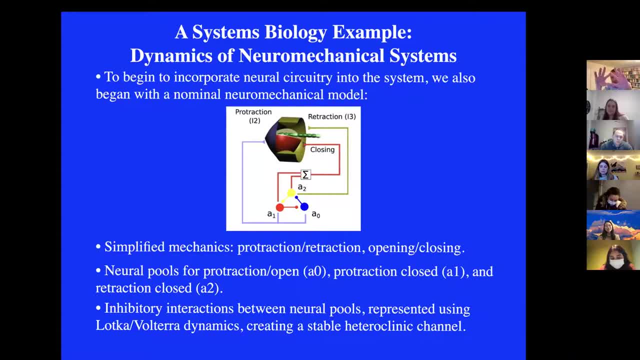 since these are each equilibrium points. if you get pressed onto them, you'll stay there forever. so if you add a little noise, you will dwell as long as you need to where you need to, and then move to the next and the next. 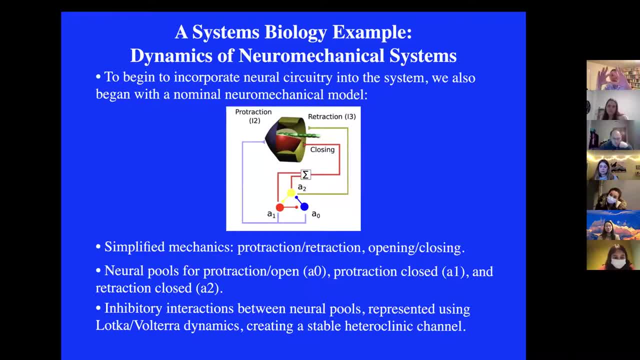 So this is unlike a limit cycle where you can't stay anywhere. you have to keep moving around the cycle. a stable hetero-clinic channel allows you to dwell for arbitrarily long times at different configurations. Now, none of that made any sense. 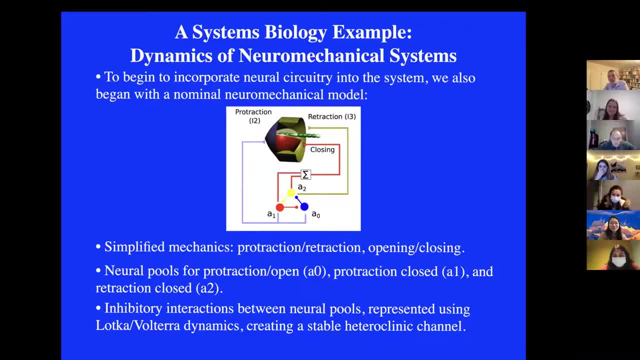 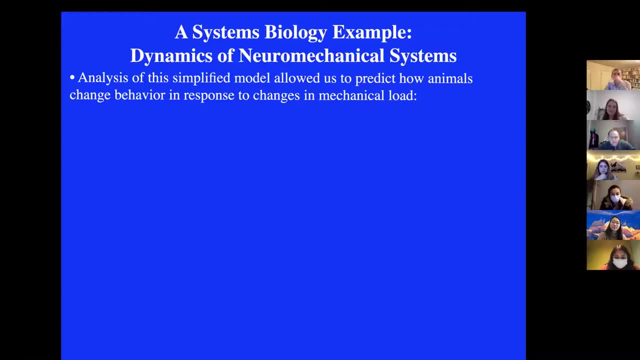 take Bio300 and it'll make much more sense. okay, But again, you can ask me more questions later. Okay, so analysis model allowed us to predict how animals would change their behavior in response to changes in mechanical load. This is a projection. it's a six-dimensional model. 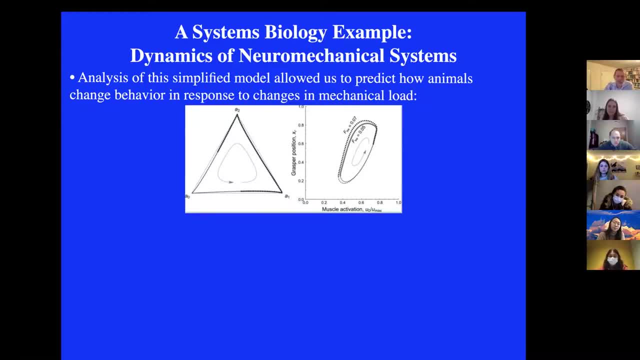 and you're looking at two three-dimensional projections. On the left-hand side, those three motor pools, A0, A1, and A2, are projected down. turns out that they live in three dimensions, but they take up only about a triangular space. 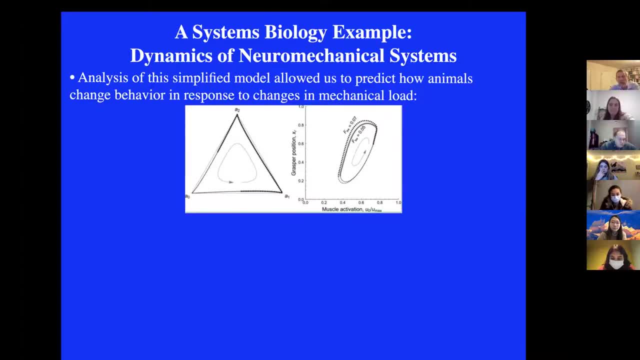 so you can just press them down onto a plane and you haven't lost anything. And the solid line shows what happens when you increase the load on the system by increasing the force on the seaweed by 40%, which is a substantial increase in the force. 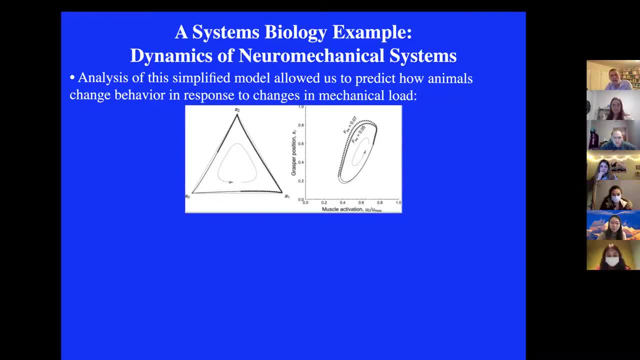 that the system has to deal with. Now, on the right, you're looking at a projection of the ratio of activations of the protractor and retractor muscle. that's along the X-axis, and then the actual position of the grasper. 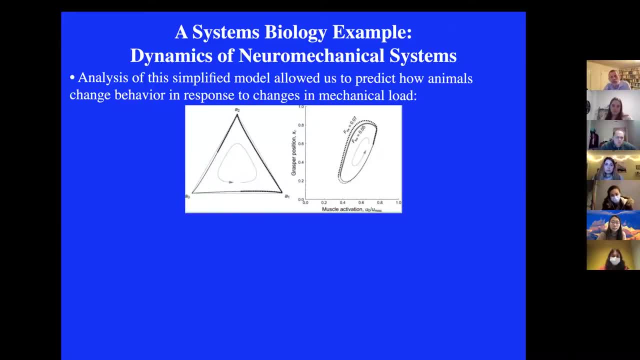 And what you can see from the change from the solid to the dotted is, as you go from a force of the seaweed of 0.05 to 0.07, which is a 40% increase. you see the dashing line shows. 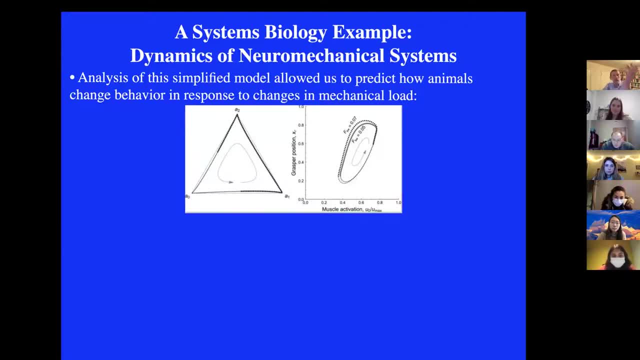 that the shape of the trajectory changes. okay, All right, so the animal is now handling. we're trying to ask: what does the animal do when it handles a tougher piece of seaweed? So you increase the load by 40% If you look at these projections. 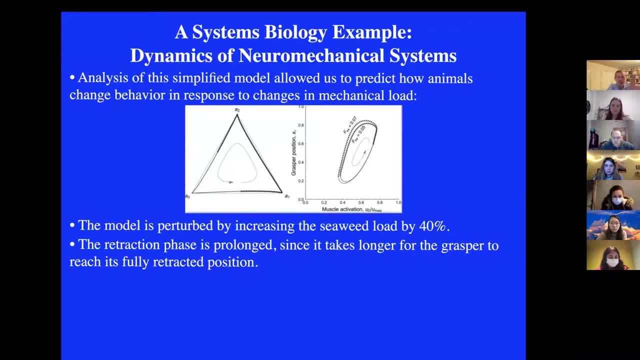 you'll see that the projections in terms of the neural stuff don't change. they're superimposed. It's all changing out somehow in the mechanics And what's happening is the retraction phase, the phase of pulling in is prolonged, And because it takes longer with the opposing force, 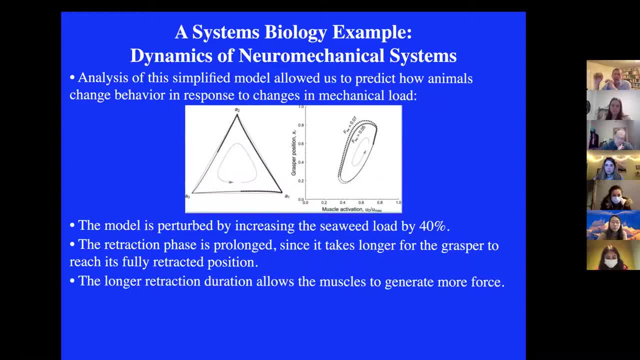 to reach your fully retracted position. The beauty of that is that these are slow muscles and the longer it takes to do something, the more force the muscles can generate, So that more force draws more seaweed in during that cycle. So you pull for longer and you do a little bit stronger. 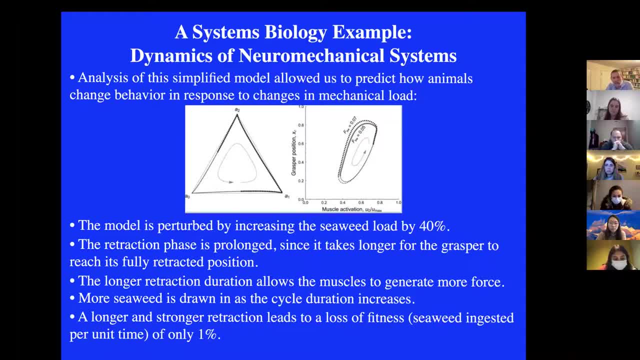 And the end result is that you only lose amount of fitness. that is, the amount of seaweed ingested per time of about 1% for a 40% change. So here's a deep question: How is it that animals are so robust and able to maintain fitness? 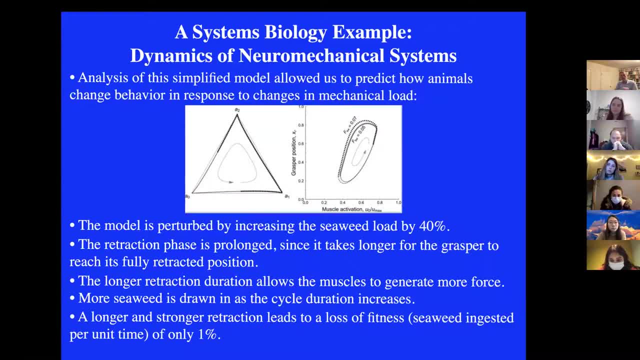 in the response to perturbations, And this very simplified six-dimensional neuromechanical model starts to answer that question. Okay, so this was published a few years ago. Now, the last thing I'll say in terms of this modeling stuff for my things. 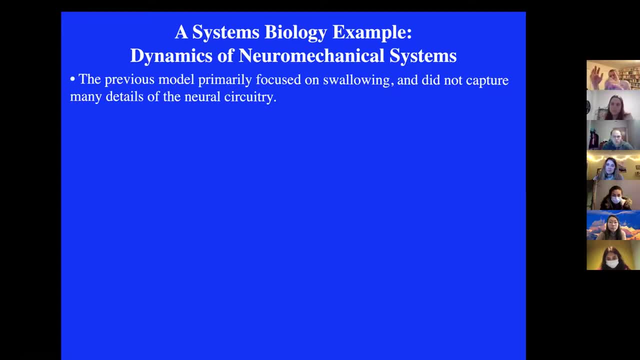 then we'll go on to more general stuff. is that this didn't talk about the question of multifunctionality? biting swallowing injection. That's one of the most interesting aspects of this system. If you have a- I don't know how many of you have had a Swiss army knife- 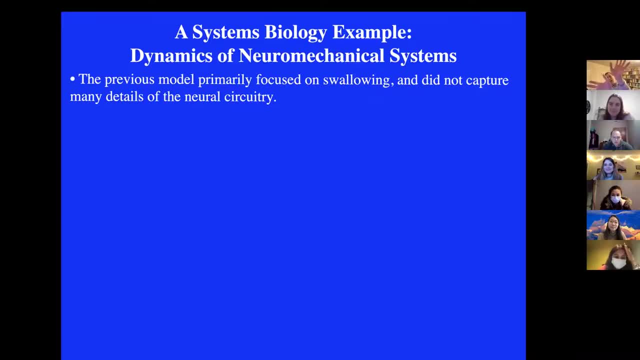 If you look at the ads, they show them splayed out like this: Could you use the knife that way? No, The scissors are gonna interfere with the forceps and the bobby pin and the awl and the corkscrew. You have to put everything away, except for one thing. 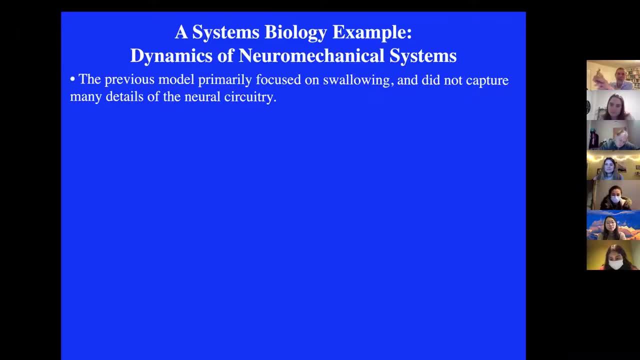 That's the tool you use, And then you put it away and you take out another tool. Now think of your hands. You can go from picking up a pen to pounding on a table, to unscrewing a jar, to playing the piano seamlessly. 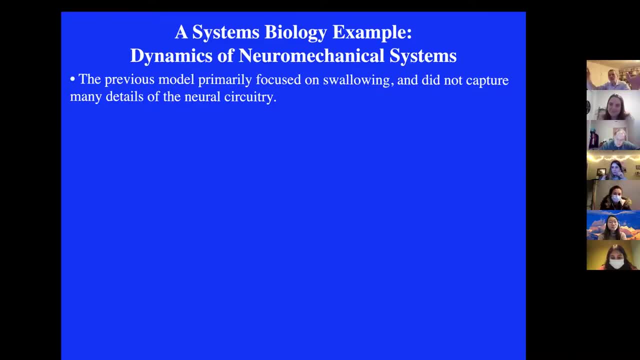 You're not inspector gadget. You don't have to keep on pulling out a new device. You have all of this in your hands by deploying the different degrees of freedom within them. So the question of multifunctionality is a very broad one, And to get that we needed. 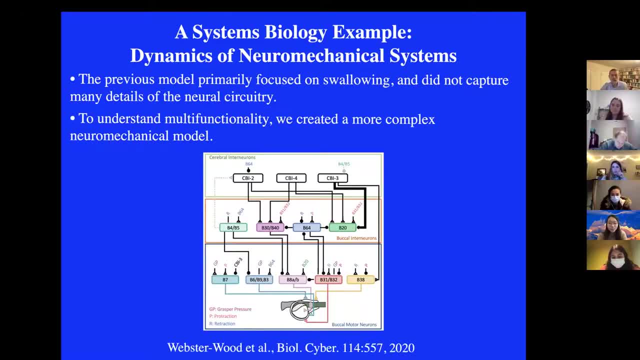 a more complex neuromechanical model, And this was done very recently with Vicki Webster-Wood, who's now at Carnegie Mellon, And what you have is at the bottom you see an image of the buccal mass. Above that, you see some of the key motor neurons. 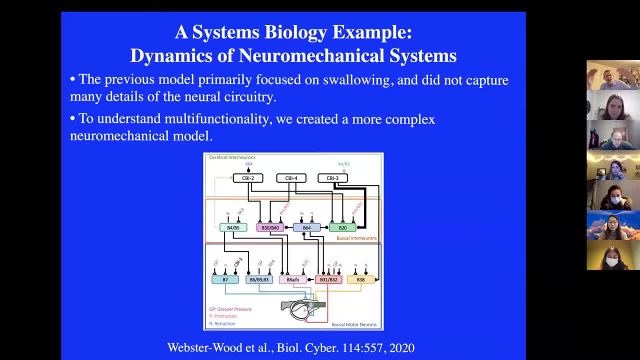 The level above that you see some local interneurons And above that you have higher order interneurons that are actually in another ganglion that's more encephalized. So that's a far more complicated model than the three motor pools I showed you in the previous one. But the plus is: 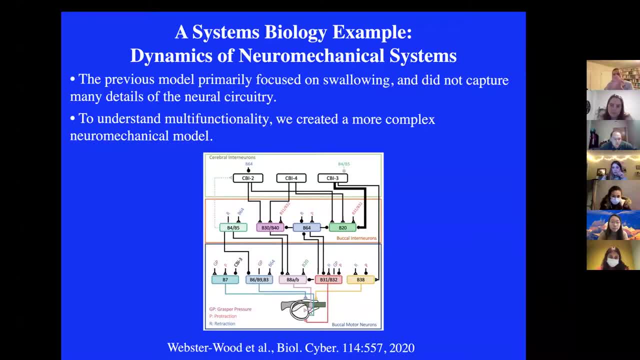 that you can now identify components of the model with components of the nervous system, And I should emphasize: what makes the system so amazing is you can actually identify cells in animal after animal and give them names. So B3 is a motor neuron that shows up in a certain 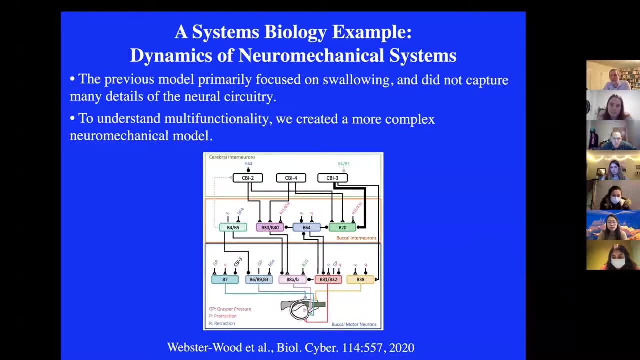 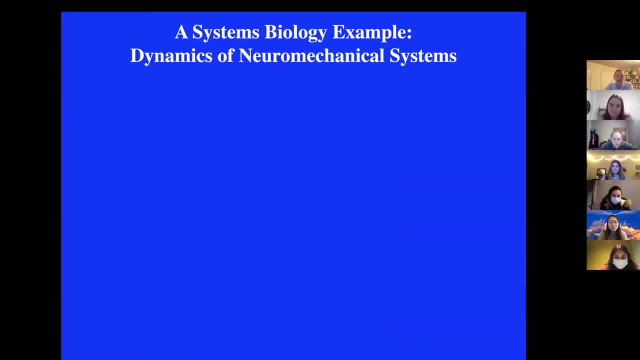 location and it innervates certain muscles and it has certain properties in terms of when it's active. So you can really draw these circuits in detail. That's what's attracted me to Plisia and others. And what do we find? So, to keep it simple, we made the neuron models very simple. 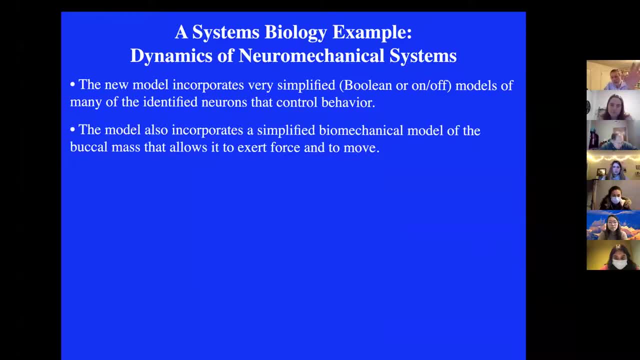 just on-off switches And we have the. biomechanics is also simplified, but we show that with appropriate sensory inputs the model can generate movements corresponding to three behaviors by adding, swallowing or ejection, And it can handle increasing mechanical loads with no change in the 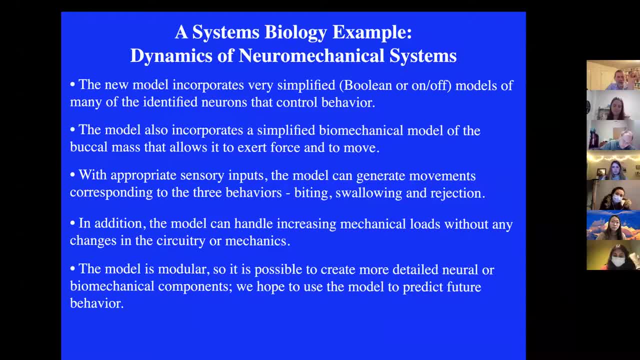 circuitry or the mechanics. That's part of the dynamics that's set up And the beauty is this is a modular model. So part of the ongoing research we're doing is to replace the biomechanical- very nominal biomechanical model with more realistic models and the very nominal neural 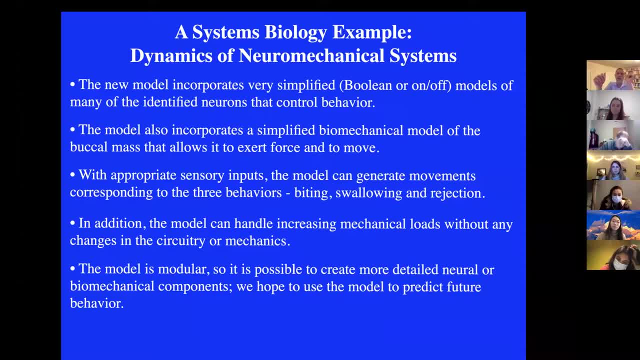 models, with more realistic neural models, And this is ongoing. And again, someone who's interested in this kind of research can approach me and potentially get involved in doing this if they, like You, don't have to love slugs to enjoy working in my laboratory, though it helps. 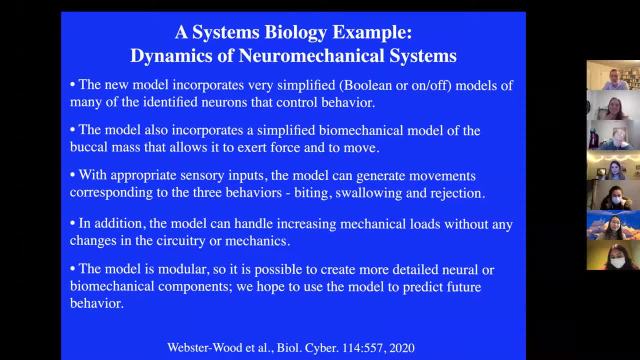 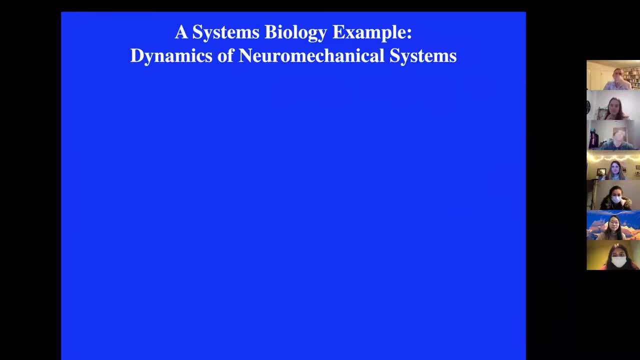 Okay, And anyhow, this is part of that paper that was recently published, last year. All right, Let me draw some general lessons from what I've just shown you, And if you didn't follow all the details, don't worry about it. We call the approach that I've been talking about is the demand-driven complexity. 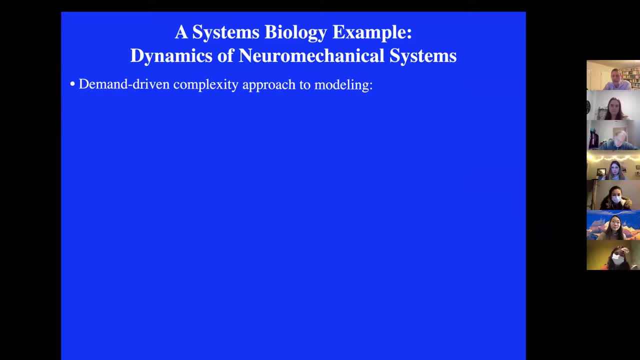 approach to modeling. That was actually an idea that was formulated first by Randy, but I've just illustrated for you concretely. The first point is that modeling is an iterative process. The goal is not a perfect model, but a model that is a perfect model. that is a perfect model. that is a 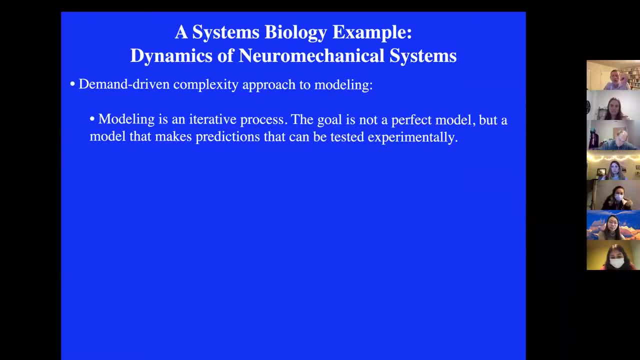 model that makes predictions that can be tested experimentally. The second point- and I emphasize this at the appropriate time: model failures. Failures are opportunities to better understand the system. to focus on the next most important aspect of the system that needs to be understood. 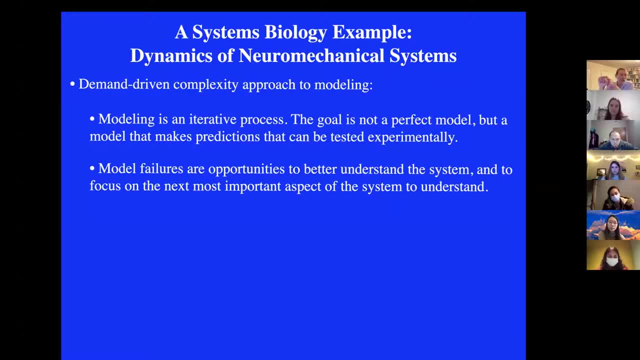 That's why failures are so important. If you create a model that is so vague that anything goes, then it hasn't given you any information. And you create a model that's so perfect that nothing fails, Okay, Maybe you're done, But maybe you haven't perturbed the system. quite right to see where the model fails. 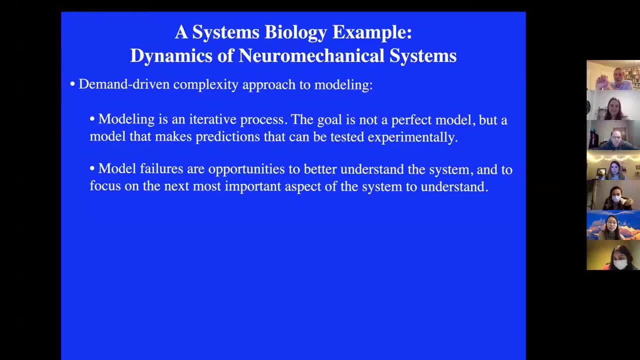 Because if the model is as complicated as the original system, you might as well just study the original system and throw away the model. Models are supposed to be somewhat simplified and that means they're going to have inaccuracies, But the goal is to make those inaccuracies smaller. 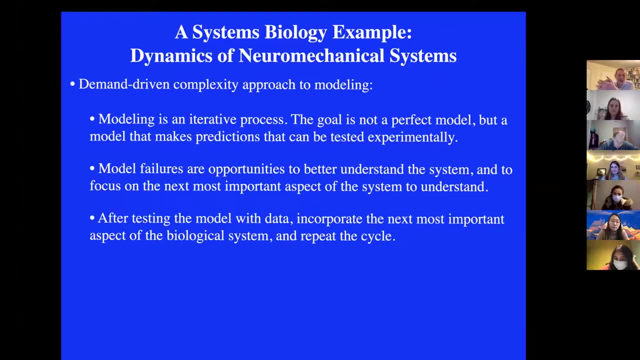 and smaller over time. So you test the model with data, you incorporate the next most important aspect of the biological system and you repeat, And that's the key idea. A lot of people don't get that When they think of modeling, they think of the model, They think of the model, They think of the model. 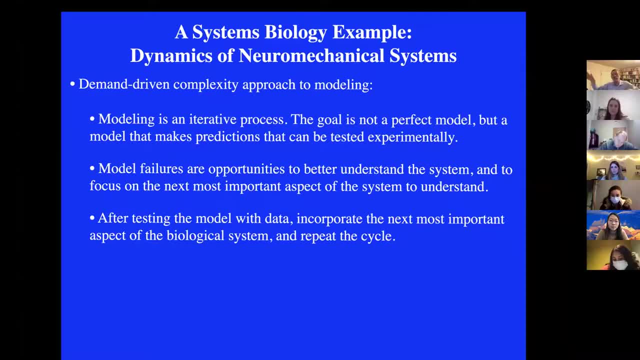 And that's the key idea. A lot of people don't get that When they think of modeling, they think of the model modeling they think of I'm going to get all this data. It's too early to start modeling. 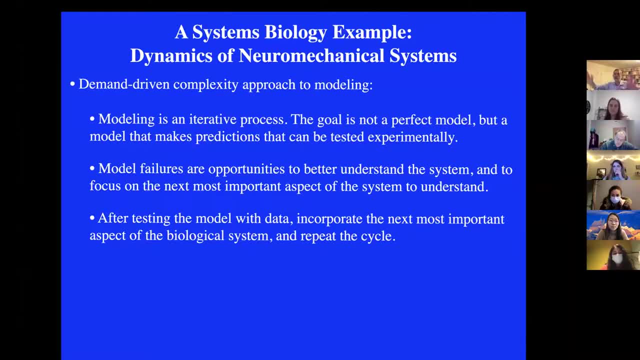 And once I have all the data, I'll throw it into this incomprehensive model and predict exactly what I need to know, And that almost never works. So the general rule is: you want to always develop the simplest model that captures the essential features of the system and add complexity only. 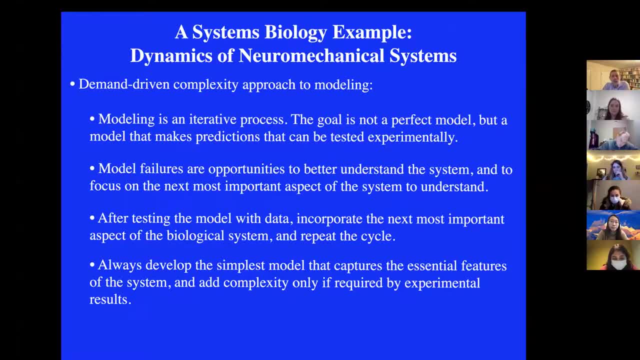 if required by experimental results. Now I want to emphasize that there is another aspect to modeling that I'm not focusing on here, because here I'm really focused primarily on the modeling experiment cycle. But there is another important aspect: Models allow you to explore the space of 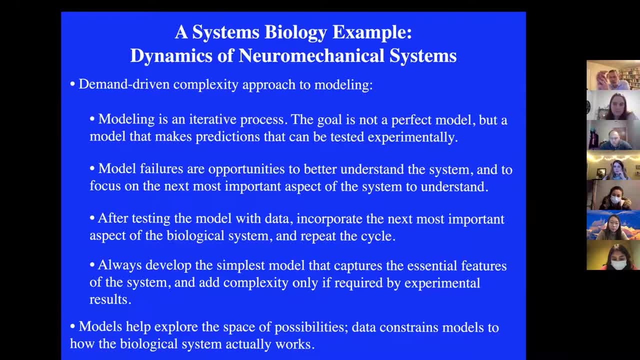 possibilities And having an understanding of that space is vital. In some cases people are so focused on creating super detailed, realistic models they miss the value and the power of a much more abstract mathematical model to give you a sense of the space of possibilities. But 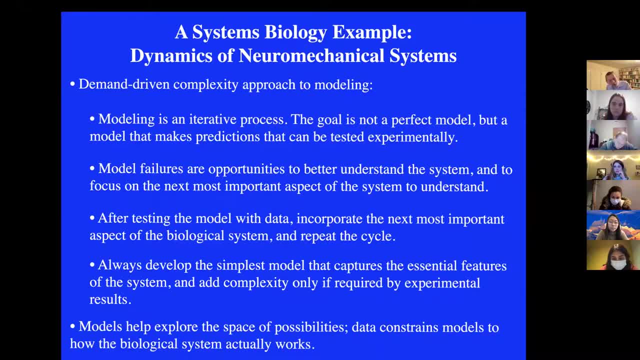 and this is where modelers have to always be patient with biologists. Data constrains, models to how the biological system actually works, And if you don't pay attention to those constraints, your models can be way off. And no biologist who is self-respecting is going to take seriously a model that says: oh, I've proven. 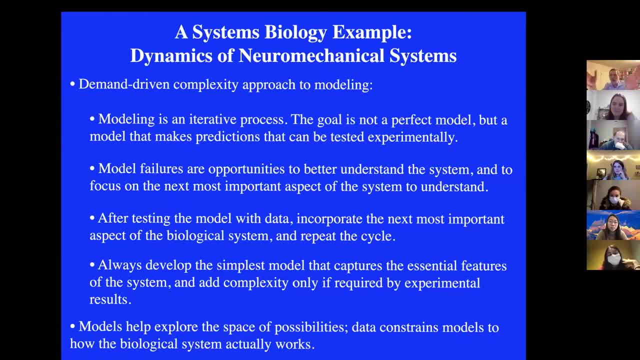 I have a theorem that proves that this is true. Go and show this in the laboratory Now. if the biologist looks at the model and it's left out everything that's important about the biological system, and they know that it takes 10 to 15 years. 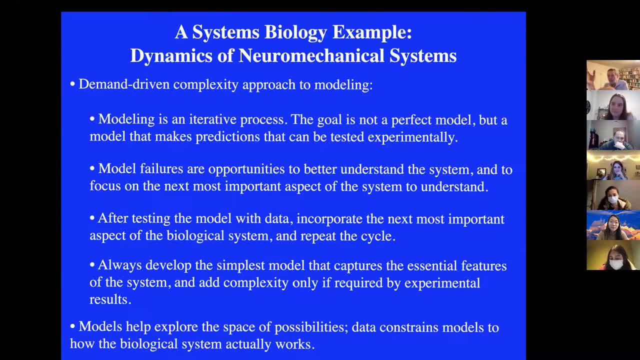 to do the relevant experiments. it is not surprising that they are going to walk away from the modeler and not pay any attention to what the modeler has to say. The key point I'm also making- and this is where a systems biology major can be unusual If you know both languages- 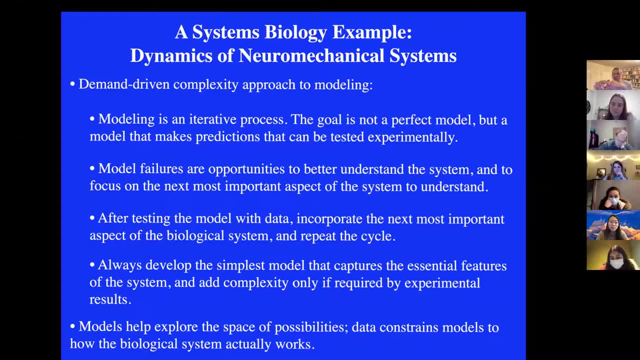 you can be a go-between, You can be a translator, You can be a bridge, You can go up to the person who's doing the experiments and say: have you ever thought of looking at this? And you know enough about the experimental work to actually not say something vague in general, but a specific thing. 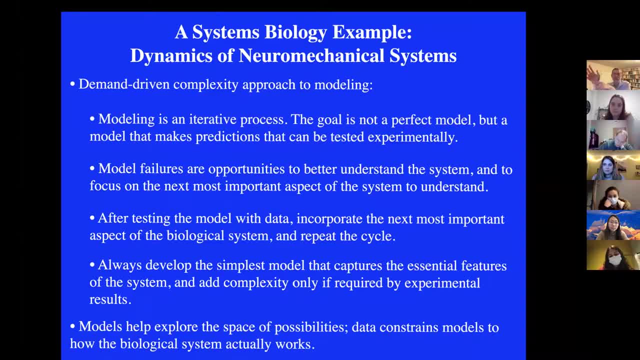 You can go back to the modeler and say: you know, it seems to me that we've left out this aspect from my reading and from what the biologist is telling me- And this is something modelers don't often get- Biologists actually know an enormous amount about their system, It's just qualitative. 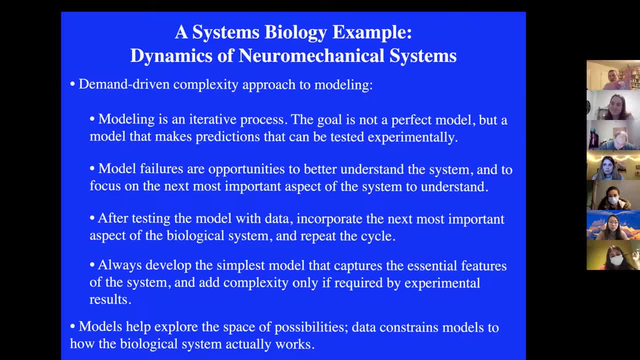 And it's expressed in biology jargon. So if you can get past the jargon and understand their feeling for the organism, the qualitative stuff, that's hugely powerful, unbelievably powerful. Ignoring that is stupid. But if you can understand that and think of how to translate that, 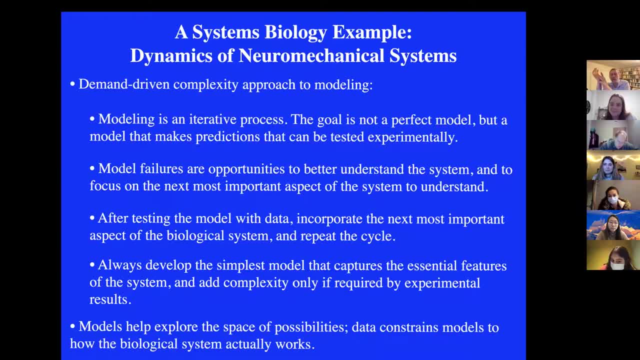 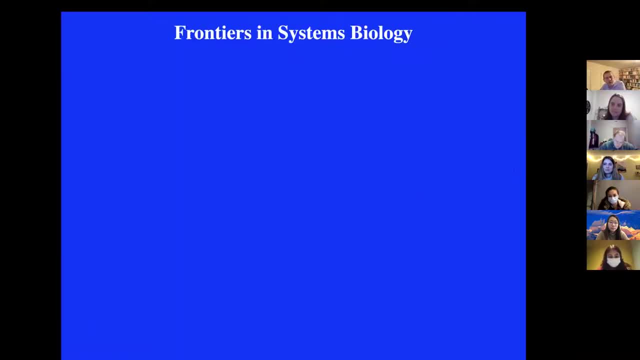 suddenly you can do things that nobody else has been able to do for making sense out of the system. So you have the superpower that other people don't, if you master both aspects. Okay, Now I'm going to just briefly talk about some of the things that I think are super cool. 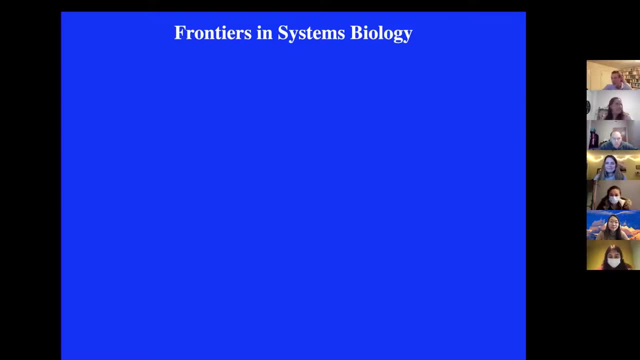 out there right now that any one of you could potentially contribute to, And then I'll wrap up. So five more minutes, I think I'll be done. So you may have heard of this. This is a protein folding problem. Proteins are composed of. 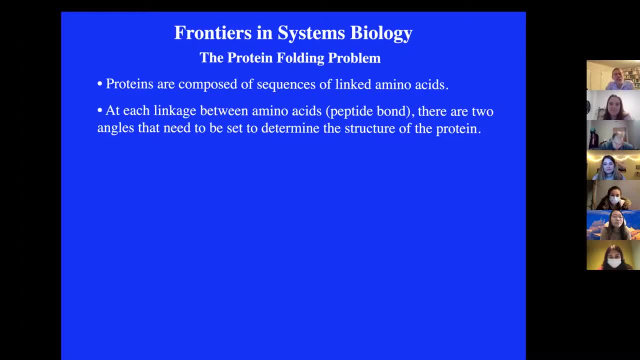 sequences of linked amino acids. At each linkage between amino acids, the peptide bond, there are two torsional angles- They're usually referred to as phi and psi- that need to be set to determine the structure of the protein. The peptide bond itself is rigid. That's the omega angle, But the 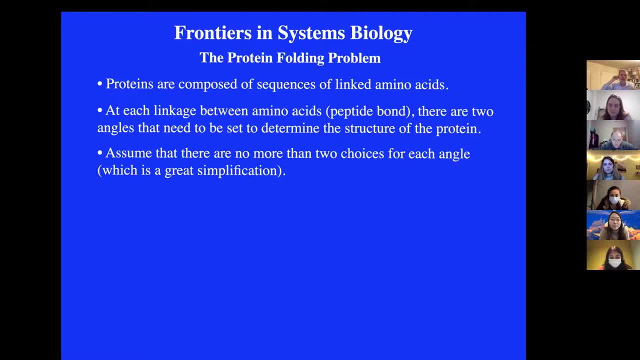 phi and psi. they can rotate. Now assume that there are no more than two choices for each of these angles, which is a gross oversimplification. They actually have multiple choices, But let's start with just two. So that's four possible configurations. It could be like this or that. 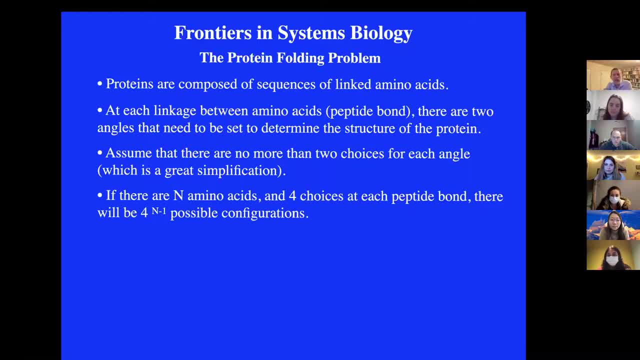 on this side or this or that on that side. Four possibilities Now. if there are N amino acids, four choices at each peptide bond, that's four to the N minus one possible configurations And lysozyme, which consists of only 100 amino acids. the number of possible configurations for 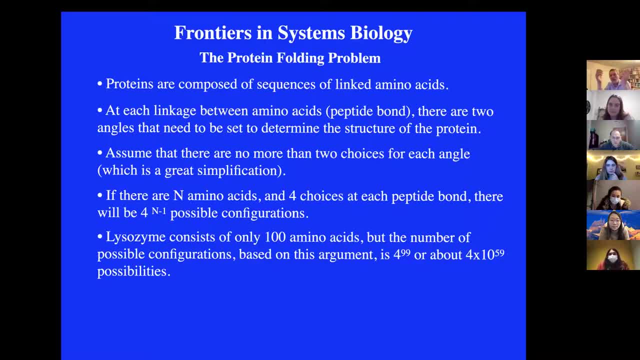 those torsional angles based on this argument is four to 100 minus one, four to 99, or about. I can't see that Number because my thing is covering it, but I think it's four times 10 to the 59th possibilities. 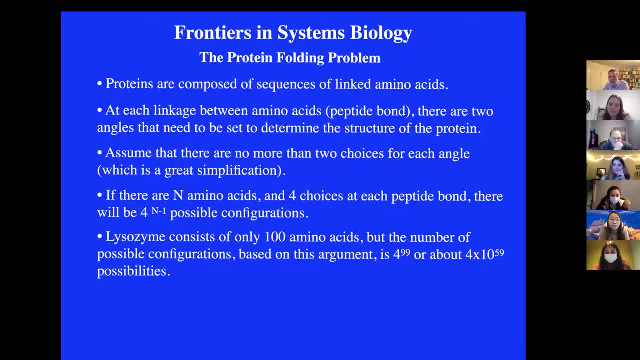 It's a huge, huge number. Okay, That's massive. But proteins this long and much longer fold in hundreds of milliseconds. They don't seem to be confused by all their possibilities. Somehow they find the right place. How do they do it? That's the protein folding problem, Okay. 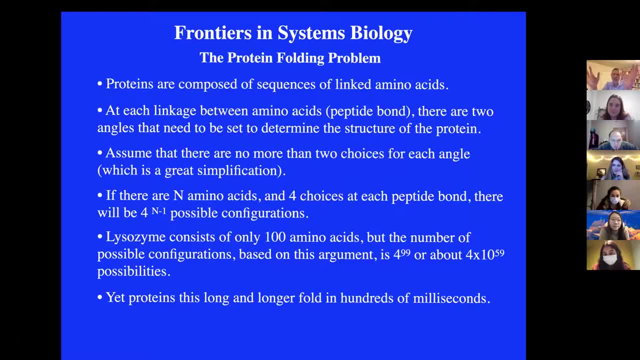 for those of you who know enough computer science, this is an MP hard problem As the data is formulated here. Okay, It's non-polynomial times, clearly exponential, but it's being done in polynomial time. Wow, Solve that. You've got a lot of. you'll be very famous, Okay, Now right. 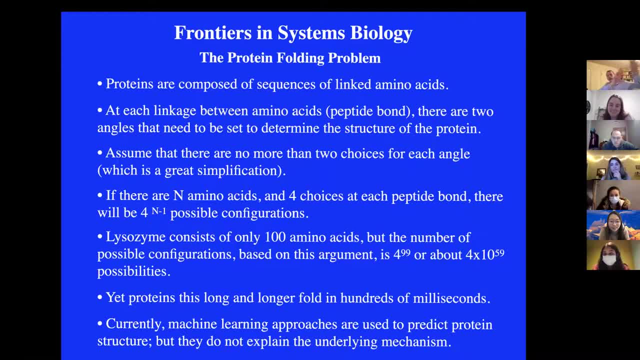 now machine learning approaches are used to take a lot of other proteins that have been folded and they understand their x-ray structure and they've reconstructed them and use those as exemplars to say: okay, if I see this sequence, there are a few changes, There are a few mutations here and there. 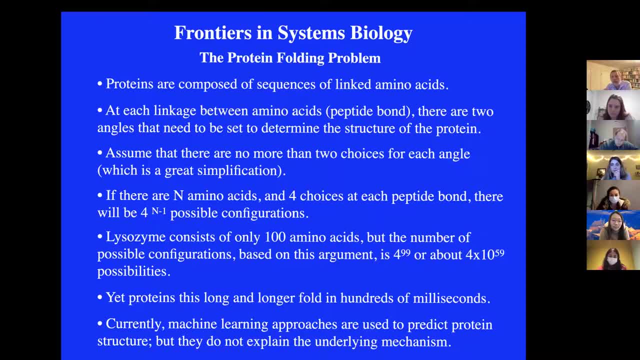 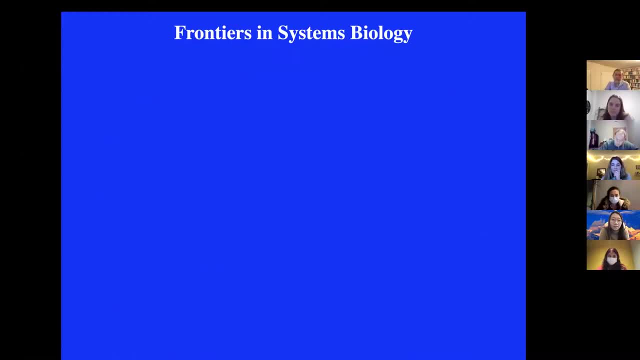 but basically it's going to fold like this And the predictions are pretty good, but it doesn't say anything about the underlying. how does it actually work? So that's an open problem and still an open problem. Another example: local plasticity and global behavior. The human brain contains billions. 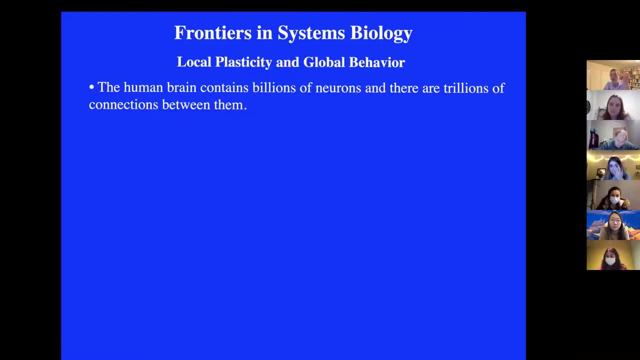 of neurons and there are trillions of connections between them. This is no exaggeration. It's amazing. Now, unlike artificial neural networks, neurons form connections even before birth, while you're you know a fetus in the in the uterus. And that's all due to spontaneous activity. The 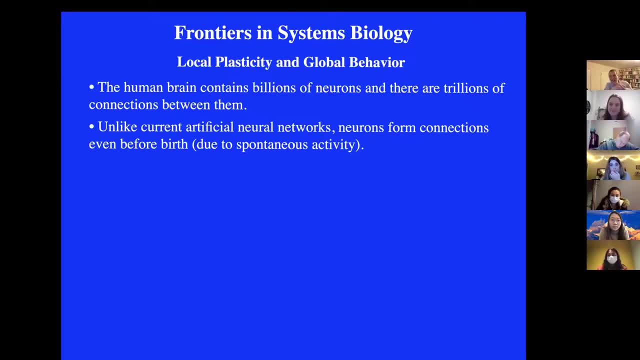 infant mom gets all this kicking because those are spontaneous motions that the embryo is generating And and if you watch the ultrasound, sometimes you'll see the the fetus is turning handsprings. All this is going on before birth. Now, after birth, within a relatively short time. 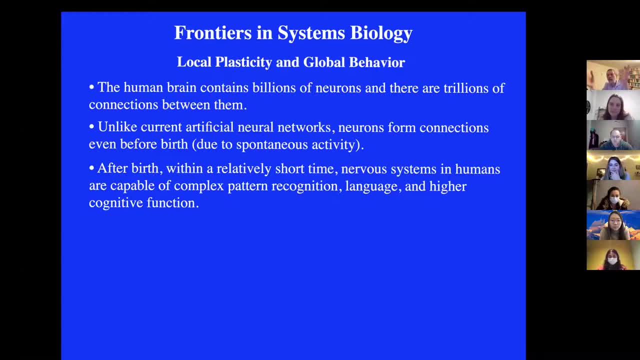 nervous systems in humans are capable of complex pattern recognition. Oh that's mommy, Oh that's daddy, Oh that's my friend. Oh that's a doggy, Oh that's a table, That's a chair. A few 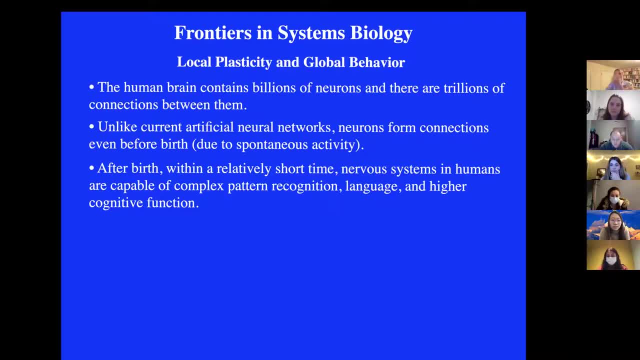 years after language And then a few years beyond that higher cognitive function. So somehow you're taking these billions of neurons and trillions of connections and you are setting them up in such a way that you can do all these things And we take it for granted, but it's actually. 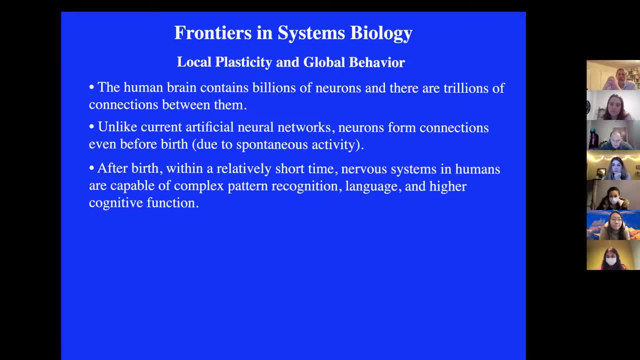 astonishing, And again in terms of the computational complexity problem, again very, very hard problem, And the amount of data that's needed to train a biological nervous system is far smaller than what is needed for current artificial neural networks. and the system incorporates new information, makes projections about the future, None of which are current. 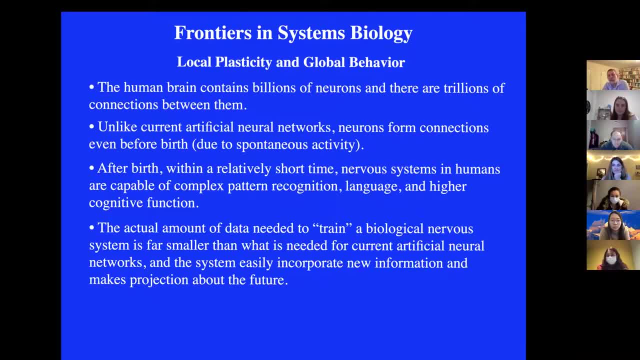 artificial neural networks do well or at all, depending on how they're designed And the number of training trials generally is huge. And then generalization and taking them. sometimes you have to just start from scratch and retrain them, because if you try to add in stuff 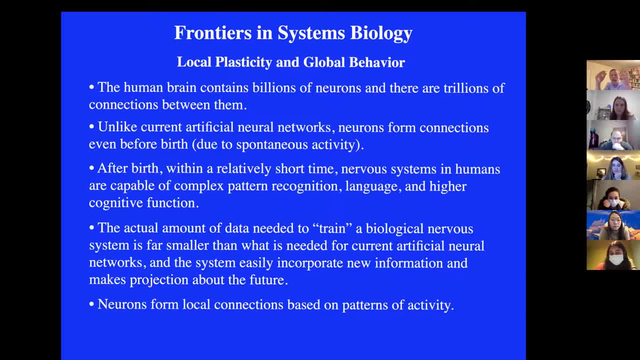 they lose other things. Now we know that neurons form local connections based on patterns of activity, And the big question is: how does local plasticity, changes in uh connections between neurons give rise to coherent global behavior? Once again, that's a Nobel prize: easy for you to grasp and take home. uh. another visit to Stockholm for you. 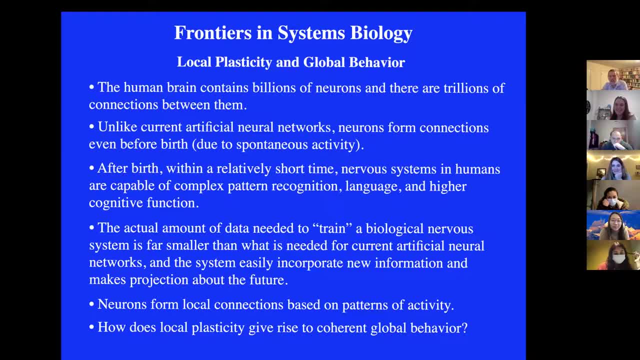 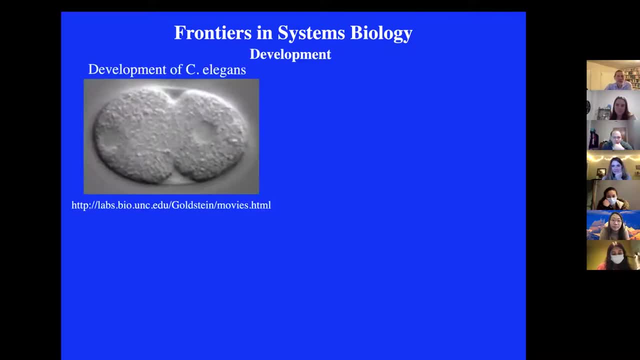 after you've taken care of the protein folding problem, This is the next thing you can solve, All right. And then the last thing I'll talk about very briefly is development, which I think is also an incredible frontier. So there's a movie that you can look up and shows the 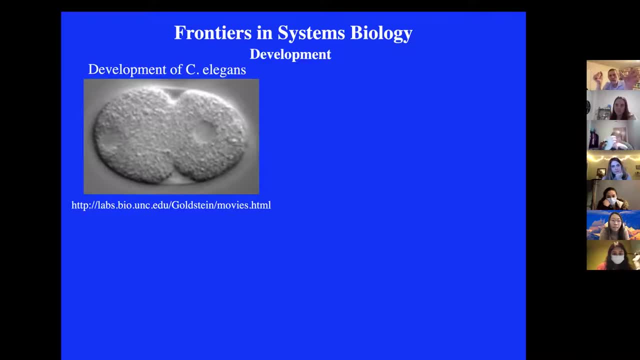 development of C elegans. This is the uh, the single cell that's been fertilized, which has split in two. And if you watch the movie- I don't, we don't have time- You'll see it becomes about 600 cells And as you're watching you'll see there's a cleavage plane. 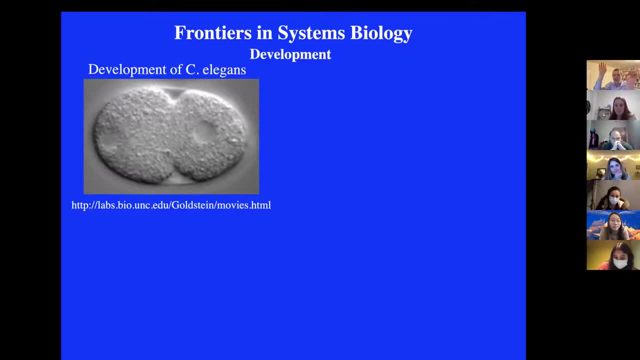 and then it starts moving around inside the egg and then it just swims away. Okay, Within a matter of few hours. So you have a fertilized egg that divides repeatedly. Each cell contains a complete description of the organism. They each have DNA, but depending on 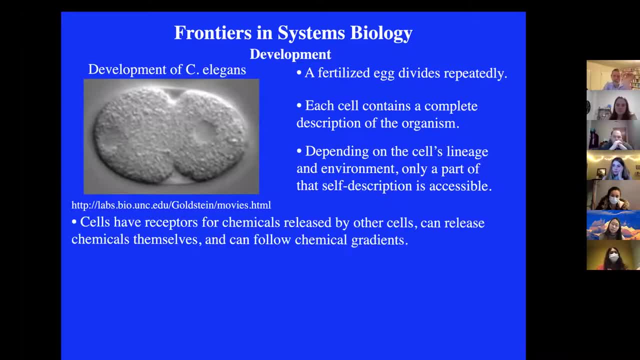 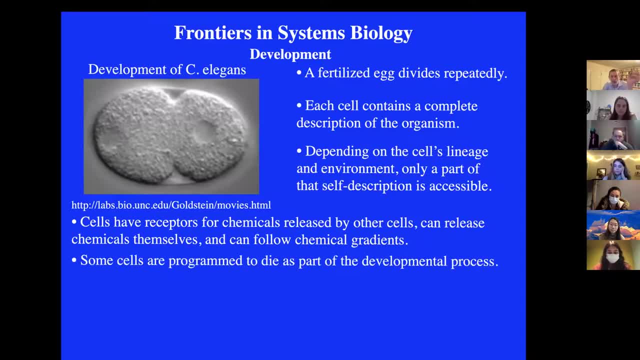 released by other cells and can release chemicals themselves and can follow chemical gradients. Some cells are programmed to die as part of the developmental process. I've just given you all the information for how cells can translocate. Cells can actually form assemblages. Some can. 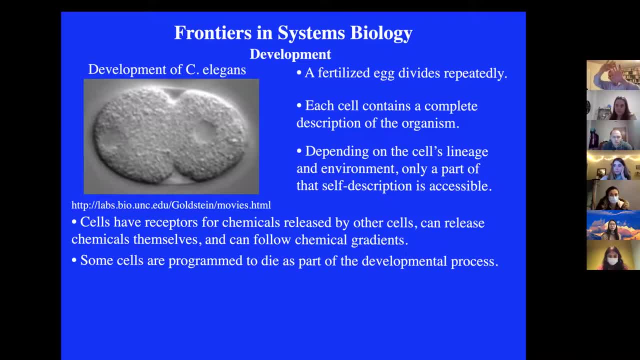 die away And that, for example, if you start with webs, you ended up with fingers, And so you have morphology And, once in final position, a cell may assume a final identity, such as a nerve cell, And you have an exponentially increasing set of cells in polynomial time. So notice, there's a theme here. 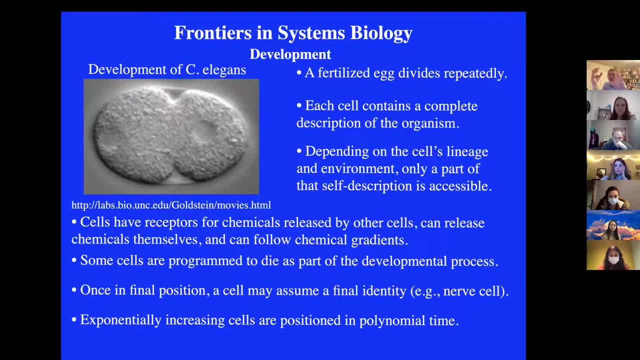 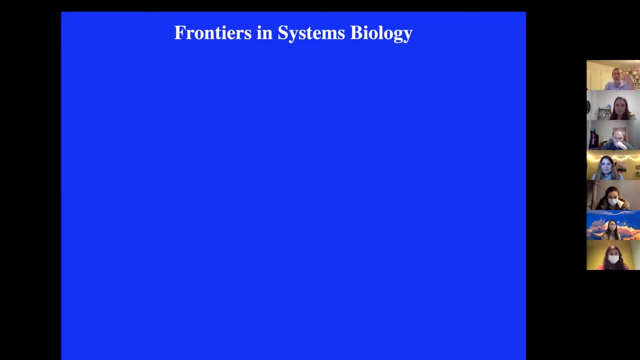 of dealing with huge numbers of possibilities and narrowing them down very quickly to what's relevant and what's useful, And the process varies, so even identical twins can differ at the cellular level. So I've talked about protein folding, local plasticity and global behavior and development. 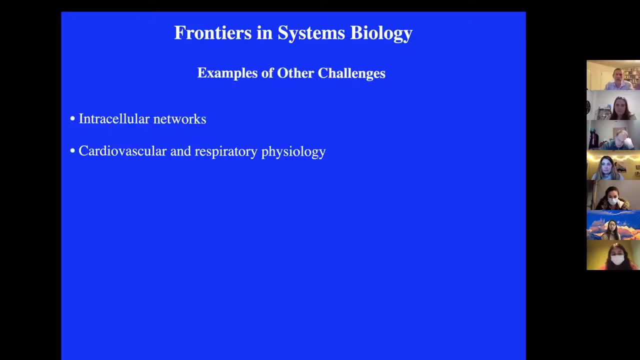 Briefly: intracellular networks, cardiovascular and respiratory physiology, helping to steer, control the immune network, ecological networks in response to perturbation and, finally, evolution and climate change. these are open areas. any person who has a systems biology background, who chooses. 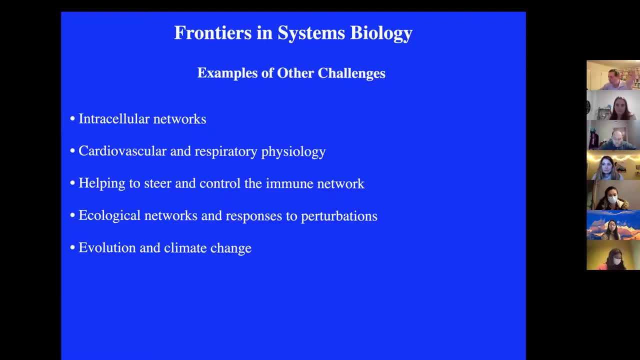 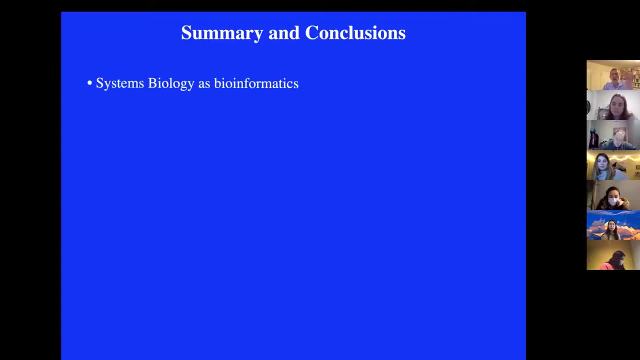 could spend an entire career studying these very exciting and important questions. So let me just summarize and then I'm done and I can take any questions you may have. So I've explained the idea of systems biology as bioinformatics. I think of that as a much more static way of thinking about. 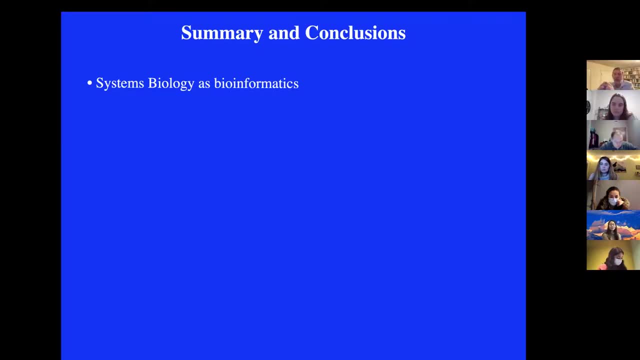 um and of categories, categorizing and looking at static snapshots, but it's very powerful and very valuable. what it gets me much more excited systems biology is biodynamics, and there you have to actually be comfortable creating dynamic models, a couple differential equation models, agent-based models, models that change and develop patterns over time, just like biology does. i've emphasized 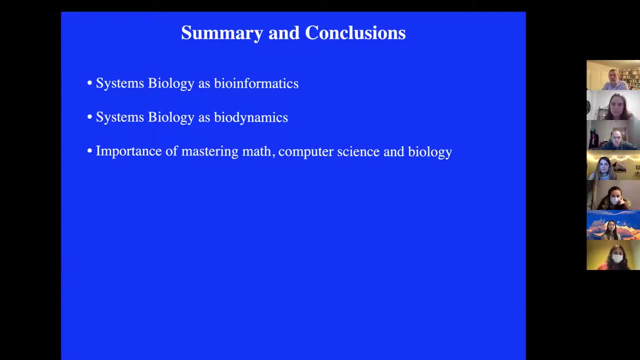 and i can't emphasize this enough- math, computer science have to be mastered along with biology. that's critical to becoming a successful systems biologist. it's hard enough to master biology, so this is a total order, but if you can do it, as i said, it makes you really unique, very special and 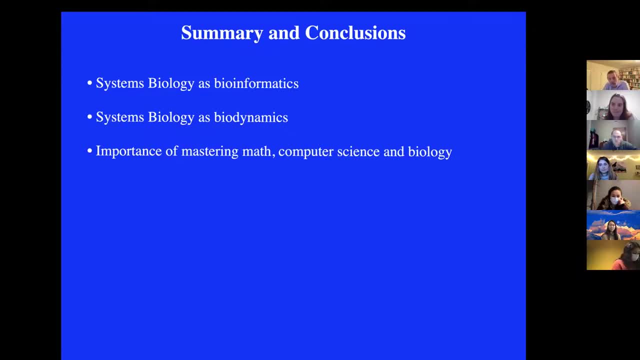 gives you a powerful access to jobs that either math and computer science students or biology students alone can't get. i've given you an example in some detail of how you iteratively model a neuromechanical system, and i drew the lesson that the methodology for this is demand driven complexity. models are not. 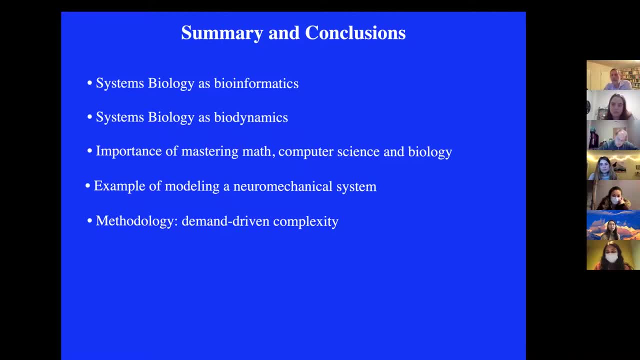 you're not going for a perfect model. you're going for a good enough model that gives you a lot of insight, tells you where you don't understand, helps you iterate by directing the experimental work, and then the experimental work is reincorporated into the next version of the model and the process. 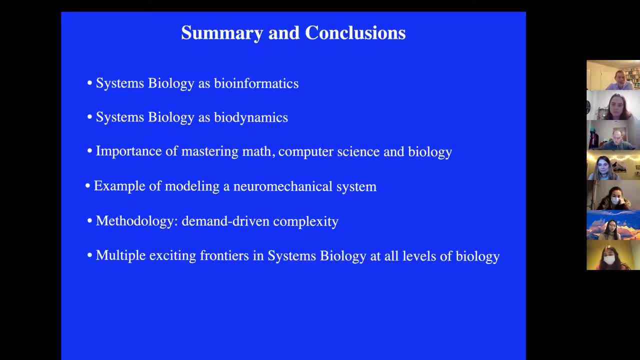 repeats. and finally, i've shown you that there are multiple exciting frontiers in systems biology, at all levels of biology, and i commend the future to you. it is in your hands. with that, i i thank you for your attention and i'm happy to take any questions. 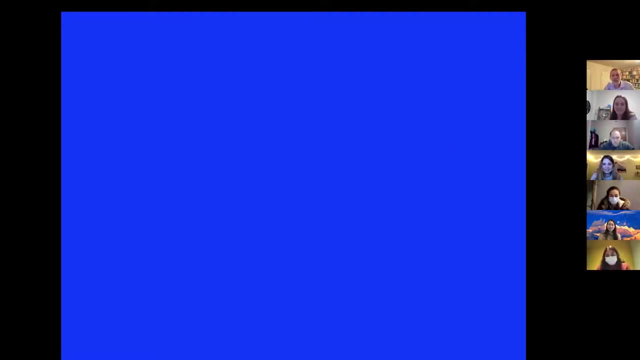 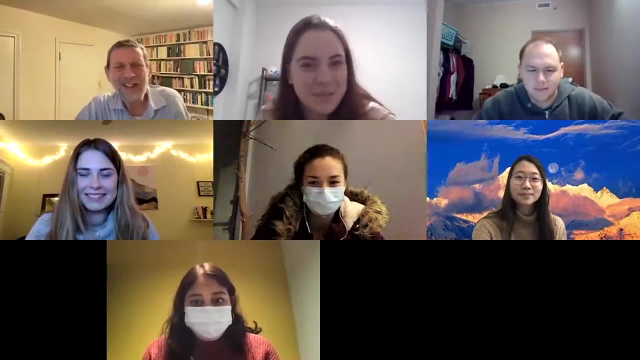 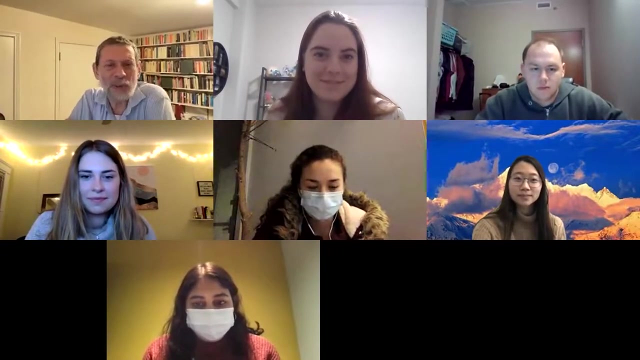 you might have. so i'm going to stop sharing. um, i can somehow mine. oops, are you? are you all? yeah, there, okay, thank you so much. that was a wonderful talk, very interesting. does anyone have any questions? yeah, i'm, i'm open for questions and i don't have to rush away, so i guess i can go um. 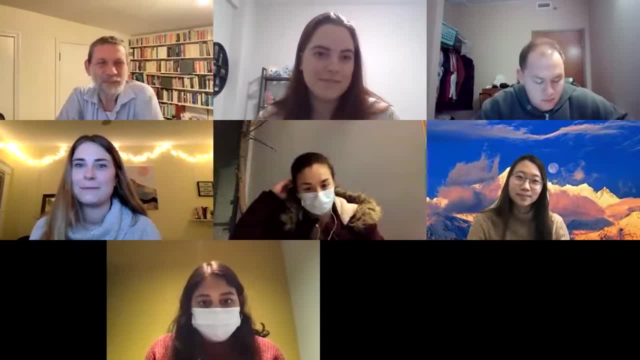 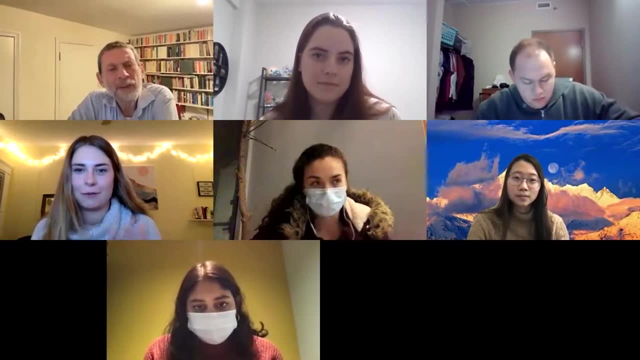 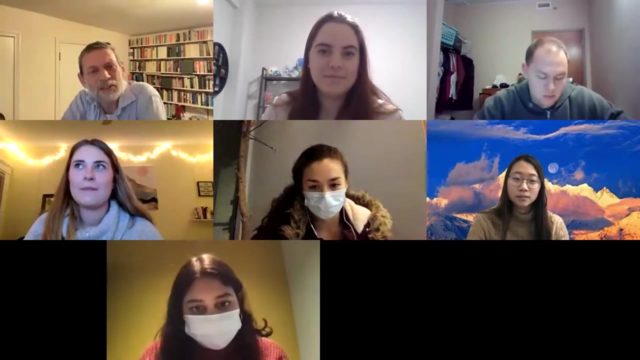 thank you again for your time. um, my question is more to do with, um, like the systems, biology, major and classes and things like that. um, so people have more like sciencey questions. they can also jump in first if they want, sure? i, i guess. um, i i'm really glad that i listened to this talk because it's made a lot more sense. 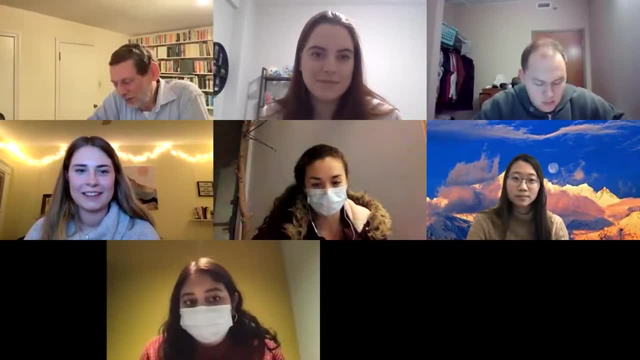 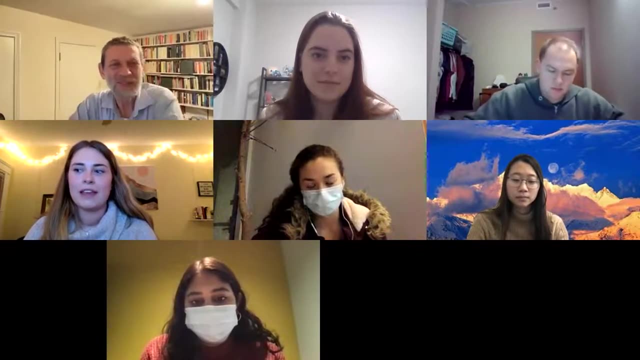 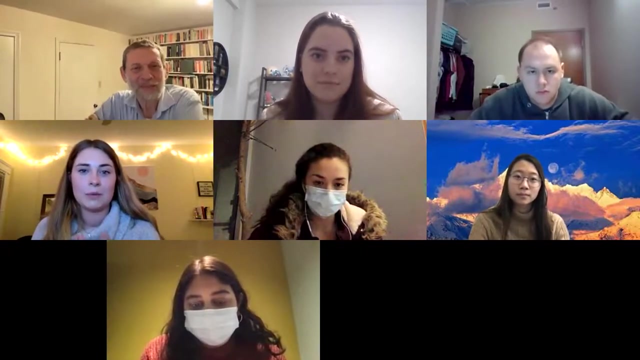 like the path that we go through, uh, in order to complete the major um with all of the goals you had in mind, but i guess, like the final thing, that i was wondering if you could talk about um, the. the final thing was: um. i think a lot of us have very different like plans for, like post graduation and 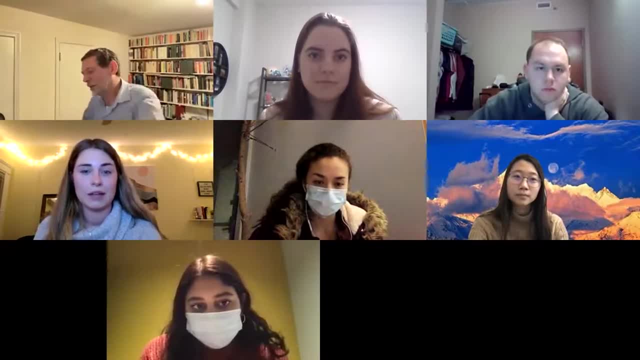 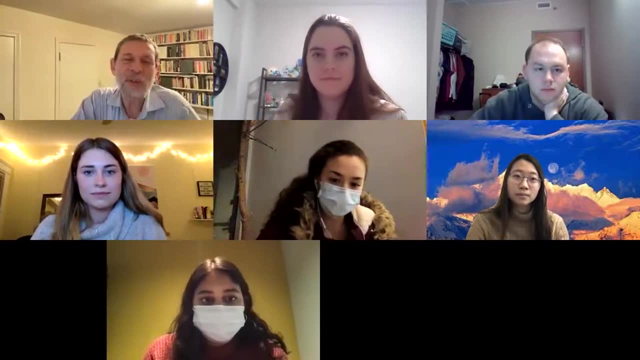 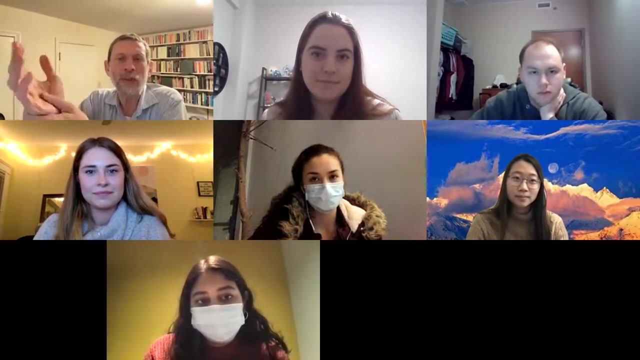 things like that. but when you were conceptualizing the major, what was um your goal, like professionally, for one of us to be able to do immediately upon graduation? that's a very good question, julian. my, my goal was to have you have as many options as possible, which is a strange answer, but it's the 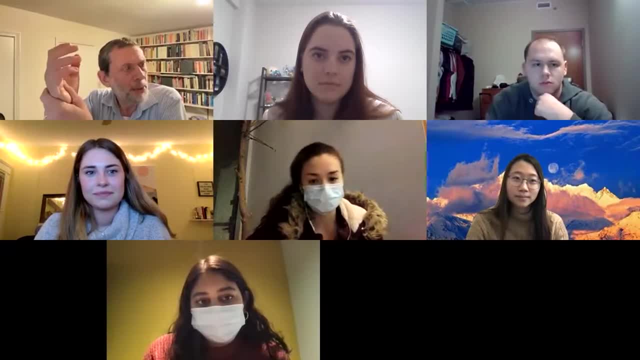 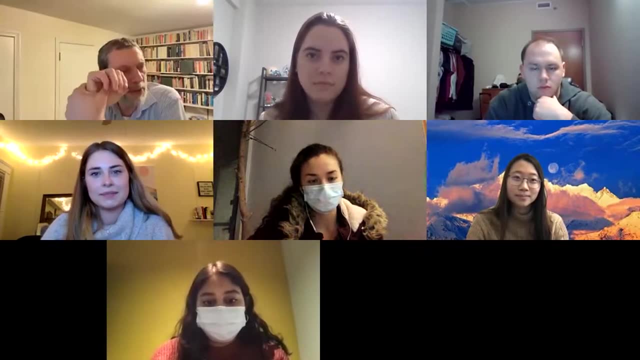 Instead of saying, oh, there's a lot of data here, you're thinking I wonder if there's a paper that has a technical model. And then you go off and you actually build something yourself, And then you come back and say: you know, I think we might have more luck with some of these anesthetization procedures if we did it this way. 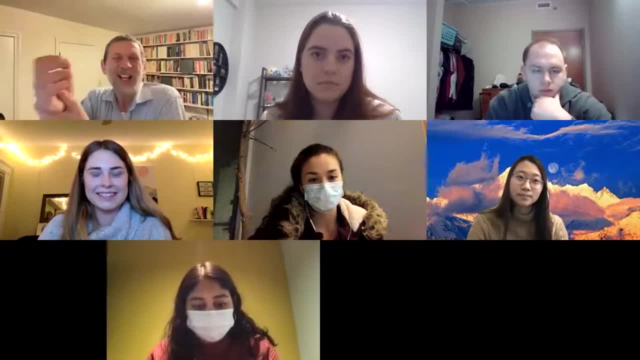 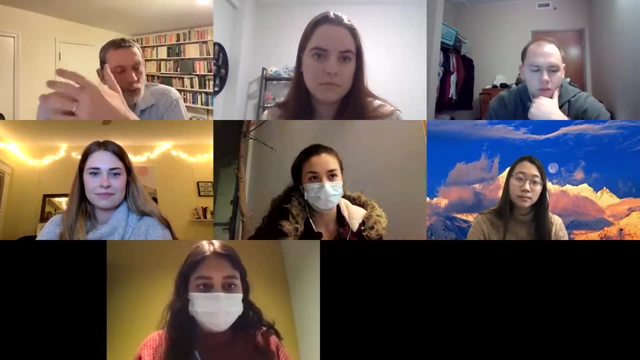 And they'll look at you like you're crazy and say, well, the model shows. And again they may shut down at that point. But if you've done it carefully and you know the literature, you can actually point out that this particular way of doing treatment allows for lighter anesthesia and better recovery and many fewer side effects. 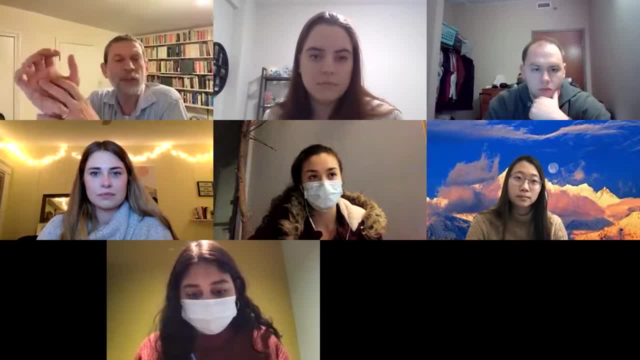 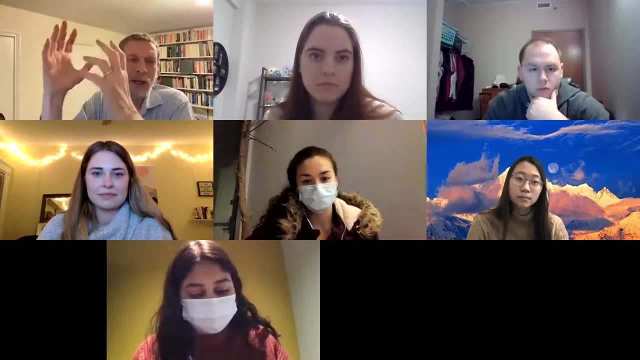 Because the data suggests that, but it's hard to see it until you put it together in a model. If you decided to work for a pharmaceutical industry and they wanted you to figure out the best antiviral, probably COVID right now, But you know they're interested in antiviral, antibacterial. 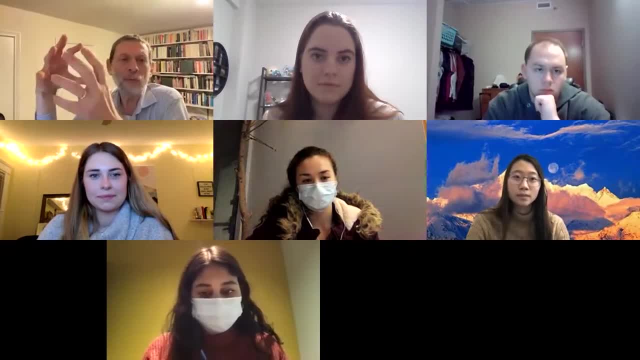 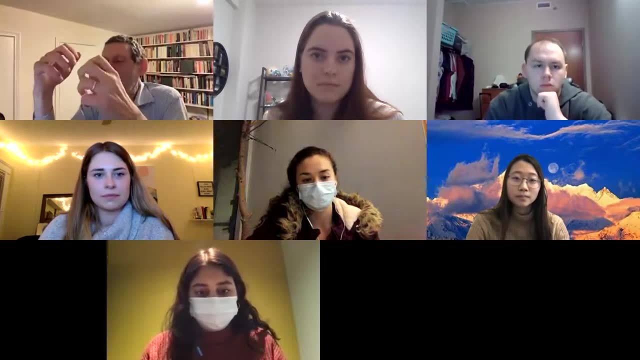 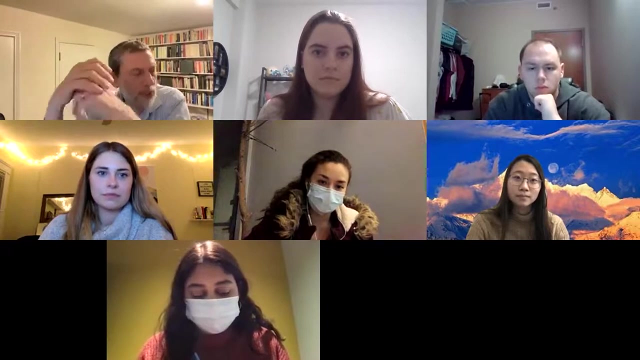 And they wanted you to be able to figure out what the appropriate epitopes were, the things that the antigens would see and would bind to and create antibodies. Then you would know how to manipulate models that would allow you to actually look at the docking sites and represent that. 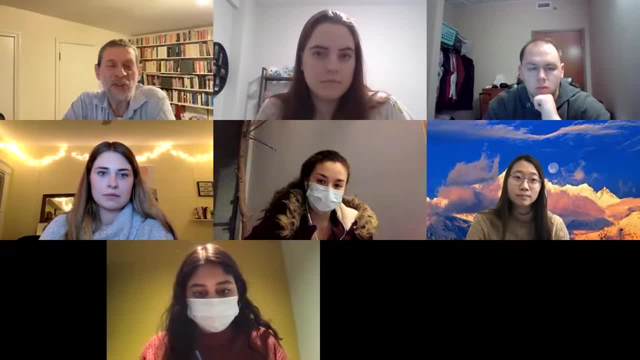 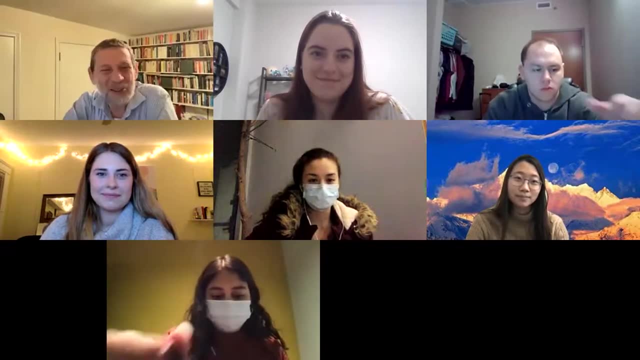 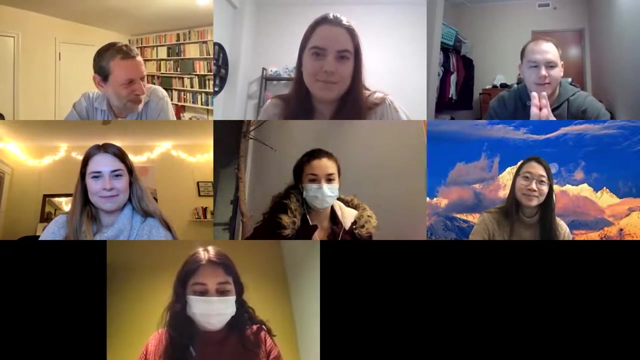 If you ended up working for the Great Lakes Commission and they were asking what level of fishing is sustainable, you might say, oh, I had a problem like that in Ohio 300.. And pull out Your old dynamics of biological systems notebooks and say, oh, that's so simplified. 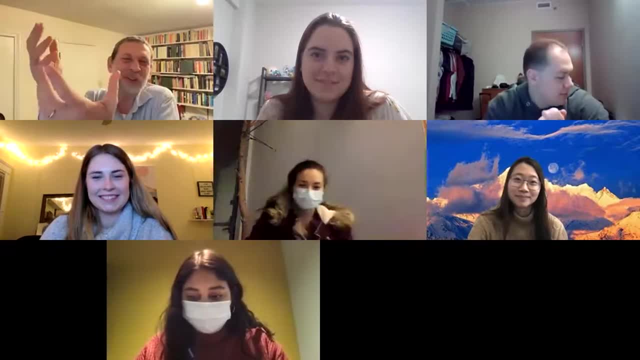 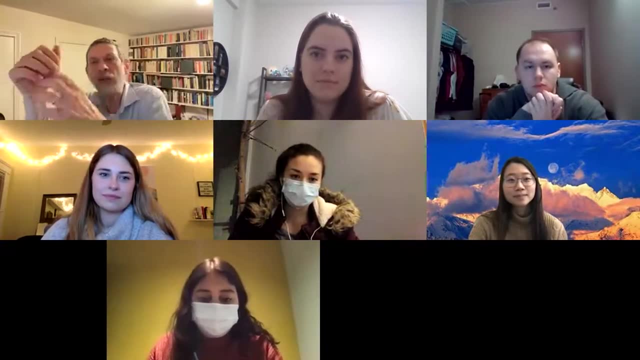 Well, that's a harvesting model, But you at least understand that there are ways in which, if you overharvest, the whole system can go extinct and you can read the more advanced literature and then come back with a quantitatively based answer. 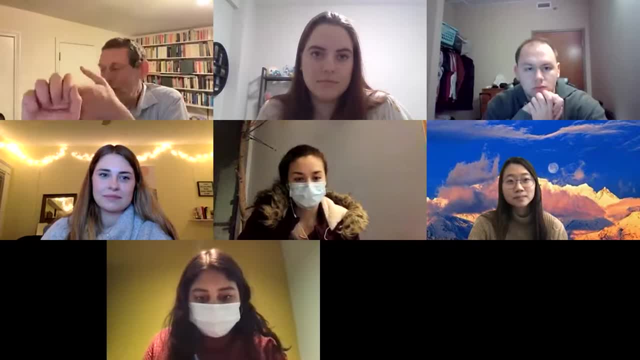 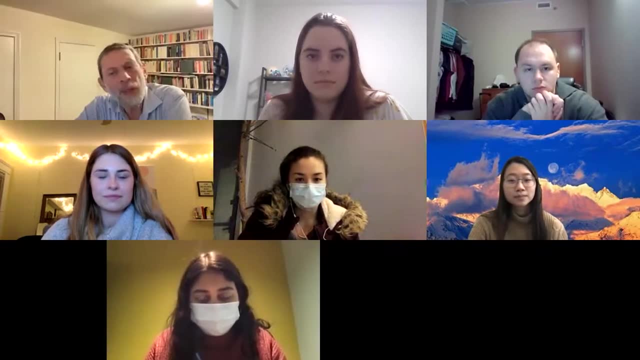 So I'm talking about government, I'm talking about business, I'm talking about industry, I'm talking about medicine, engineering, computer science, the whole gamut of things, Because by and large, we're talking about the whole gamut of things. 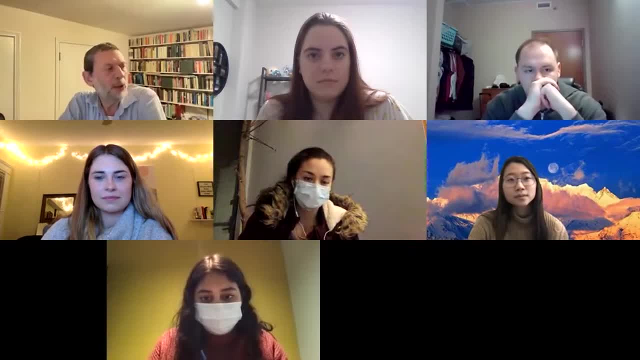 But technology is increasingly the sort of the technology that everybody is beginning to realize that if they could actually master it we could do amazing things. And if you're a systems biologist, because you have the more quantitative background, you don't sort of just know about a qualitative. 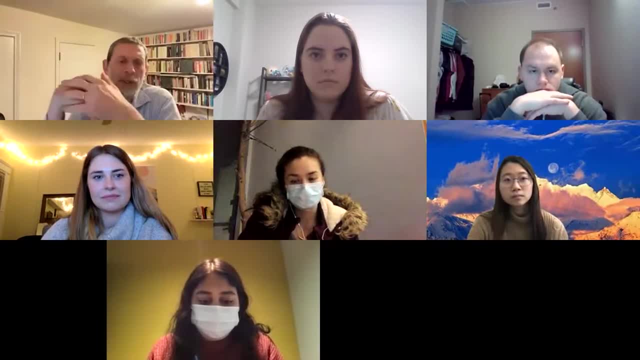 You can actually build something. You can make something that will make predictions. So that was my goal, which is very different than saying I want you to be able to get into the medical school of your choice or be good for working for big pharma. So I think if you're a systems biologist, because you have the more quantitative background, you don't sort of just know about a qualitative. But technology is increasingly the sort of the most quantitative background you don't sort of just know about a qualitative. 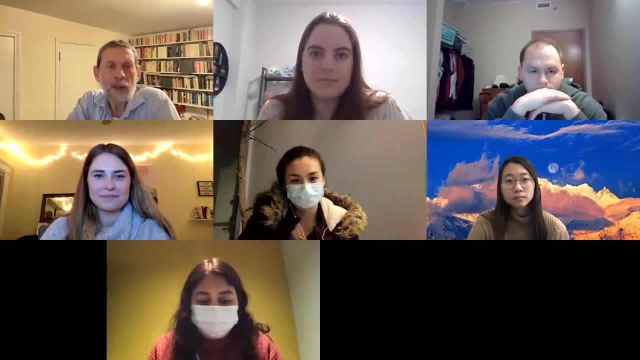 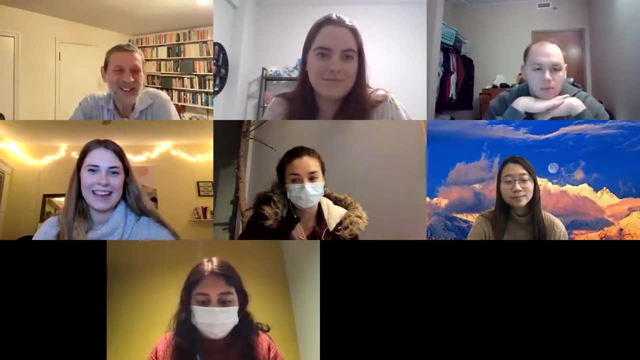 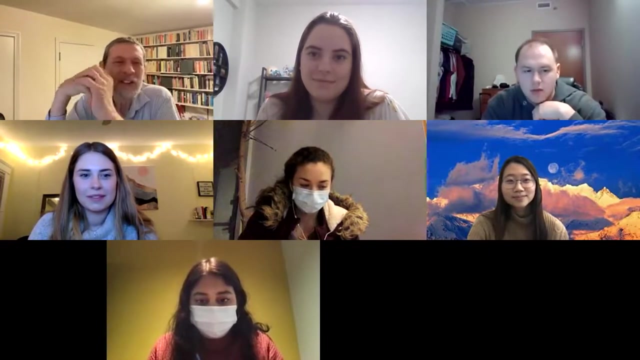 It was giving you the tools so that you could do almost anything, which I think is going to be very useful in the coming years. So I hope that helps a little bit. Thank you, Yeah, it definitely does. Other questions: I have one kind of a smaller point that you brought up in your presentation. 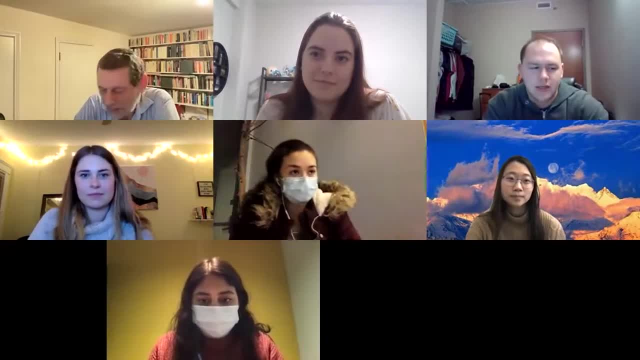 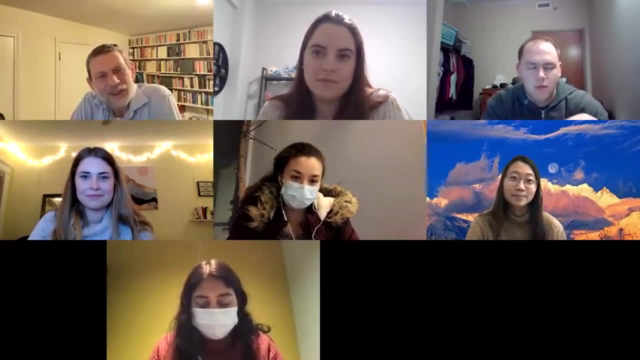 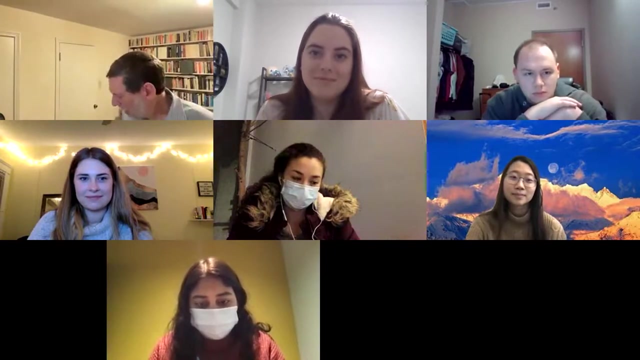 So when you were building Bio 300, I guess, like before I took it, you know ever heard of Mathematica. So it's like what made you land on Mathematica for the language that we were taught? That's a very good question, So I mentioned this at the beginning of the first. 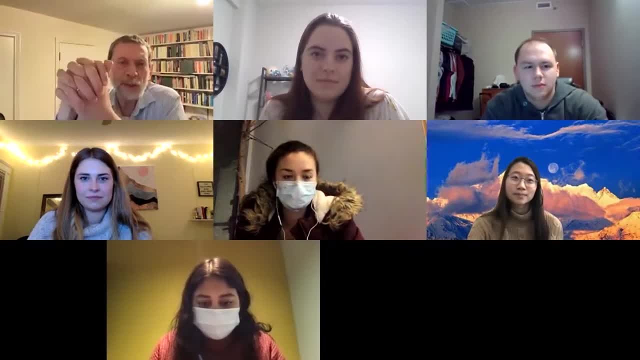 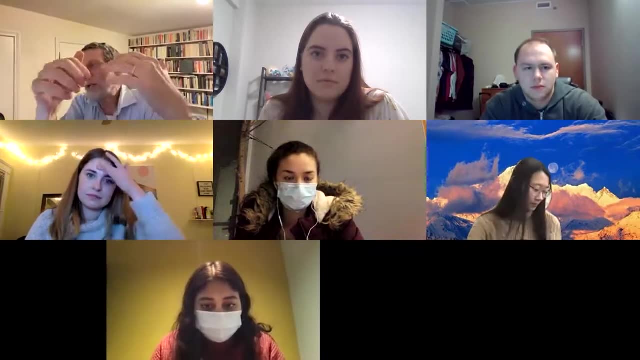 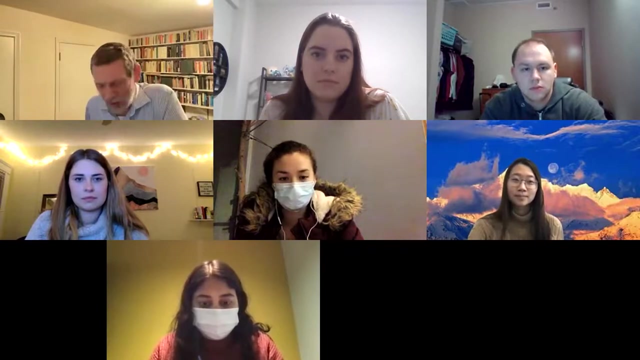 lecture. There are lots of choices. I could have had you do a programming course and done everything in C++ or Java, But the problem is a lot of that would create this barrier. A lot of biology students don't have any kind of strong background in computer science and in programming And I 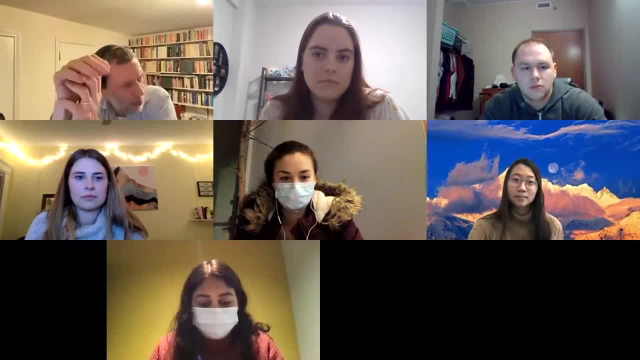 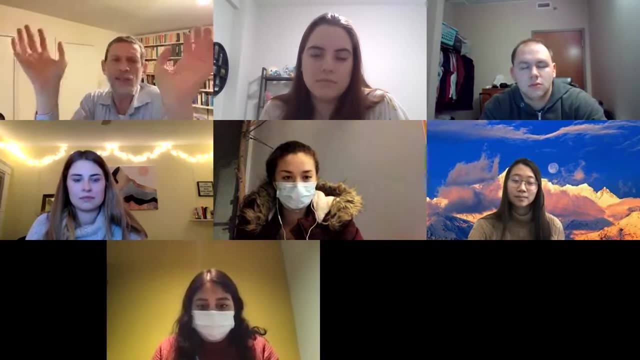 didn't want to spend hours and hours and days and days and weeks. graphical user interfaces and file systems, and where do I store data and all this kind of stuff? If you're doing C, that's not hidden from you? I mean, you have to link to the appropriate libraries and you have to compile them in, and so 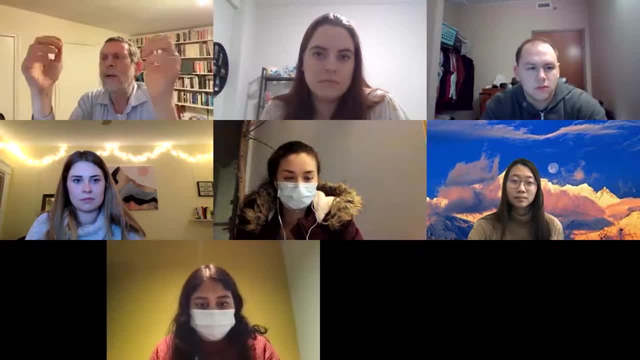 forth And that you know there are higher order things you can do in C, And there's lots that's been done in C And there's lots that's been done in C And there's lots that's been done in C. 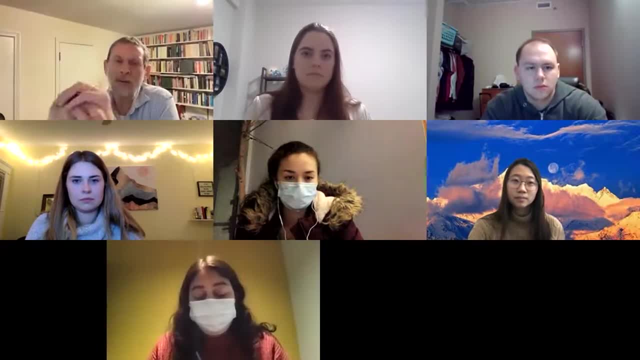 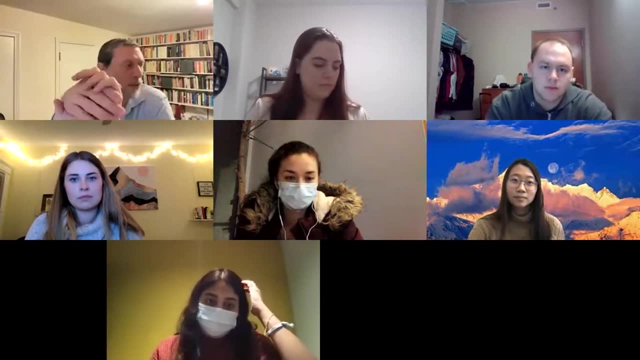 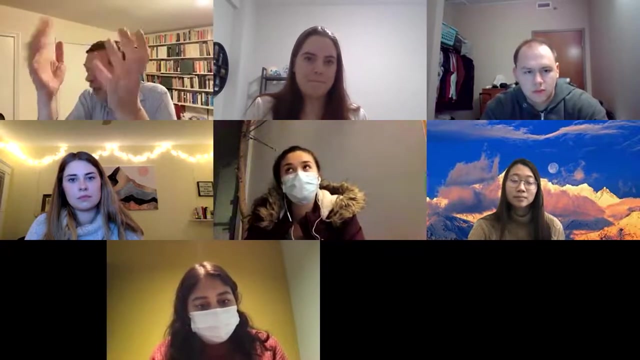 But it doesn't free you of having to deal with a lot of stuff that you don't really want students to have to worry about. If you use a specialized thing like Neuron or Amber- Neuron is for modeling nervous systems, Amber is for molecular dynamics- Then it's really great for that, but it's terrible. for other things It's just too specialized. Now, among those things that are general purpose, you have Mathematica, you have Maple, you have MATLAB- I don't know why they all start with M, but they do- And any one of those things that are general purpose. you have Mathematica, you have Maple, you. 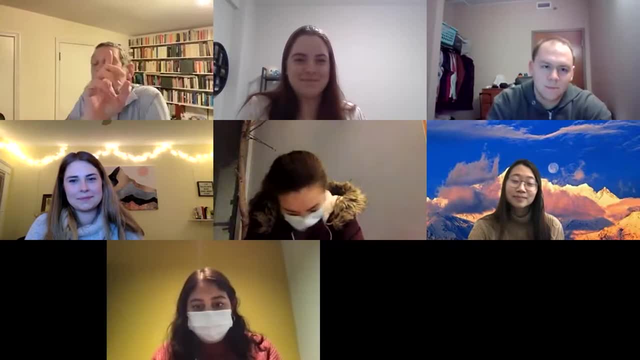 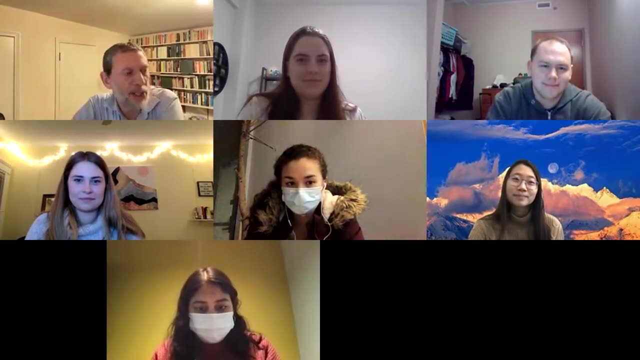 have Neuron, And any one of those, in a certain sense, is close to being equivalent. Oh, one that starts with P is Python. That would have been another one I could have considered Now if Python had been better developed and had more of the kinds of tools it does now, like the Jupyter. 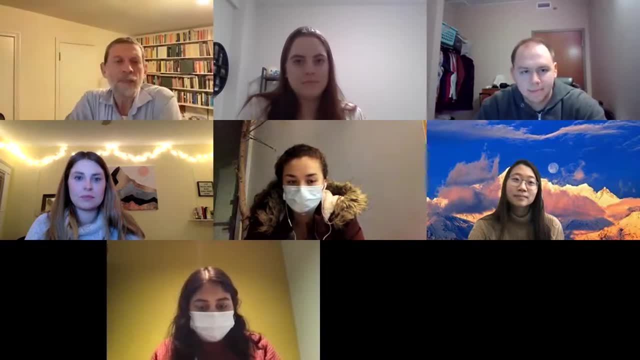 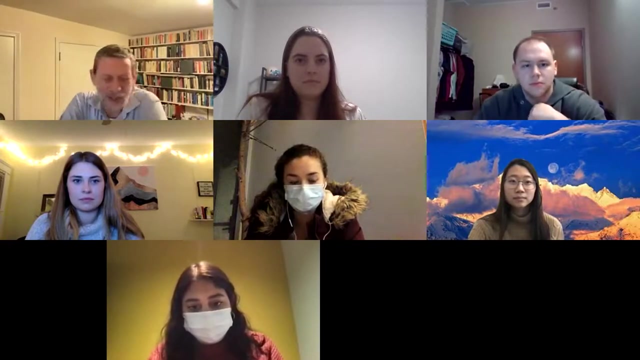 notebooks. I probably would have done it in that And I have thought about possibly switching over. But, having worked with Python and with Jupyter notebooks, there's still a lot of cruft that students are exposed to and have to deal with that. for someone who doesn't have the kind of 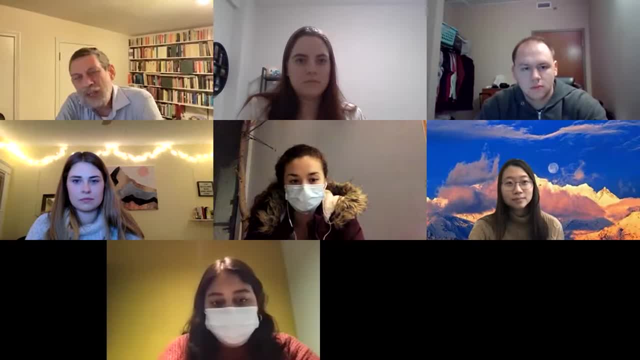 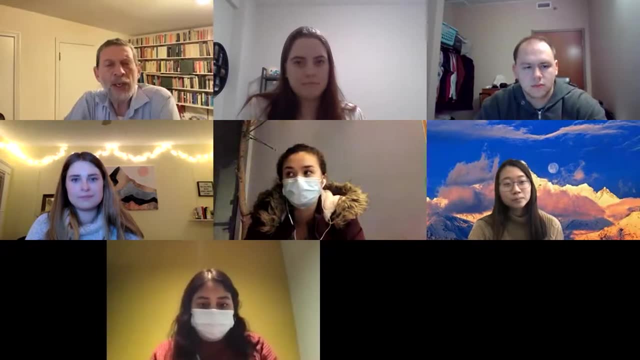 background. So the problem that makes that easy would make it very, very off-putting. And they get you know a few of the error messages and they simply shut down In Mathematica the built-in functions and some of the 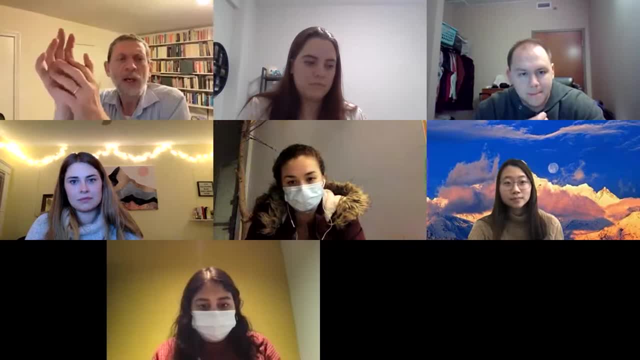 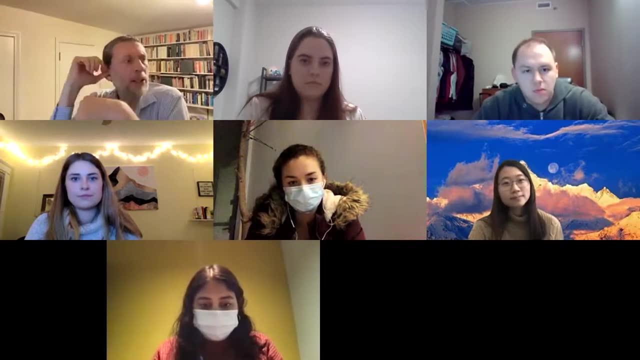 simple things that are easy to invoke, allow you to do very, very powerful things with very few lines And you get immediate feedback. And the other thing that, for me, sold me on Mathematica was two really very powerful things. One is that you can do word processing, So I could write my entire textbook in Mathematica. 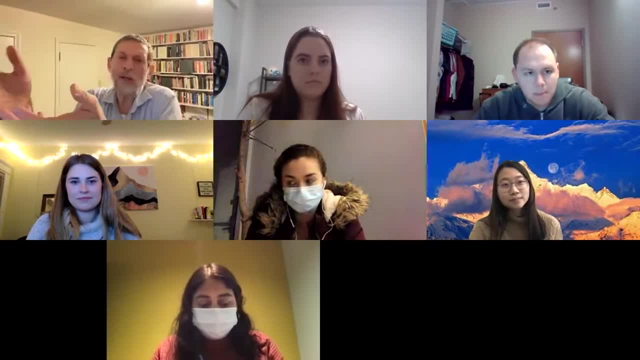 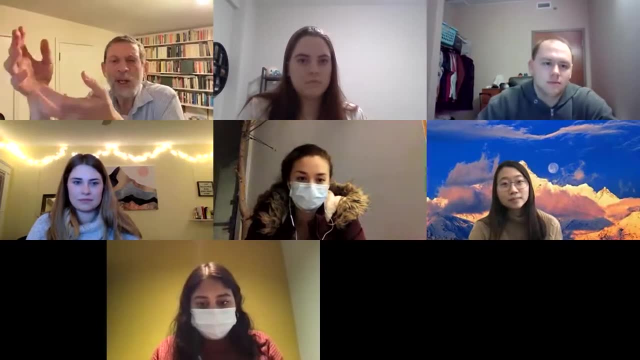 and then I could hand it to you, And so you could just take code from the textbook. Think about other textbooks. you've had right. Even if they provide you MATLAB code, unless they put it in some other form you have to type that in again. Now they might hand you files, but here you could. 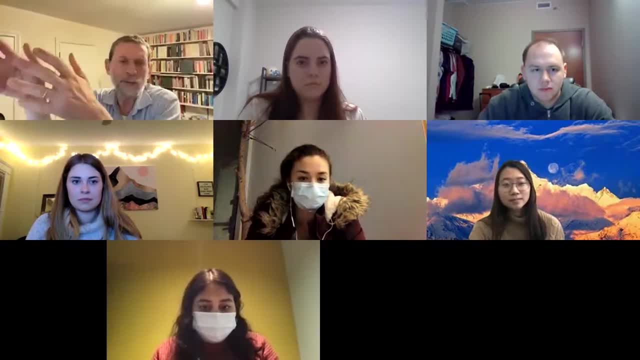 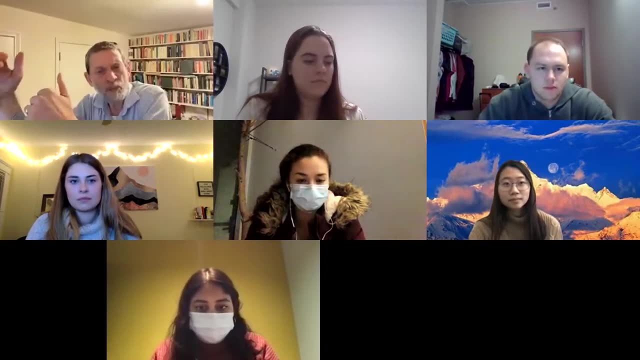 go to one of my figures, pick up the code, put it in your own notebook, activate it, get the same figure and then start tweaking it. So the overhead to actually presenting very complicated stuff is much lower And you could read and go back to the text and see how that. 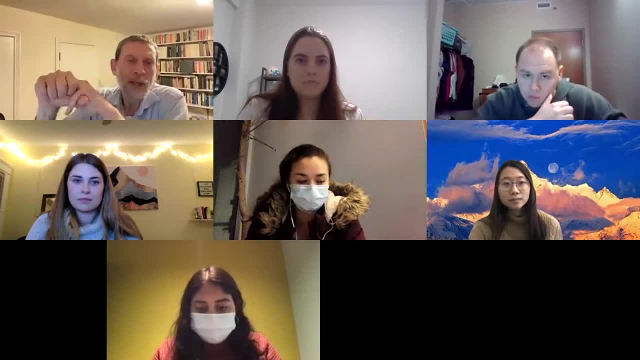 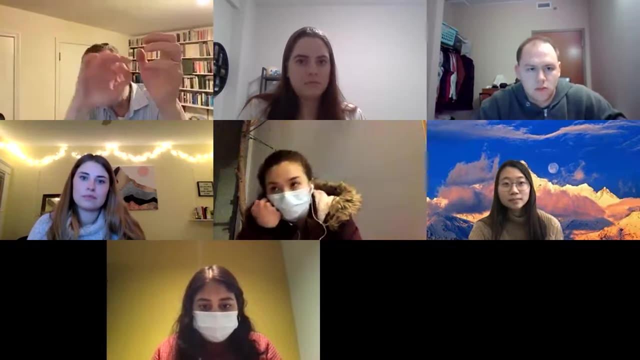 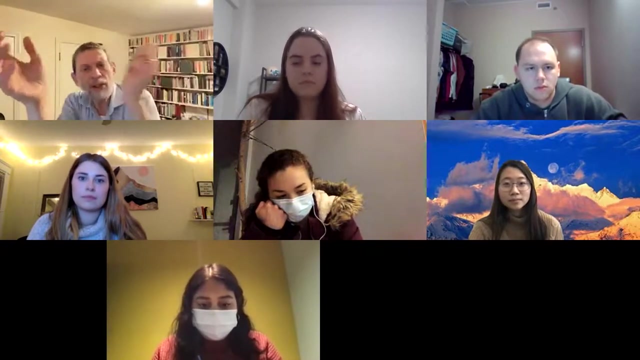 integrated. The second thing that was really powerful was manipulate, Because there you could take a model and then you could dynamically alter it by moving sliders or clicking buttons and see the model change right in front of you instantly. So suddenly, and this is a very important thing- you can see the model change right in front of you instantly. 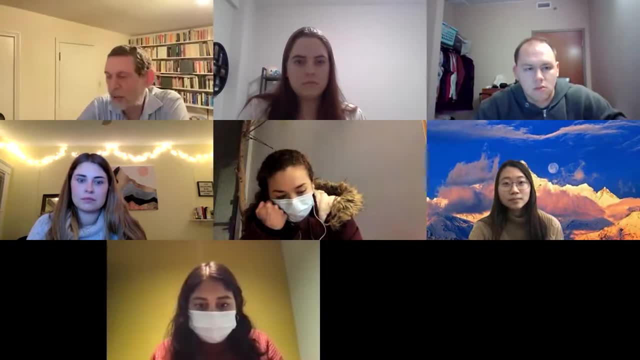 So suddenly- and this is a very important thing- you can see the model change right in front of you instantly. So suddenly. for me, this is the most important thing. Biologists are actually. this is something that mathematicians, computer science and engineers often forget. Biologists are very smart people. 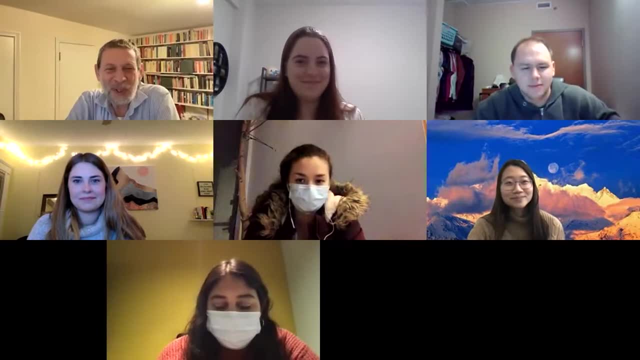 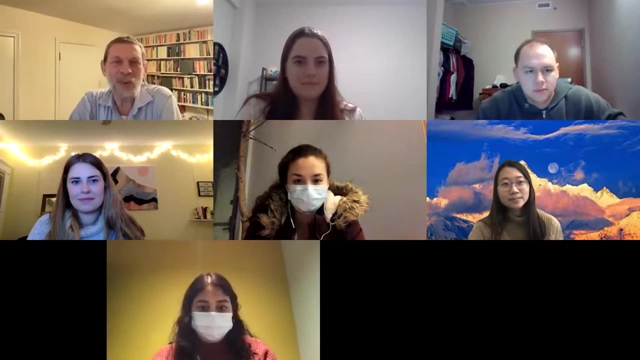 but they think differently. They are focused on seeing examples. They like actually watching dynamic processes. That's what they do. They'll spend hours staring through a microscope at a paramecium, because it's just so cool, And during that time they'll learn a lot about how. 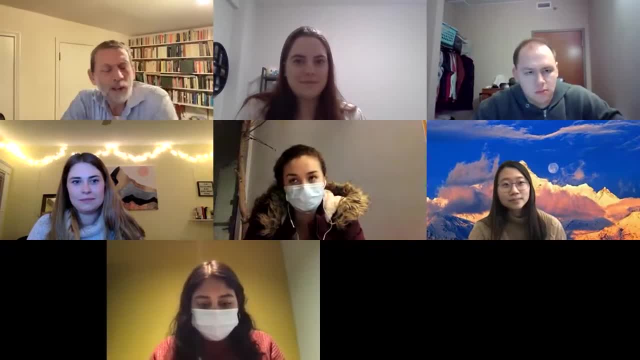 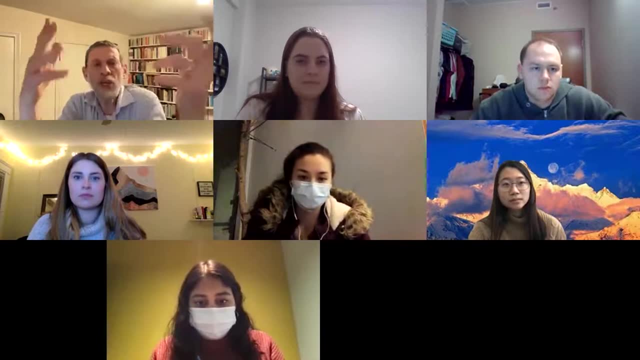 it works and have all these interesting ideas. With manipulate you can turn math into an experimental science. You can play with the model. You can then change, and then people in the second half of the semester. of course the models get too complicated, You can't do it. But if you had a three-dimensional 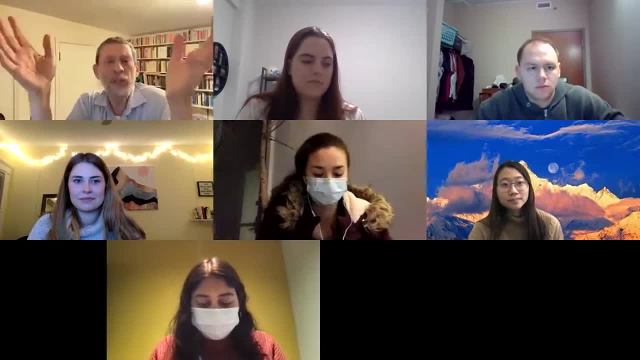 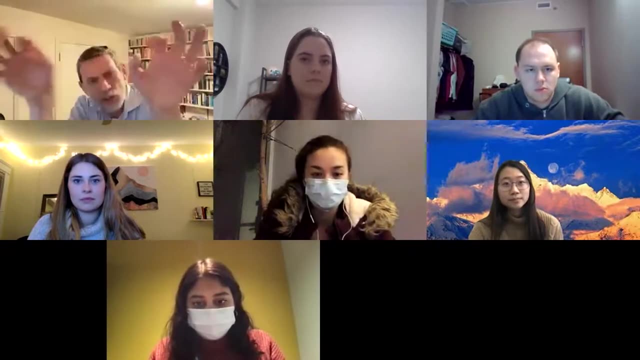 four-dimensional model and 10 parameters. you could actually set up and manipulate and learn a huge amount about equilibrium points and instability and oscillations and all sorts of stuff, just by playing. That's very hard to do in almost anything else that I know of, including. 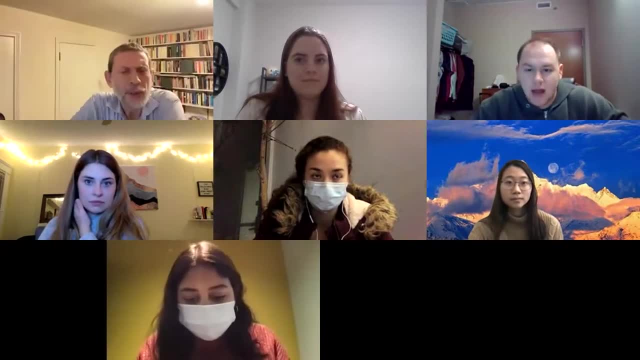 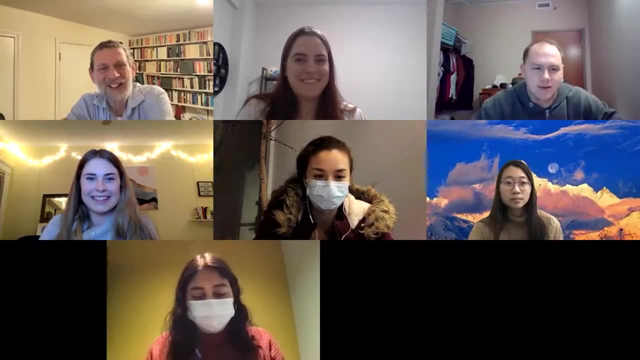 MATLAB Not impossible, but just much harder. So those are the things that, Sorry, I was just going to say. yeah, I have no clue what I'm doing in MATLAB as we stand, And that's what Right. And so the ability to put together text. 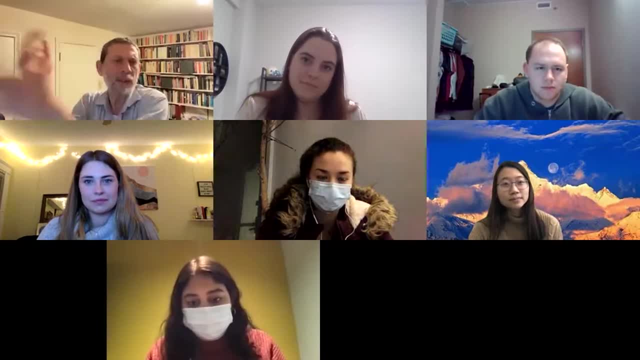 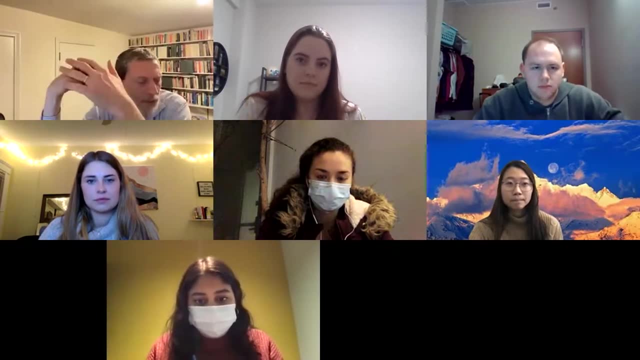 dynamic equations that the students could simply pick up and use and to be able to manipulate models. for me, that was the selling point for Mathematica And it's again, even though it's not as popular as some of the other things. 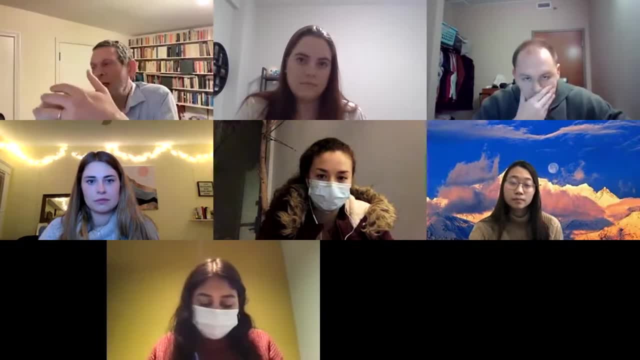 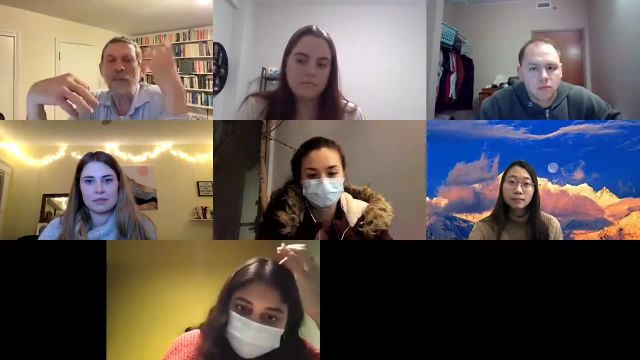 once you get the Principles- The nice thing about Mathematica: the principles are: everything's an expression and all you're doing is transforming one expression into another, which is a very mathematical way of thinking about it- very abstract, But once you get it, you can do an. incredible amount with that. The new things you're learning are the particular specific functions, some of the details, but the principles of what you're doing are the same over and over again. So it's much easier than other programming languages where you have to keep on. mastering different kinds of Things. That was why I went for Mathematica. Yeah, I was just Because when I took the class, I had used MATLAB before, and then, right after the class, I proceeded to use MATLAB to do dynamic modeling. 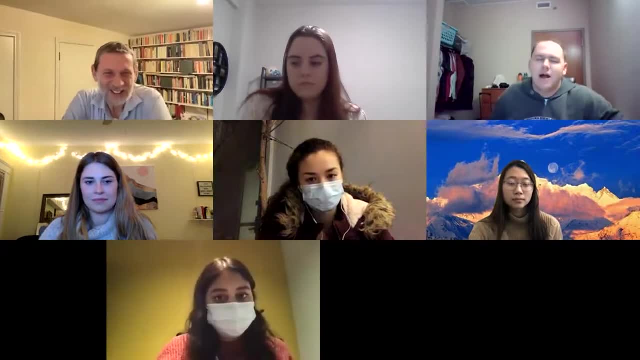 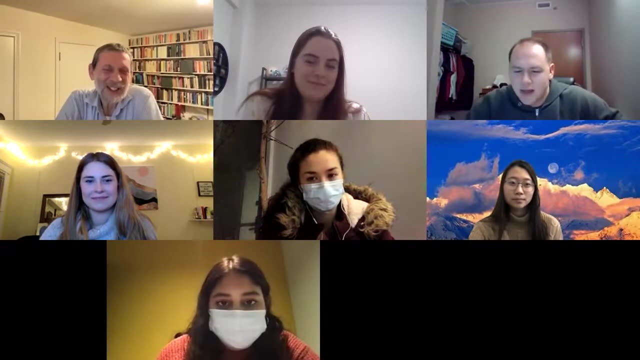 from then until now, And I knew I was trying to think There was a reason that Mathematica was chosen over MATLAB. I just couldn't think of what it was. but Yeah, Okay, those are the reasons. And again, it was easier for you to use MATLAB, having done Mathematica. 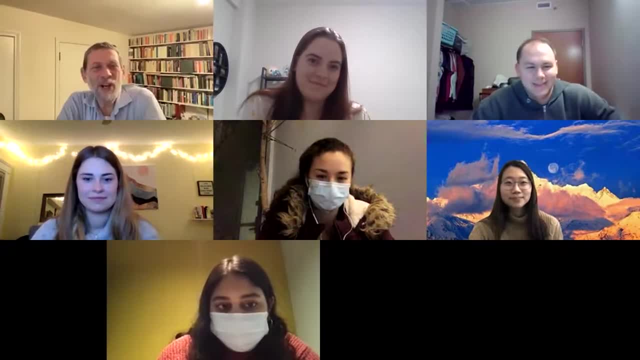 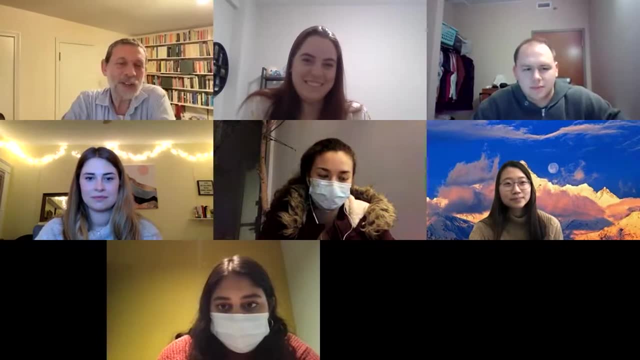 Oh, 100%. I mean ODE45 is not really the most. I mean, once you get used to it it's not bad, but it's really not the most transparent. And again, everything in MATLAB is focused on matrix. 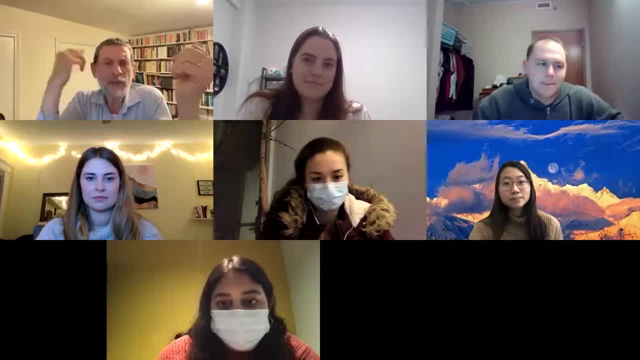 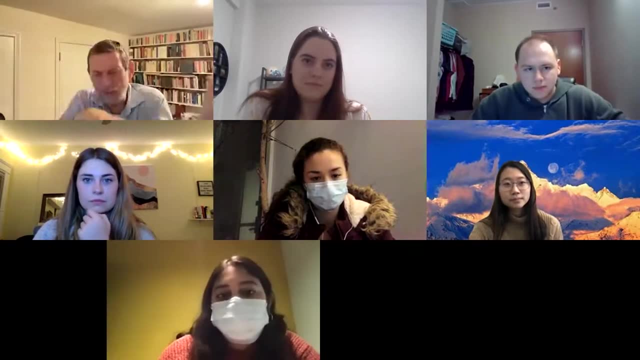 manipulations. That's really what it's about, But in Mathematica that's lists and the list transformations are very straightforward. So again, once you think of how to translate from Mathematica and MATLAB, most of the things that are going on conceptually are not very difficult. It's just 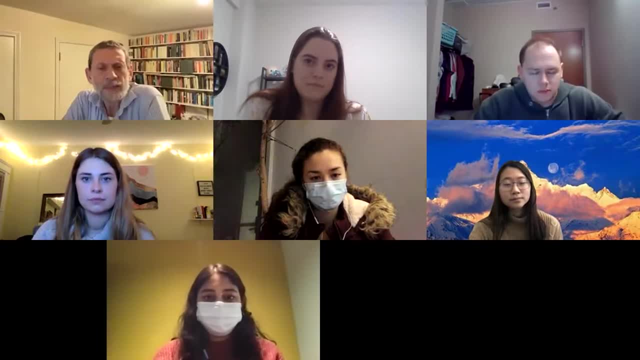 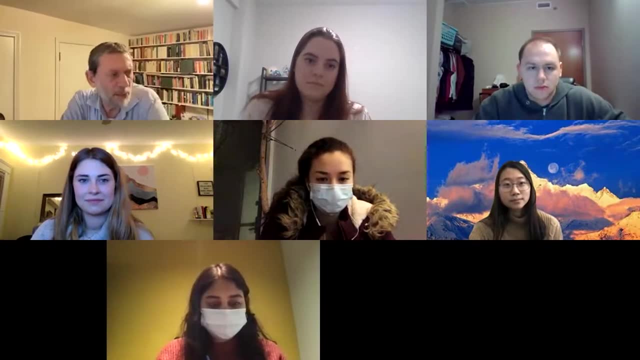 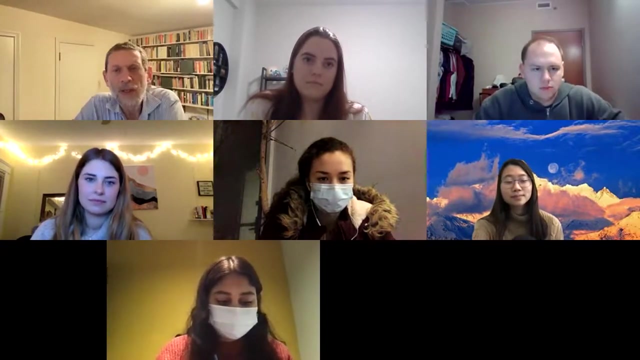 learning the syntax and things like that. So, anyhow, I like a tool that starts off and can be presented in very simple ways but is actually every bit as sophisticated and complicated as any of the very advanced tools. So all right. other questions Could you speak more about? like the 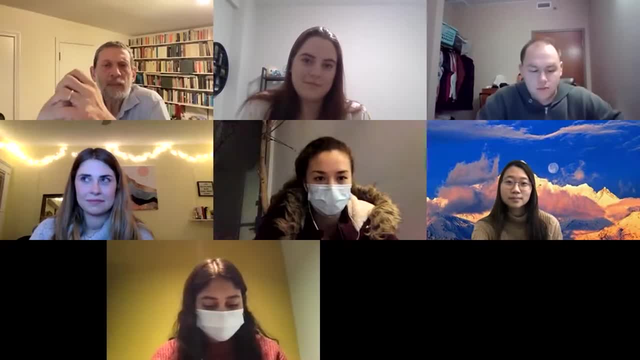 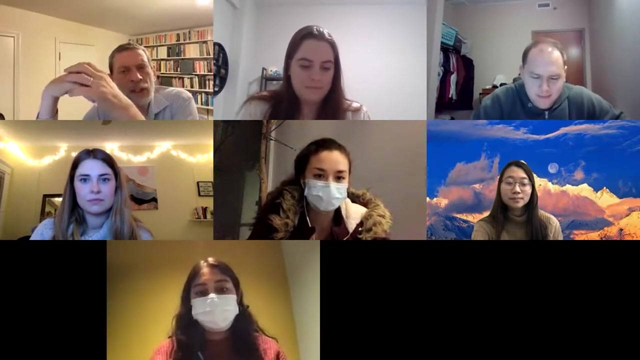 engineering and creation aspect of systems biology, Absolutely, absolutely. Let's talk a little bit about it. This is a whole area that's going to be more and more exciting. So there's a whole area that's now called synthetic biology. Have you heard of it? The basic idea is that you 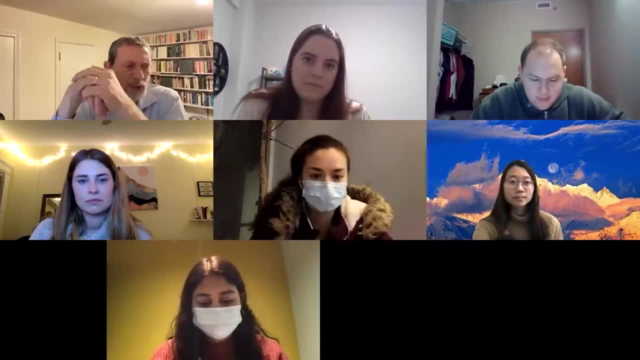 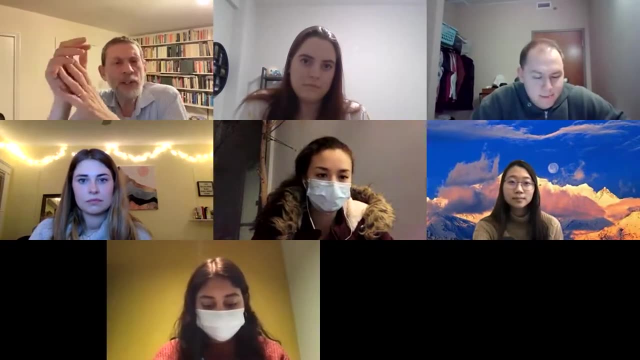 would use your understanding of how biological systems work to actually create, for example, complete artificial cell. Now that was just fantasy and science fiction. That's no longer so much fantasy and science fiction With CRISPR-Cas9, the ability to now go in and 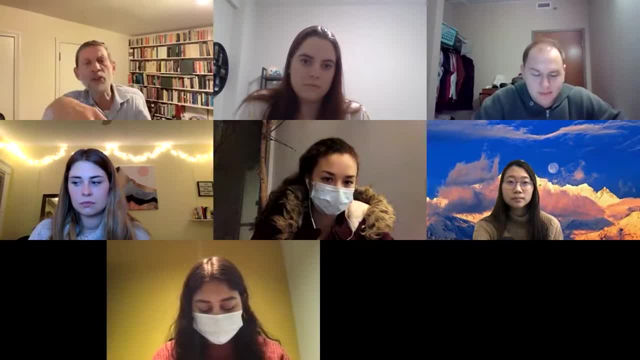 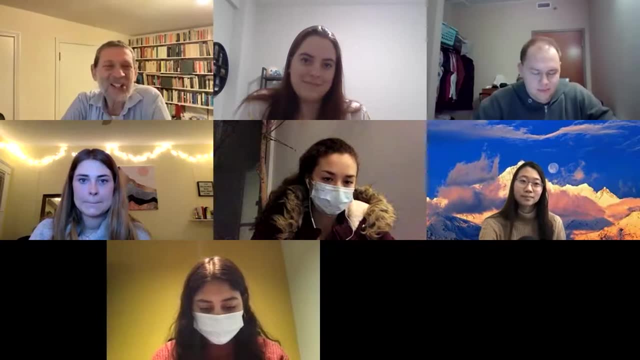 reach into an adult and change parts of the genome is incredibly powerful, But, of course, one of the things you'd like to do before you muck around too much with that, since none of those tools are perfect and they may actually change other things you might want to spend. 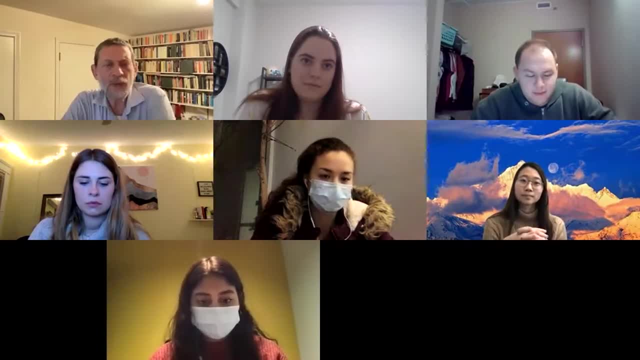 some time modeling what might happen if you do this. Similarly, if you're an epidemiologist and you're confronted with a problem, you might want to spend some time modeling what might happen if you do this. Similarly, if you're an epidemiologist and you're confronted with a problem, you might want to spend some time modeling what might happen if you do this. Similarly, if you're an epidemiologist and you're confronted with a problem, you might want to spend some time modeling what might happen if you do this. Similarly, if you're an epidemiologist and you're confronted with a 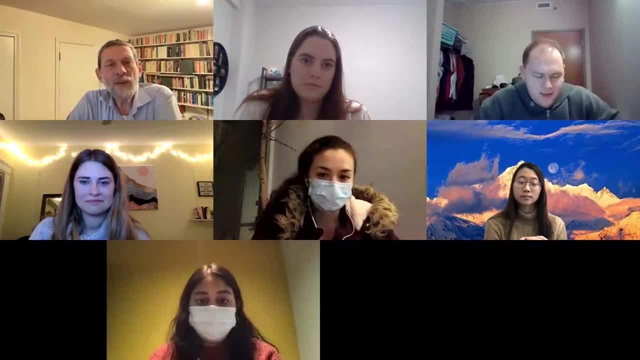 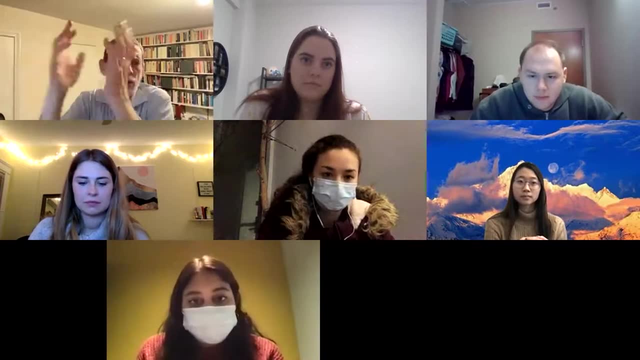 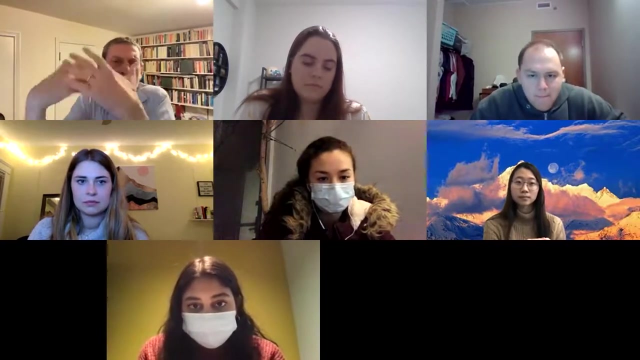 pandemic. and there's yet another new variant: if you have a set of models and tools and that you can say things about what will happen if we do X versus if we do Y, to the spread and speed, I mean not everybody's going to pay attention and do what the best advice is, but you can set up these very 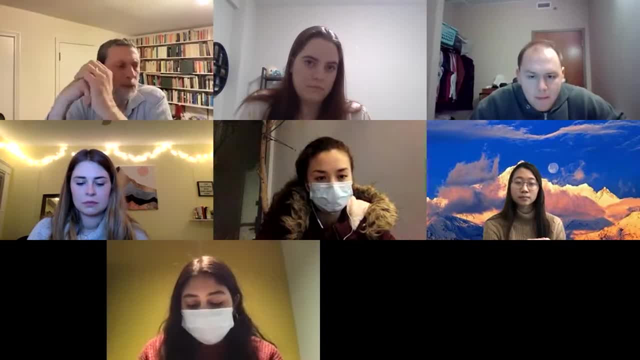 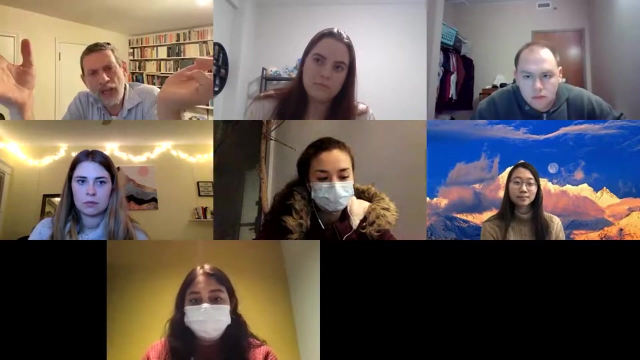 good models to talk about, how to flatten the curve so you don't overwhelm the health system, what social distancing can do for you, how to avoid super spreader events. All of these kinds of concepts are things you can build and then manipulate and use to predict aspects of. 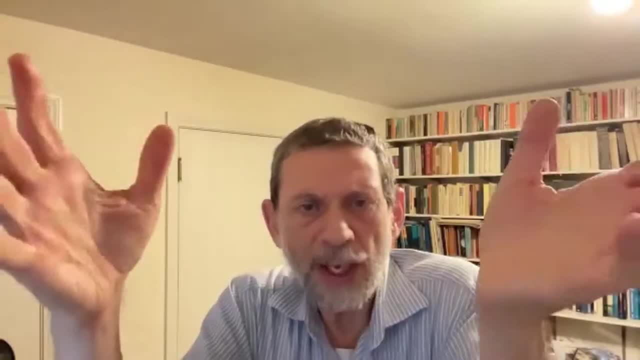 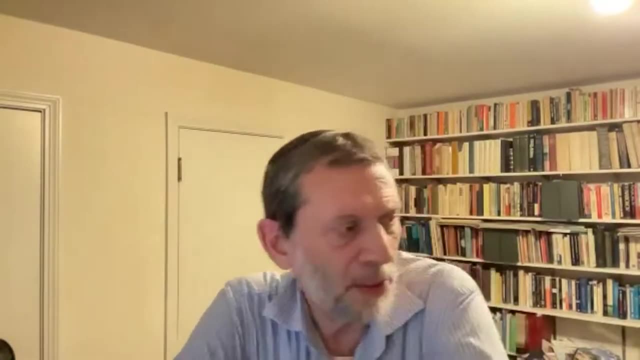 the future. So the engineering aspect. the other engineering aspect, of course, is that if you come up with a better understanding of any things I talked about protein folding, if you really understood the process well, then you could design your own proteins. Right now, people are 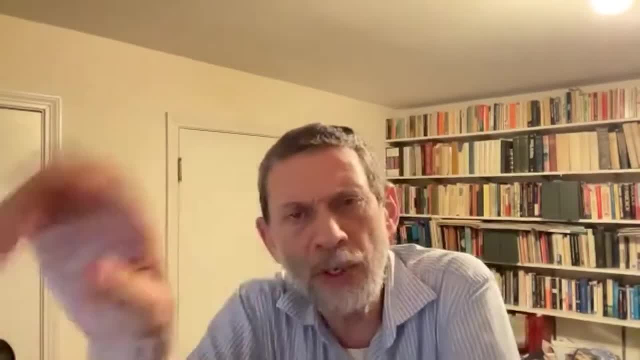 doing that. It's hit and miss And it sort of works because again you used what you've seen before: You put motifs together, but it's still somewhat hit and miss. If you could actually simplify it, you could do it. If you could simplify it, you could do it If you could. 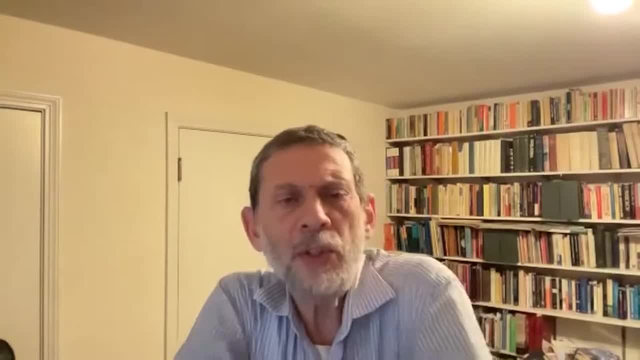 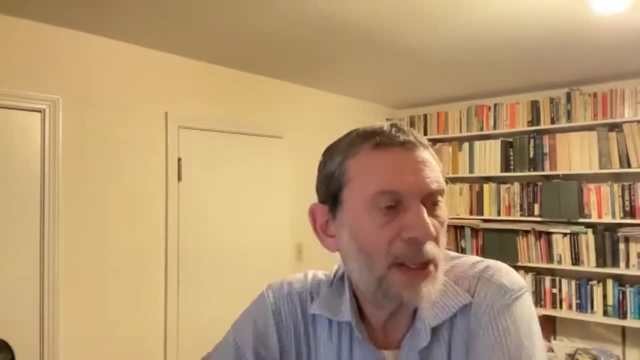 simulate what the protein is going to do when you put it in a particular sequence and describe that protein in detail. that would be very powerful. If you understood how learning actually works, then you could create far more powerful artificial neural networks than what we currently. 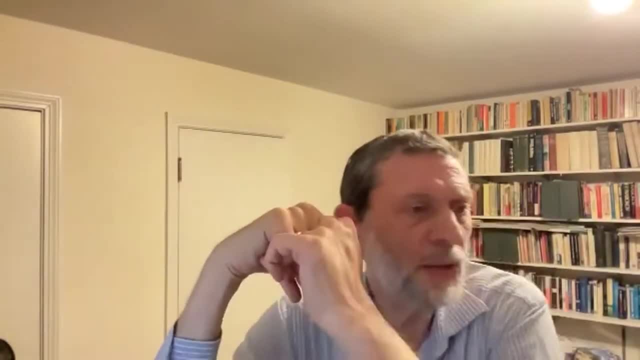 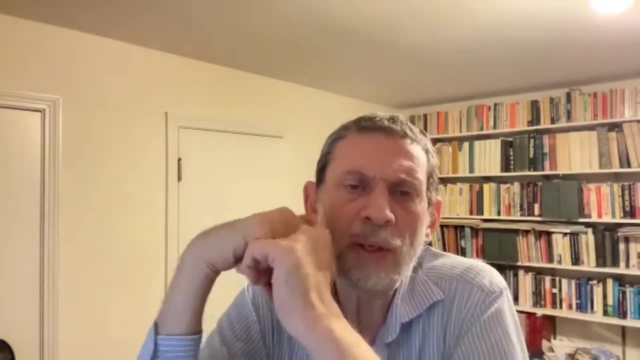 have, And if you were able to actually, instead of having to manufacture devices, you could develop them, that would be amazing, astonishing the kinds of things that could be created under those circumstances. So any of these things are going to be very powerful, And if you were able to. 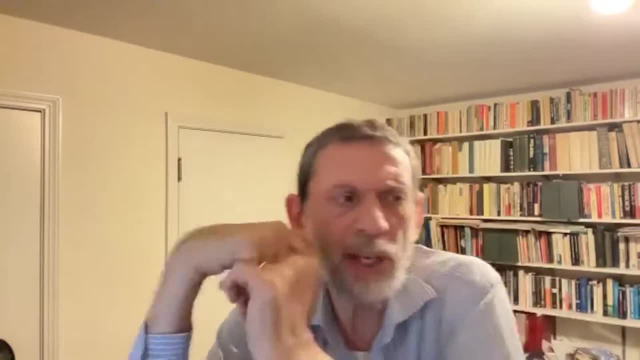 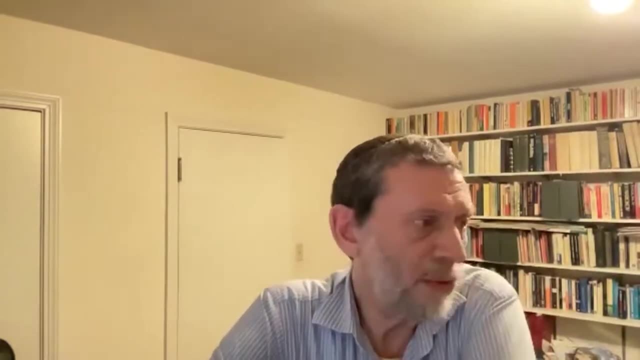 do that, that would be very powerful, And if you were able to do that, that would be very powerful. And any time you have deeper understanding at the systems level of what is actually going on, your possibility of engineering things either using biological materials or even other materials, 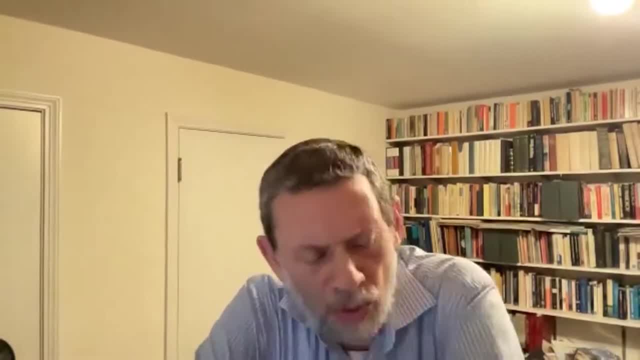 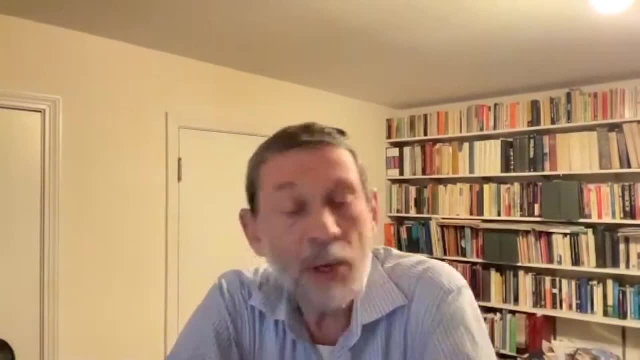 silicon and creating new devices is hugely enhanced. I didn't talk about this, but I have for many years been collaborating with Roger Quinn in mechanical engineering and, more recently, Katie Del Torio, And we've been focused on biologically inspired robotics. 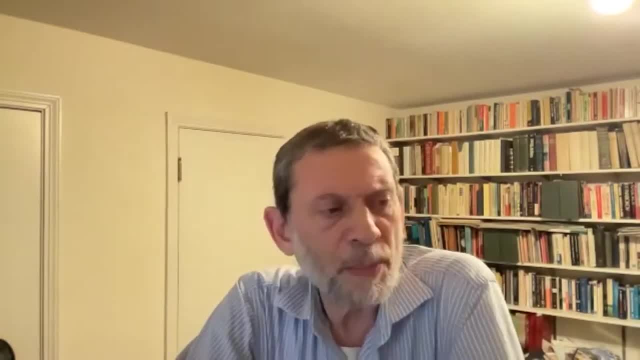 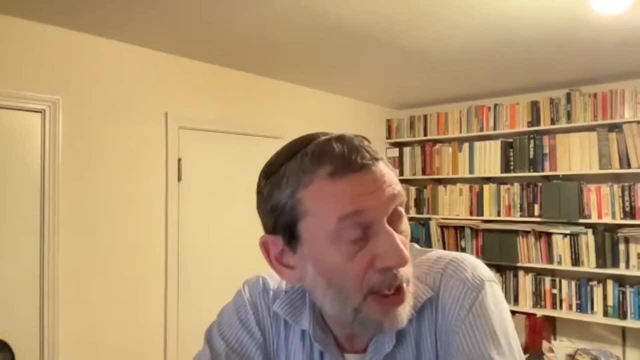 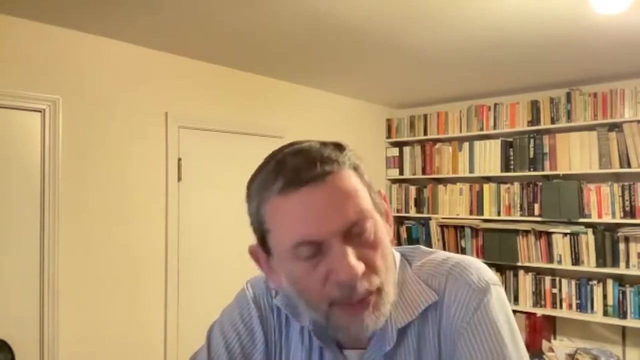 And these are robots that incorporate various kinds of biologically inspired components. So one of the things we did actually now back in 1994, we showed that if you had a six-legged robot and you incorporated reflexes, it could handle incredibly irregular terrain with very 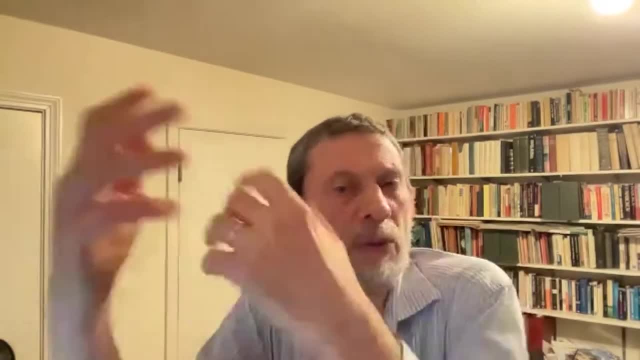 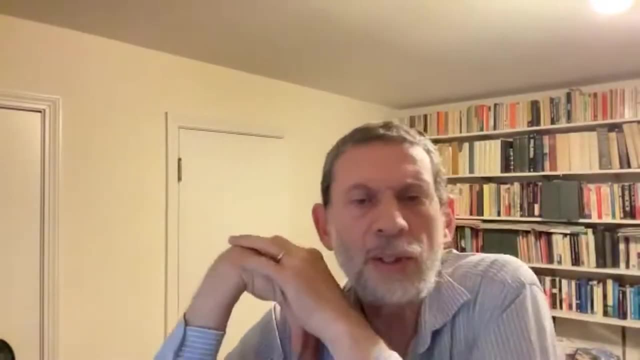 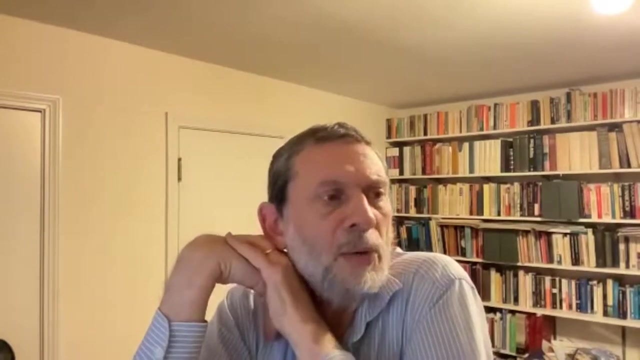 little difficulty. So that's where you take the ideas from biology, you apply them in an engineering context and suddenly you can do things that engineered devices previously could not do. So it's a very, very powerful area, And the more you know systems biology, the more comfortable you are. 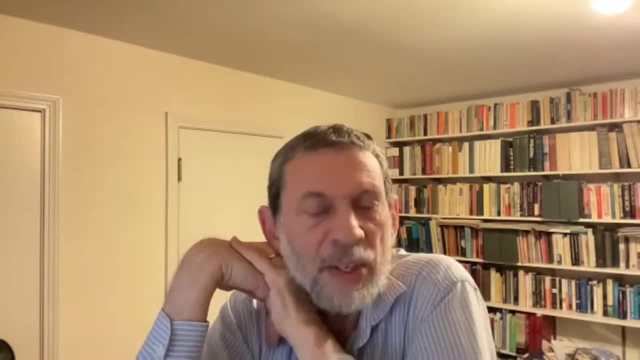 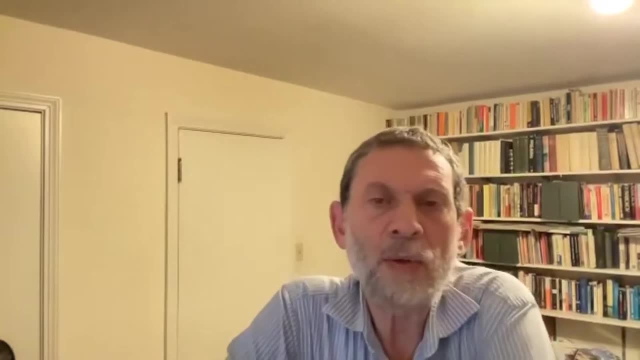 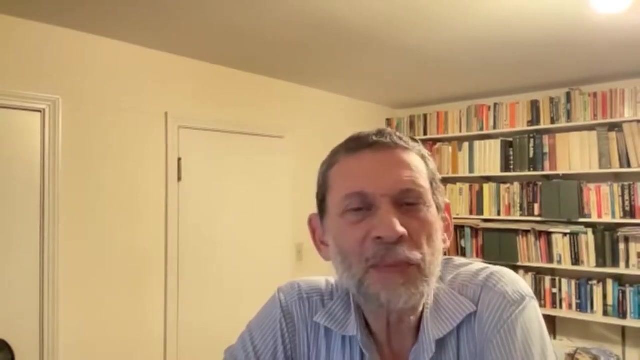 collaborating with engineers and being able to speak their language, so they can take what you know and turn it into an engineering device or yourself become a synthetic biologist or bioengineer. Any other questions? Yeah, I actually have one too. back a little bit more general. 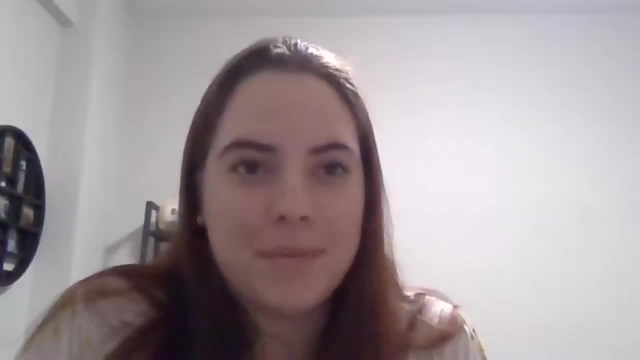 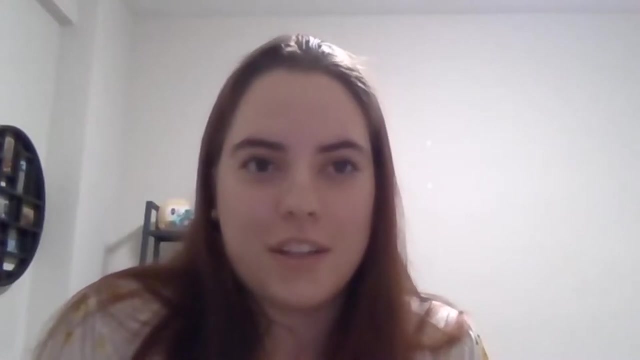 So we've talked a lot about all the problems that are potentially solved with people who know systems, biology and all that, And I was just wondering what your opinion is on why the major is still kind of small after so many years. I was thinking that at this point, technology 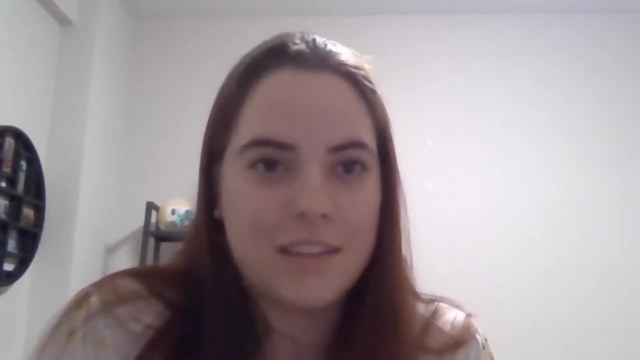 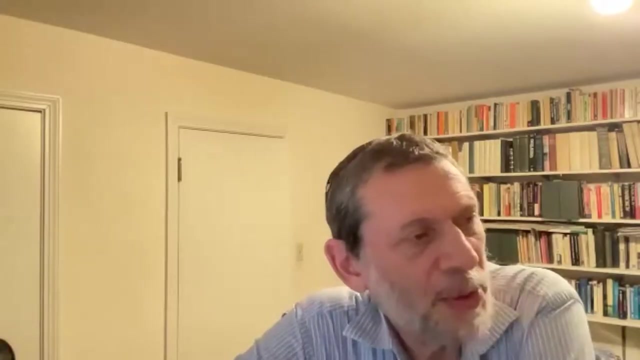 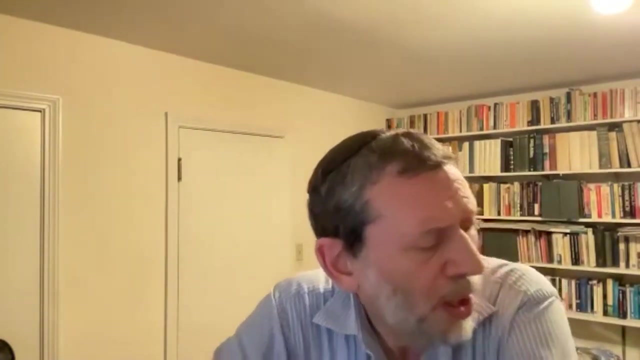 like. we know that technology goes hand in hand with any science and everyone's using it, So why wouldn't more people be interested in doing this? So that's a wonderful question, And I've thought about this as well. Here's the issue. First of all, there's the publicity issue. 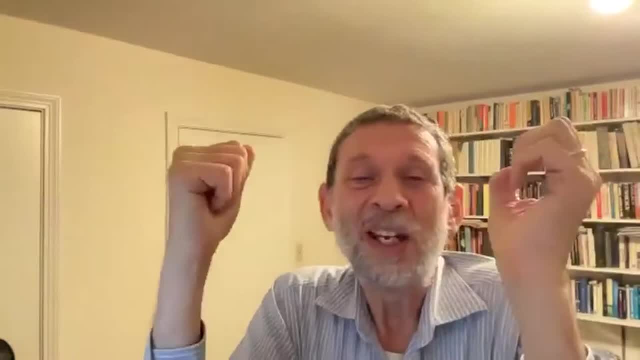 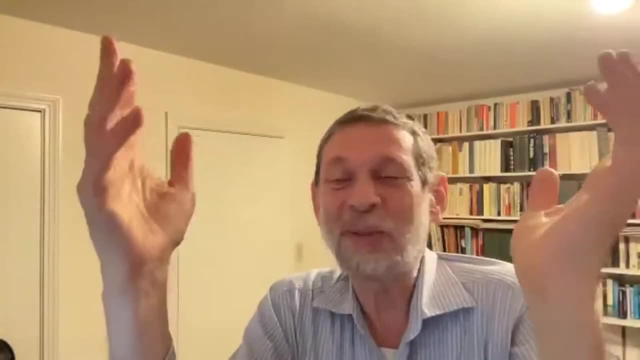 So you're the best ambassadors If you tell your friends this is the most wonderful major and they've got to think about it when they're about to declare a major, you could see a doubling or tripling of systems, biology majors. But the answer is: 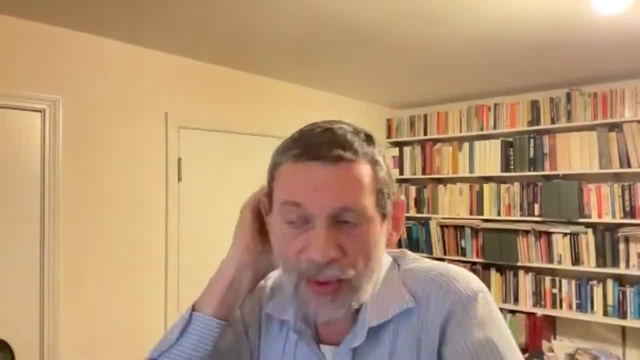 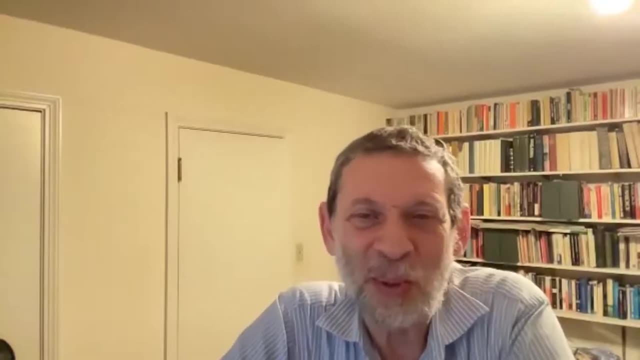 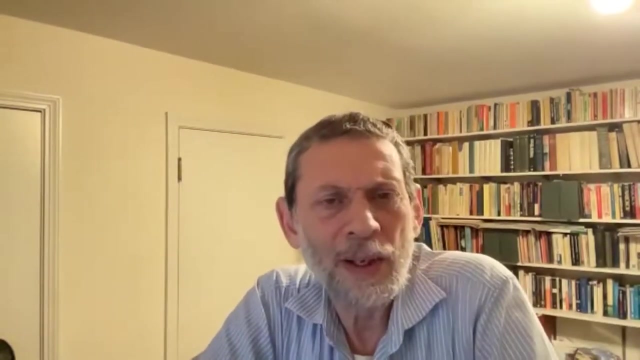 and this is what I sort of hinted at earlier and this is why the courses I teach are a rather rocky adjustment for most of the students. in those courses I'm trying to put together the disciplines that have traditionally been very far apart, And people are really good at biology and they know that from high school. 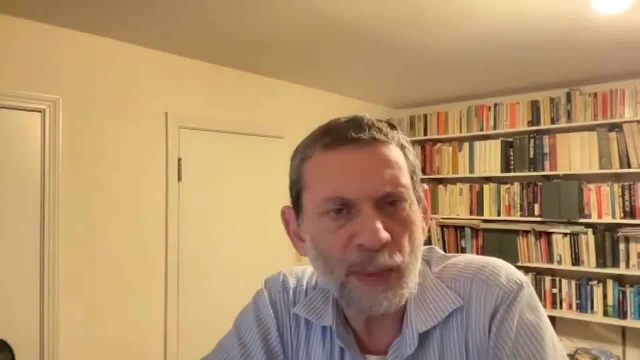 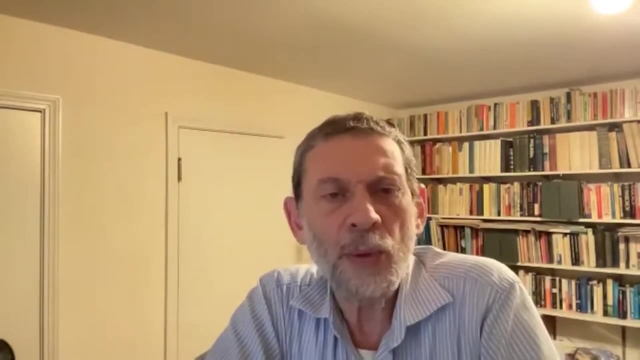 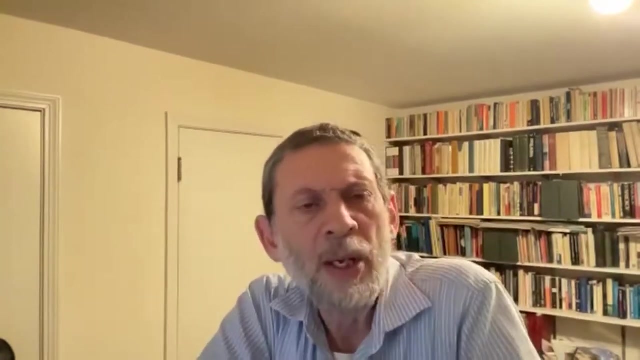 we're fascinated by the different structures. They have no problems memorizing all these different, complicated names. They probably want to be a doctor or they'd like to study some aspect of how biology works, And they often are very repelled math and computer science because it seems to them to be a conspiracy to convince them that. 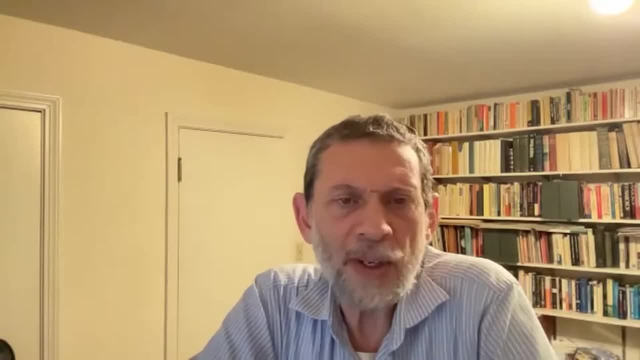 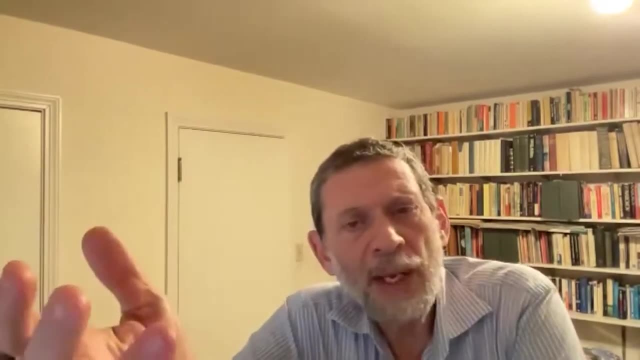 they're idiots And the people who know how to do it well are very impatient with them and don't sort of seem to be able to communicate in a way that makes sense to them. And vice versa, people who are math or computer science people are very good at thinking in their head, seeing abstract. 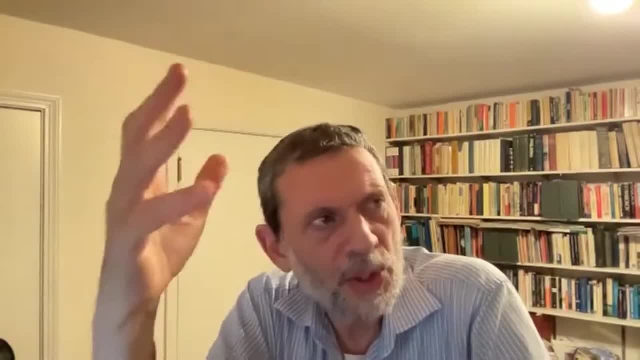 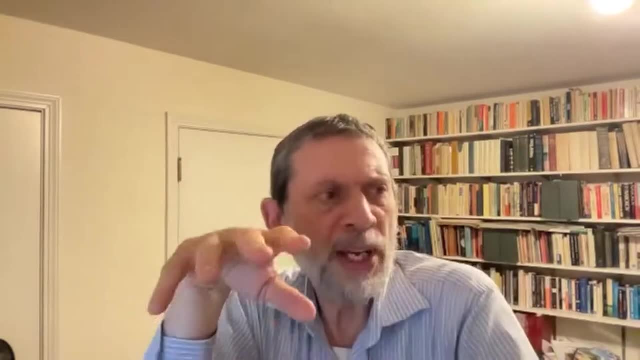 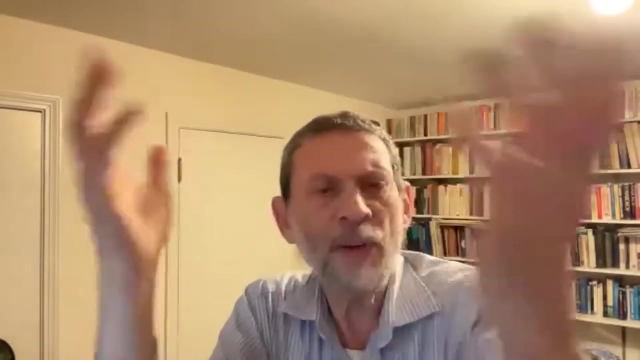 patterns and being able to get the intuitions in that abstract way and then figure out how you potentially could show through a proof that that will be true for all cases. And that's very, very difficult to do- all cases, not just exceptions to the rule, And they get very. 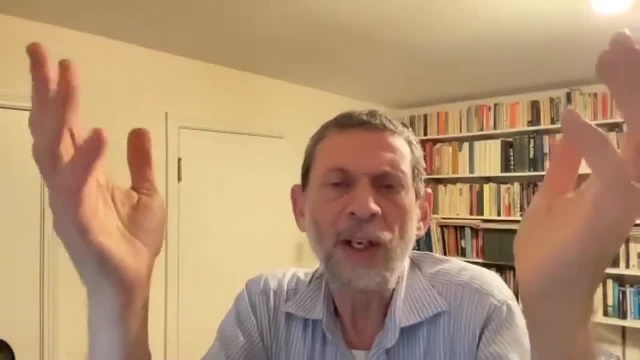 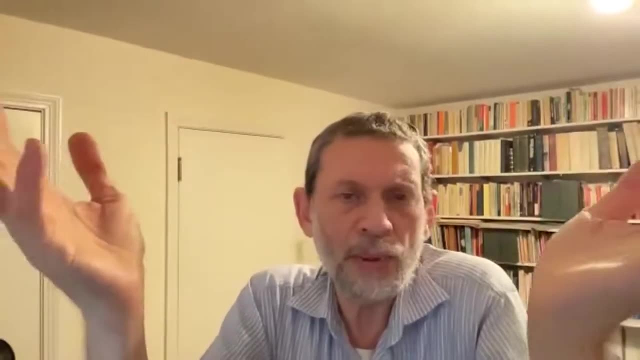 impatient with biology, because it's all exceptions and it's all arbitrary. Why is leucine called leucine And why is isoleucine called isoleucine? Why is the pituitary called the pituitary? I don't know. They thought it was a mucus secreting gland. I mean, it's all. 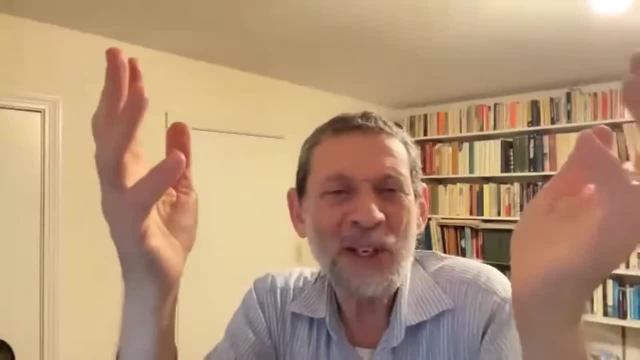 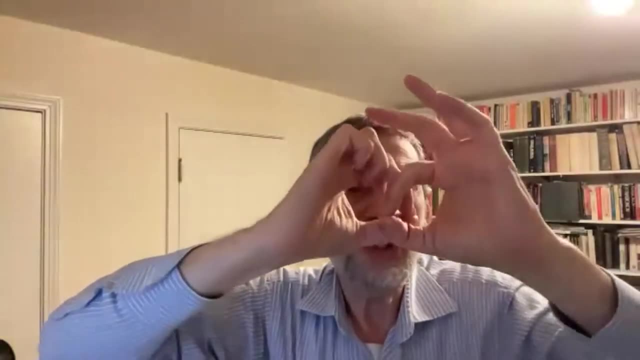 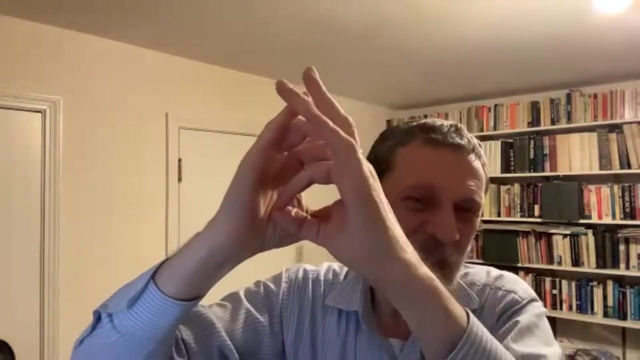 ridiculous and you have to memorize all this crap to be able to talk about biology. So what happens is that you're talking about the intersection of two sets And if you think about the Venn diagram, that intersection is not close to being the set. 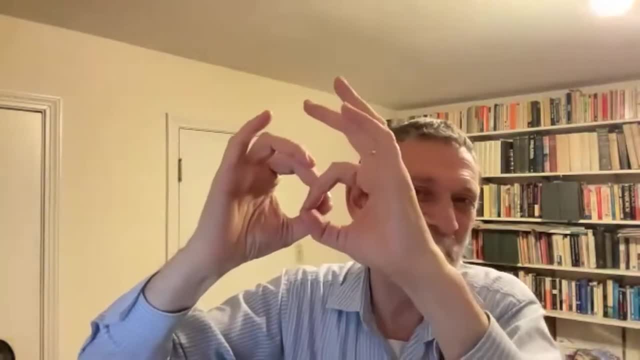 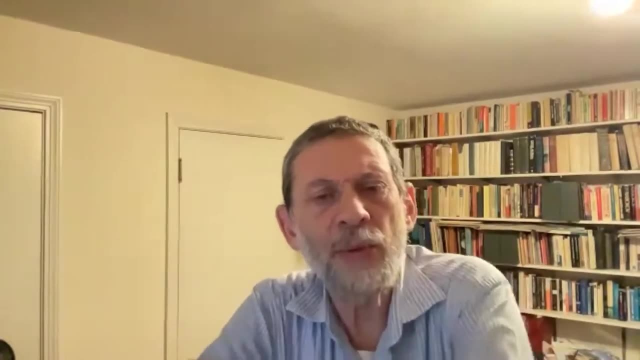 of all elements in both sets It's a very, very much smaller intersection. So that's another way of saying it's pretty hard to do systems biology, but it's very worthwhile. But again, you are the best ambassadors If you see this as something that's valuable. 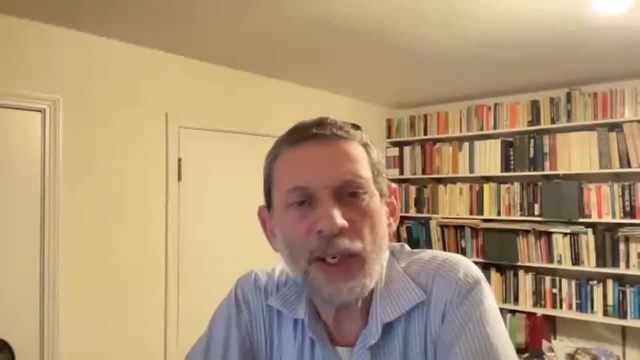 and you're going to do it. you're going to do it, So that's another way of saying it's worthwhile. You should be telling people this is really the most exciting thing you could do with your life And if you're interested and you can emphasize the point I made to Jillian, you're not. 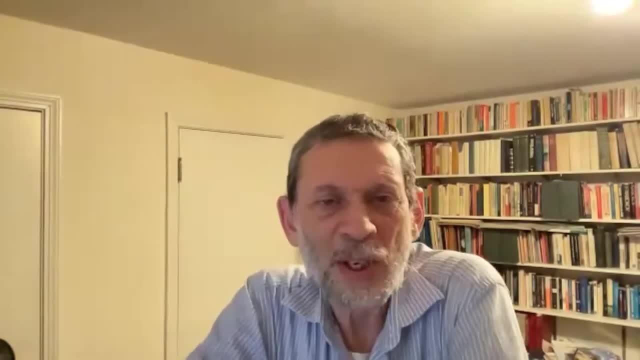 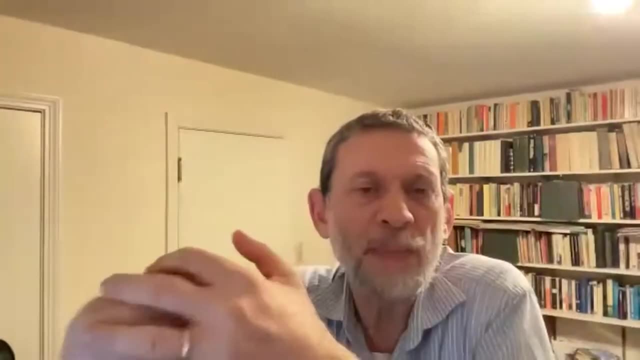 locking yourself into anything. by being a systems biology major, You can go to medical school, You can become an engineer, You can become a business person and get an MBA. None of that is precluded by being a systems biologist And you got a BS, which is a professional degree, So you go into 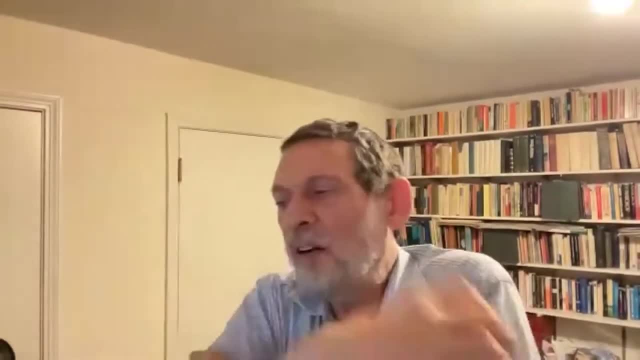 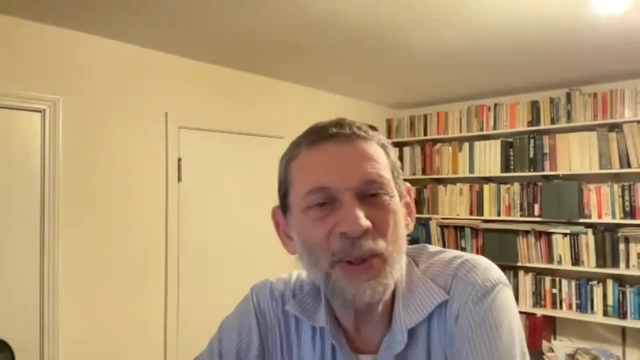 government. If you go out and tell people that again, a lot of people find that the major is hard. They ask: what are you taking? Well, I'm taking the more advanced physics, I'm taking the more advanced math, I'm taking computer science, I'm taking databases. They say, no, this is not. 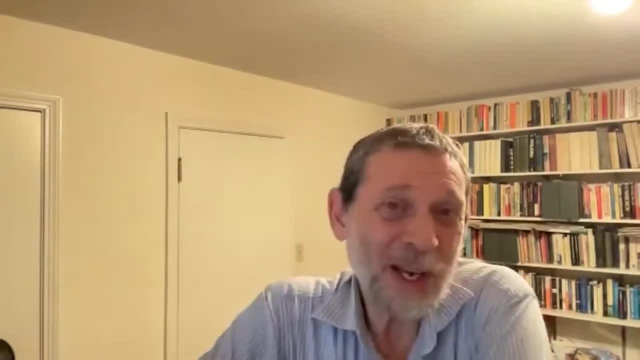 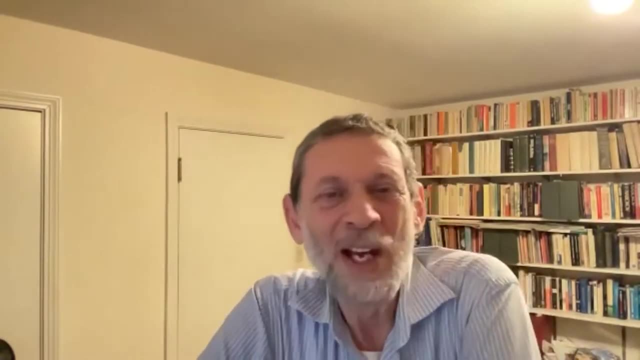 for me. I'm sorry, Forget it right. So I think that's what's happening: that people look at all that and they say this is just too much coursework of stuff I'm not going to be able to make sense out of. I want to be able to live and breathe as an undergraduate, So this is not for. 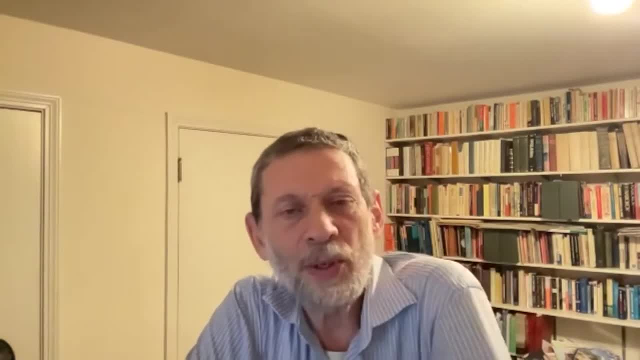 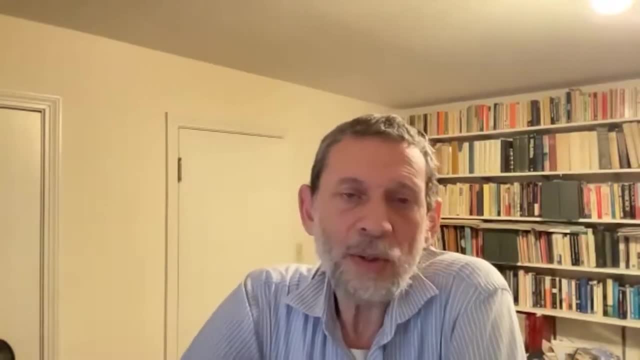 me. But if, on the other hand, you have this larger view, which I try to present, why it's important to master these things, how valuable it can be, then I think that's useful. One of the things that I like very much about teaching Bio 300, and this happens almost every semester. 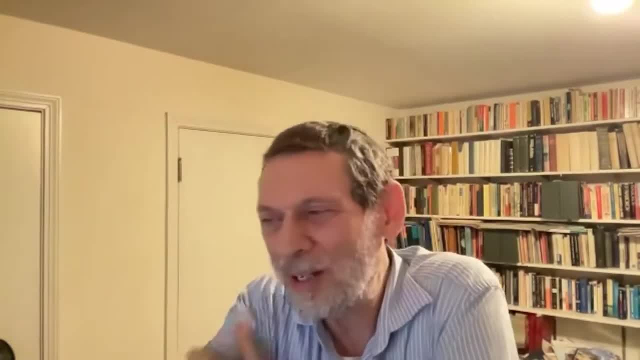 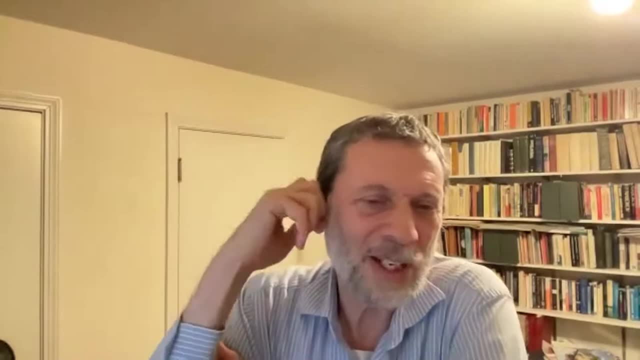 a student approaches me and says: you know it's during ad drops, you know I'm doing the exercises. I really don't know if I can do this. So I talk to the student and I get a sense of their background and I get a sense of who the student is and their level of you know dedication. 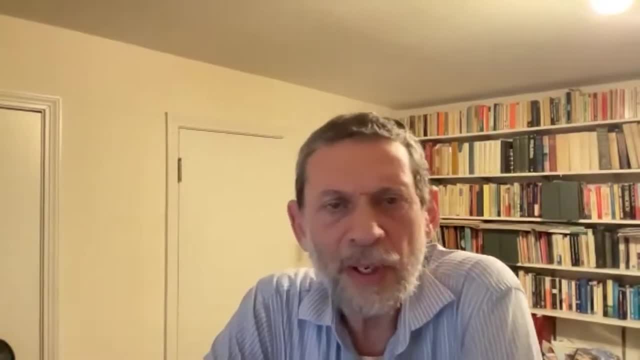 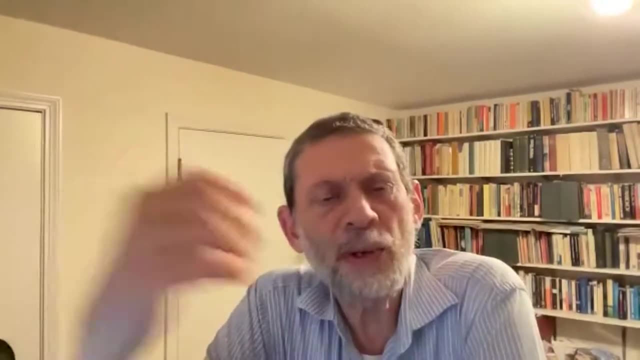 their motivation And if I see that they're really smart and super motivated, I say you're going to be able to do this, Don't worry about it. If they seem to me someone who- just you know it is hard for them to grasp more abstract things at all, then I might counsel. 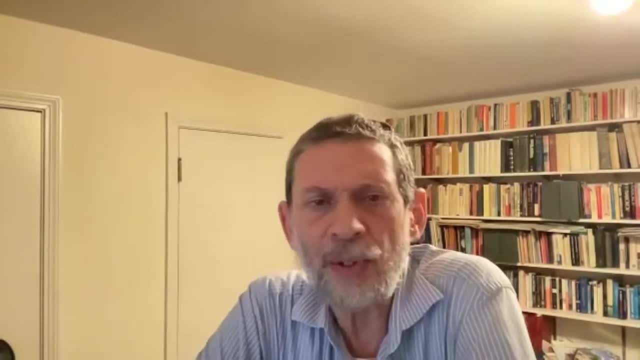 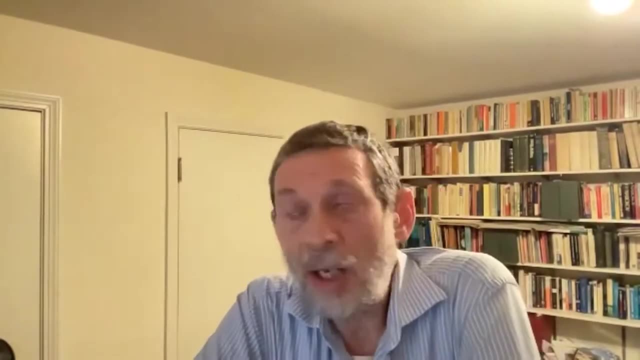 them and agree with them that it doesn't make sense. But the majority of times I have that conversation, I encourage them to stay And generally I think I can say without exception- actually- they come back afterwards and say, wow, thank you so much for encouraging me to stay on. 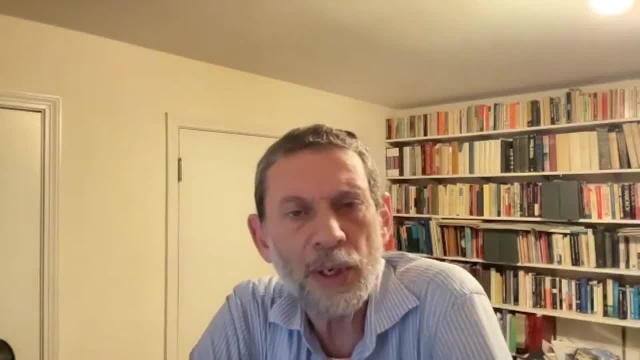 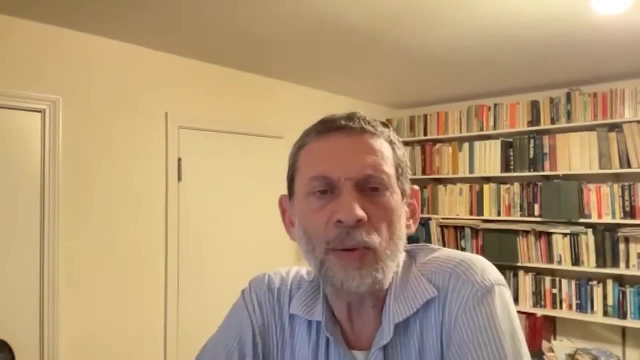 I really loved it and now I know I can do things that I never thought I could do. But you see, that's part of the issue. A lot of the courses are not taught the way I teach, And so, if you sit down in a math course, 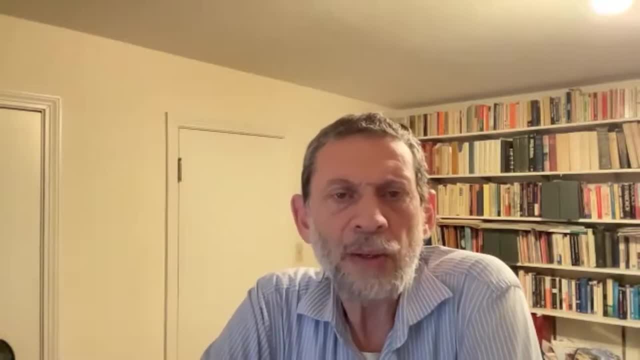 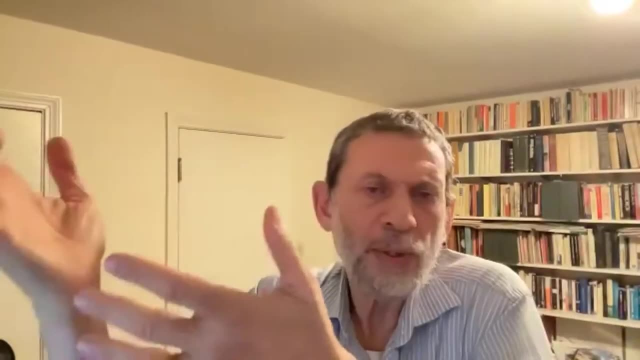 you're not properly prepared, you don't have the support system and you're not able to follow what's going on. from the very first lecture you're just going to wash out. And in computer science, if you've had no experience, I mean it's so frustrating If you come in as a I don't know. 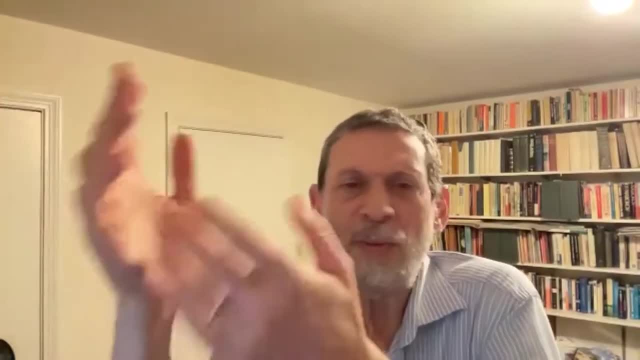 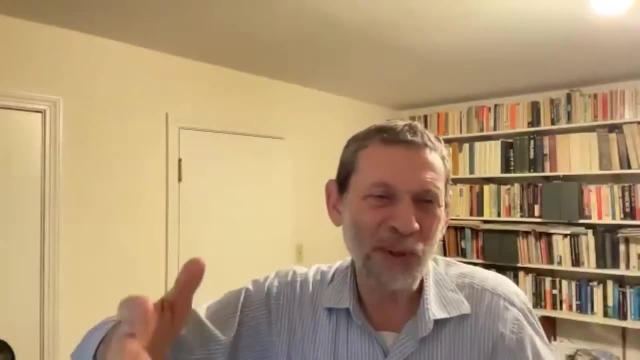 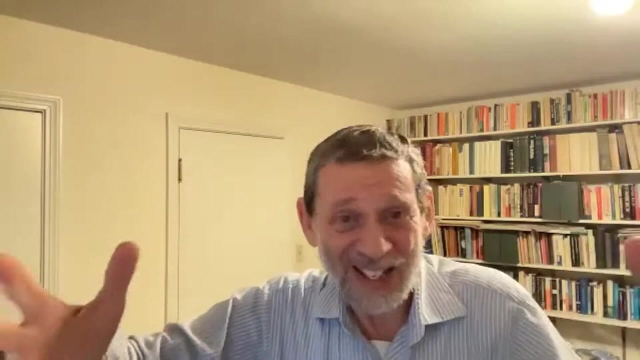 freshman and you sit in COMS 131 or whatever appropriate course. you're surrounded by people who, when they were 10, got their first computer and started not just playing video games but programming them. And then they've gone and done hacking and they are all into the 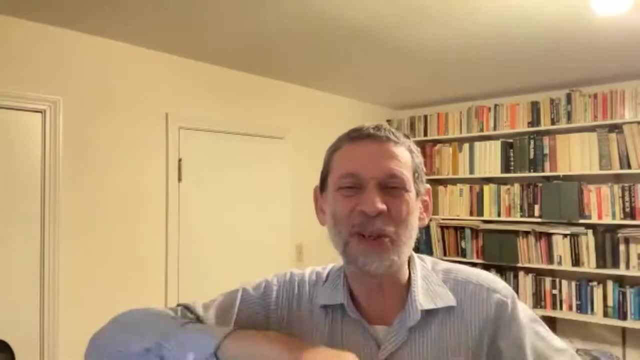 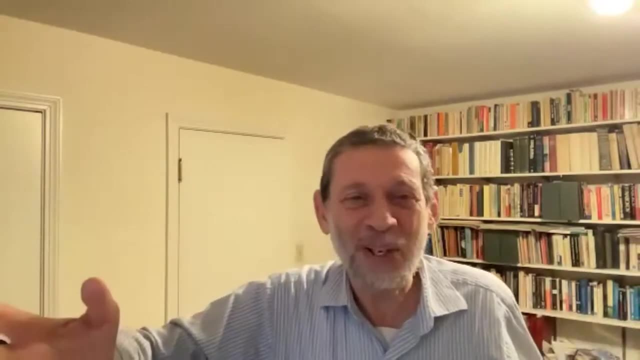 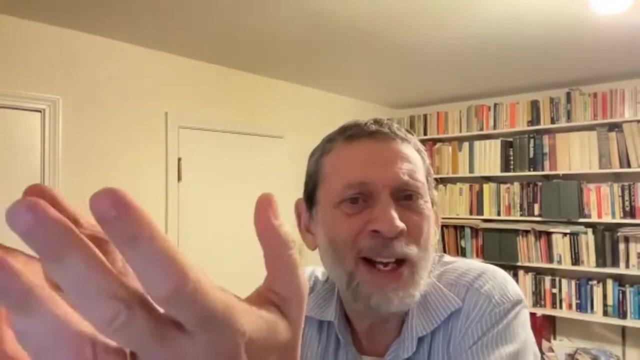 cryptocurrencies, and they're part of these communities that are doing machine learning And you just have a conversation with them and you freak out. They've got 10 years or eight years of experience and you're just starting to learn Java or MATLAB. Oh my. 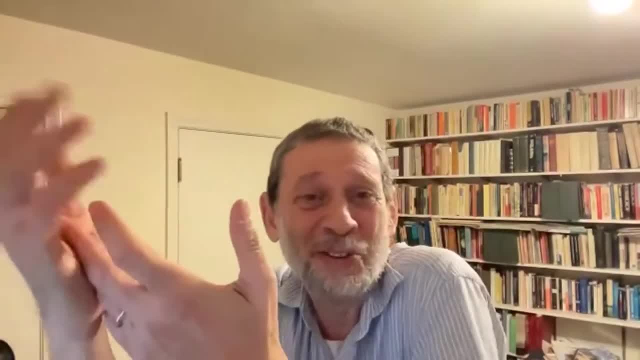 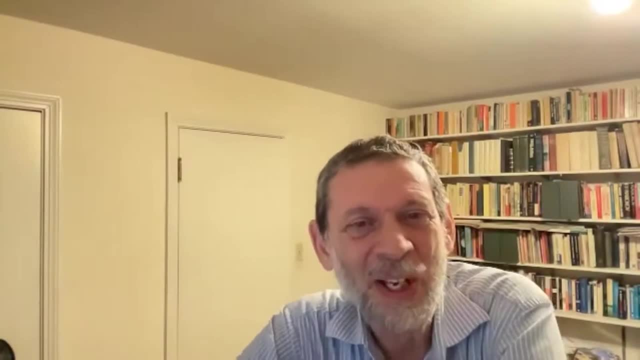 Right. So how does that make you feel? It makes you feel like you're an idiot. So you come into that situation and unless you're a very brave and courageous and persistent person who knows that he or she has to master this material, you're going to just say: this isn't for me. 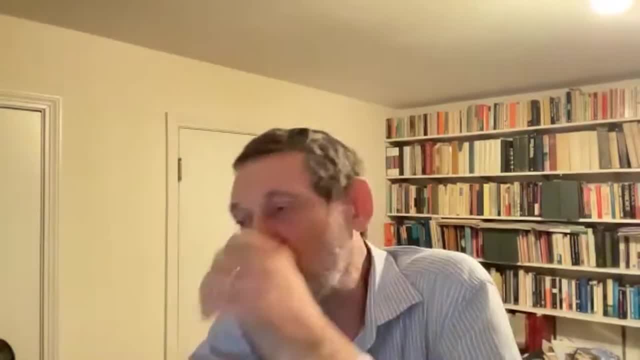 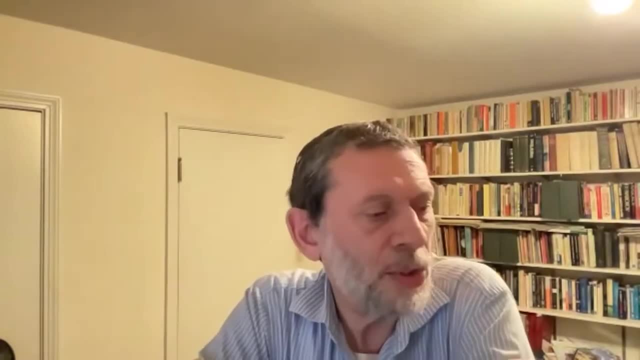 Okay. So again, I think that's part of the reason we have such problems attracting a large number of people. But part of the reason I'm not worrying so much about it is that the major has slowly but steadily gotten slightly larger, And I think that's part of the reason I'm not worrying so much. 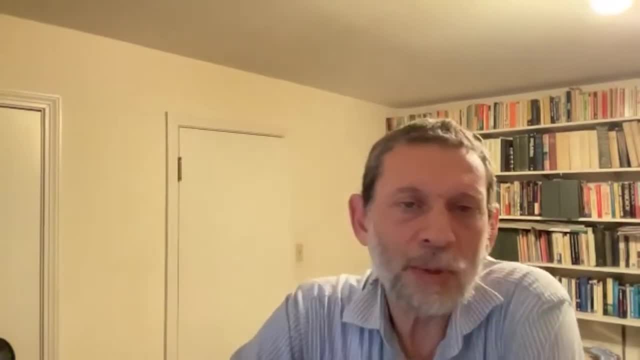 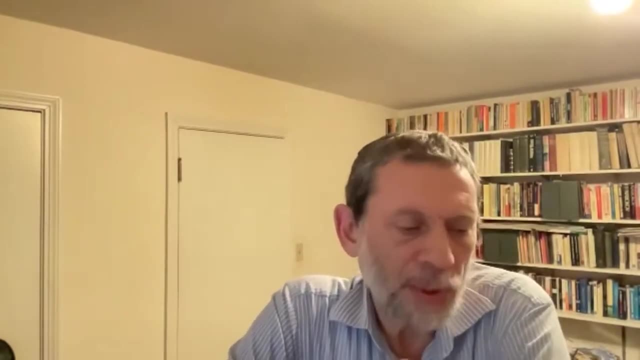 about it is that the major has slowly gotten slightly larger over the years, And one of the things that I've noticed- which has been wonderful- is that there are usually enough people coming into the key courses, that those courses have high enough demand, that there's 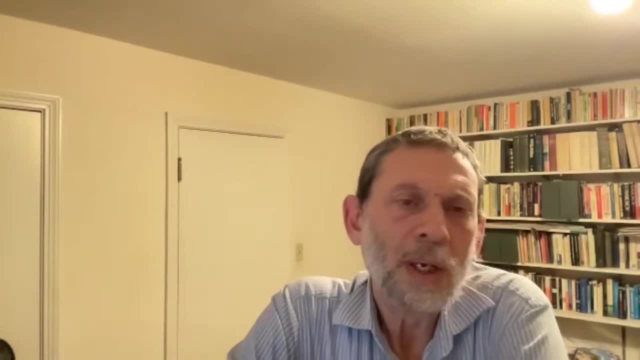 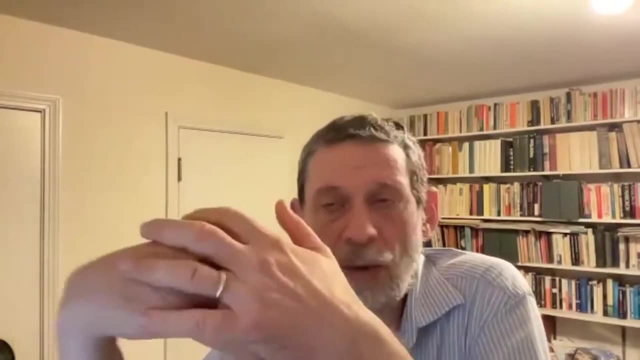 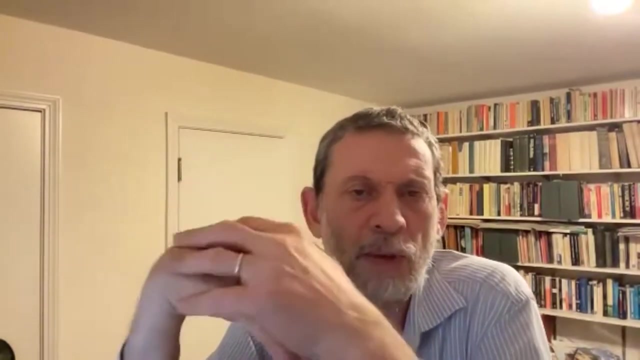 no risk of their getting canceled. So as long as we're able to bring in enough people so that we populate these key courses, the courses will continue. But I go back to this: Each student in systems biology is really our best ambassador, And if they want to talk about how wonderful it is, 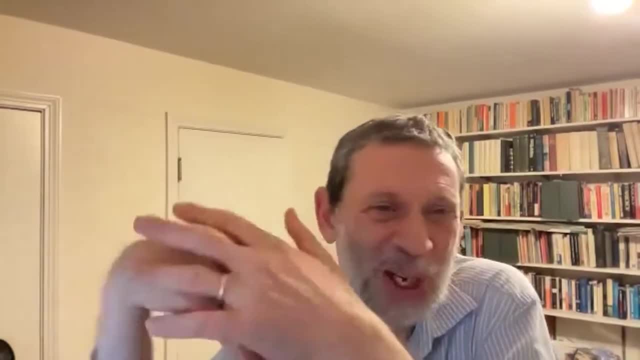 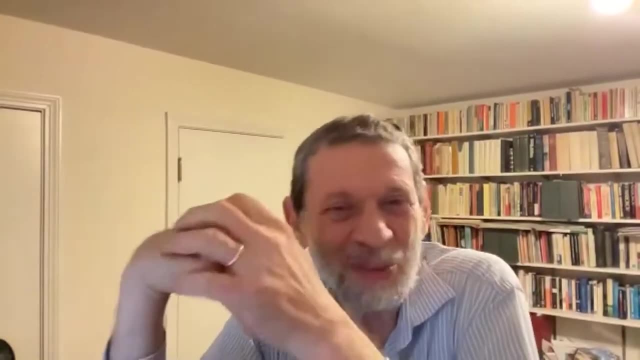 and how great it is. Now don't lie. If you had a miserable time in Bio 300 and you hate 306 and you think that Dr Steele and Dr Snyder are only interested in torturing students, then don't invite other people to become part of the major. But if you see us as actually really caring about, 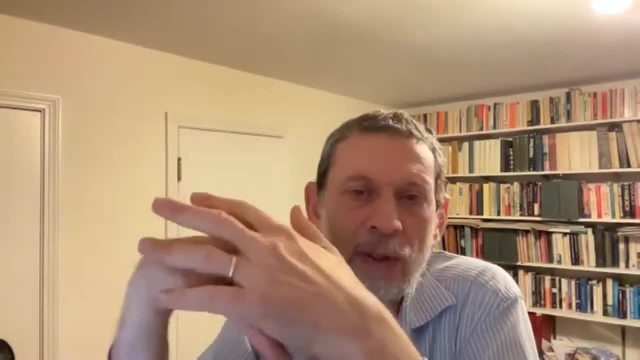 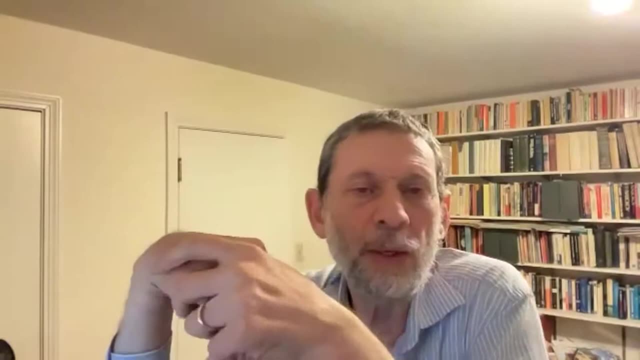 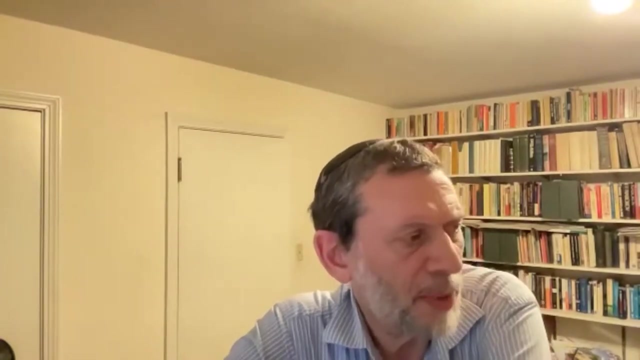 giving students these tools and you can convince your colleagues, your peers, that having those tools would be incredibly valuable. then that could increase the number of majors. I think the problem is, per se, the way the major is structured. I think the major has the right. 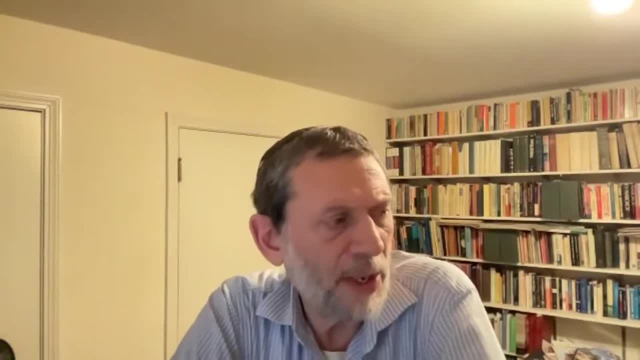 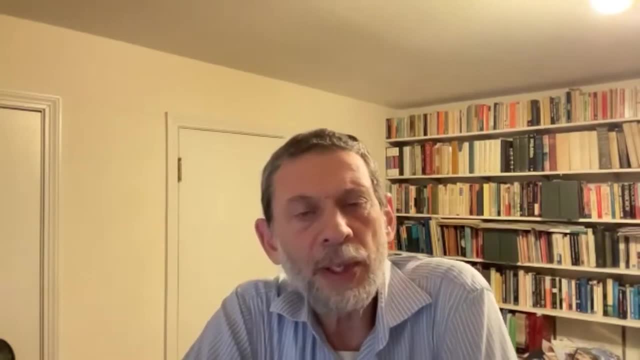 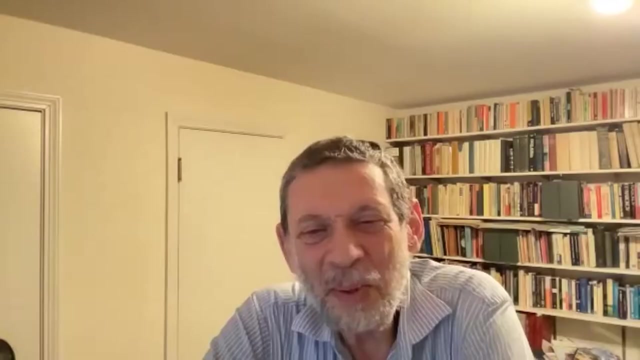 things in it. I think that, as I said, the Venn diagram of the intersection of those who have biology backgrounds or more abstract backgrounds is small And so inherently, it's a tough road to go. Thank you, Any other questions? I don't have a question, but based on that, 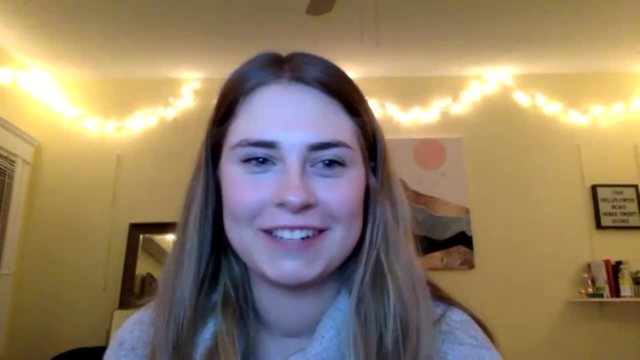 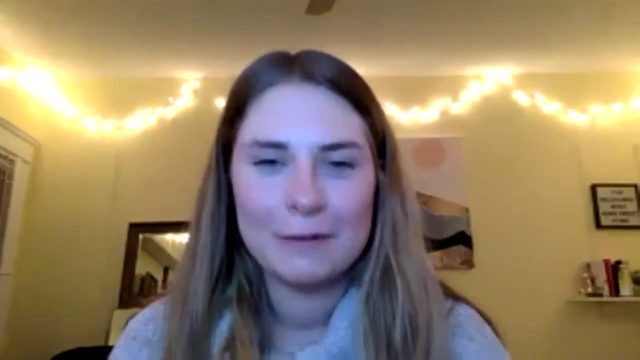 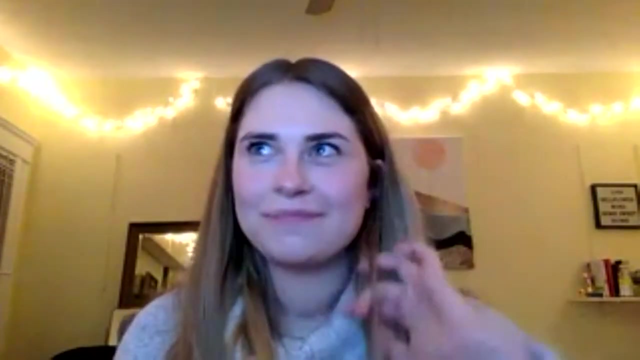 I have a small suggestion, maybe for those who were to come after us: if you were to ever reconsider adding a course or something. I very much related to your statement of feeling like an idiot in Java classes, because I just wasn't one of those kids. I wish there was a systems biology class. 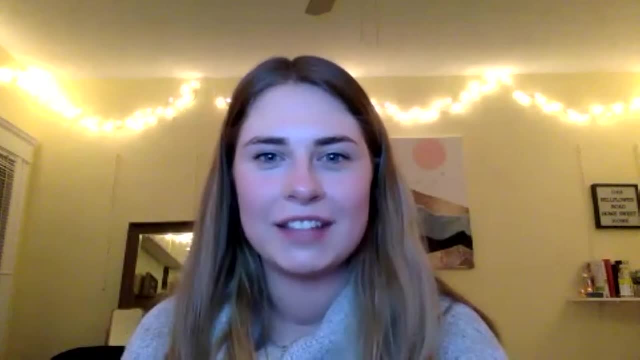 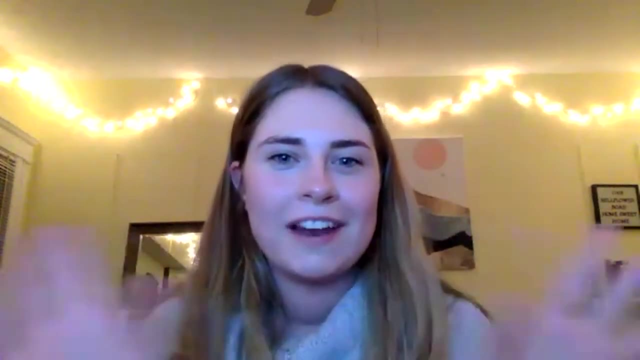 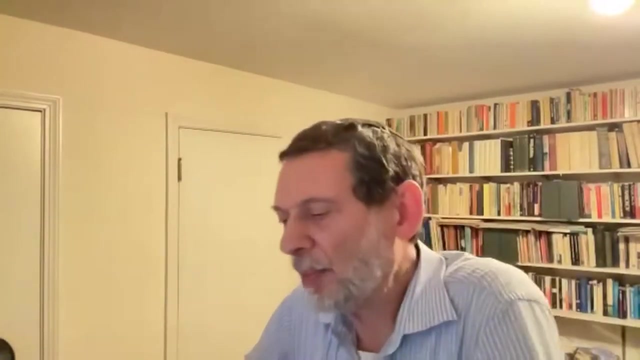 that didn't have any prereqs that we could all take when we first started, because I think that would have made me a lot happier as a freshman. So again, I'll discuss this with Robin Mounting such a course. So the first point I'll make is: 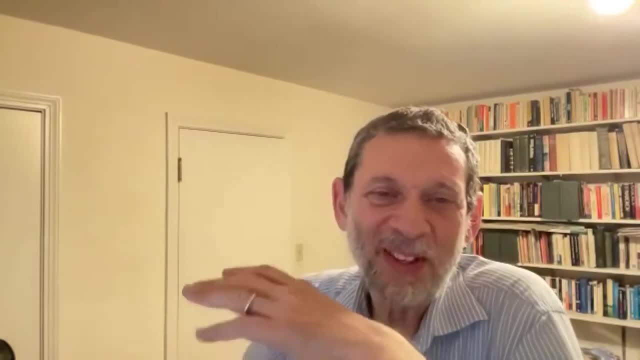 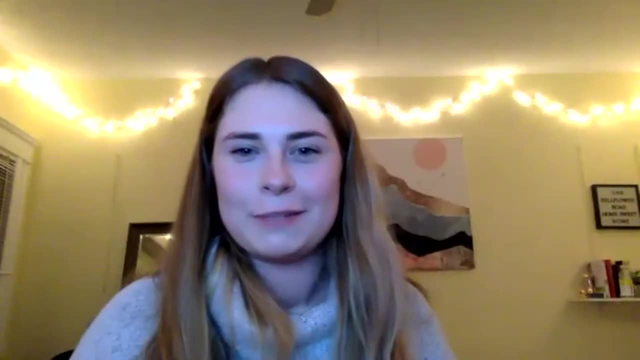 I don't know how many of you noticed this. Bio 300 has no prerequisites, That's true. Yeah, You can take it as a. I've had high school students take it. I think it's the 300 that freaks people out because you're a first year in. 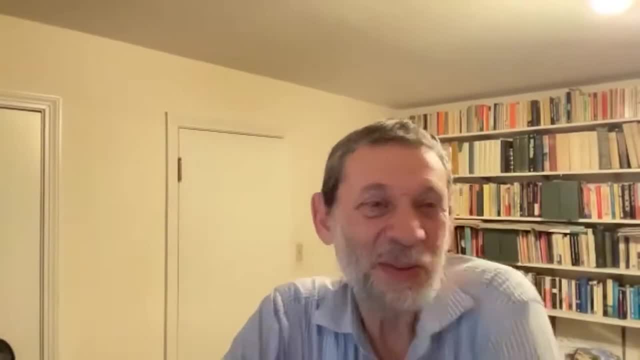 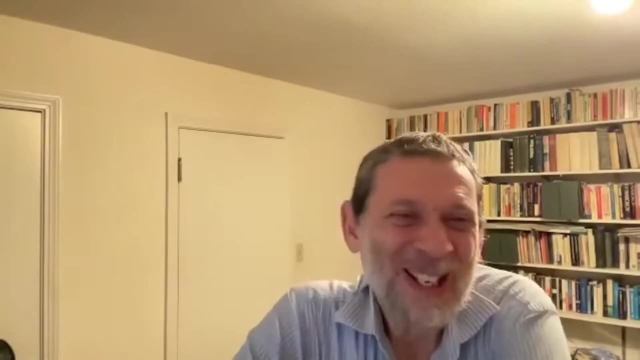 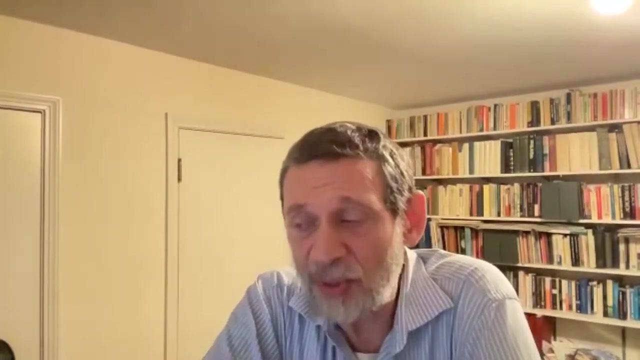 Yeah, again most. but I've had freshmen in the class who've done very well, Right, Smaranda, And no, it wasn't you, your teammate- And I've had seniors who've taken the class and have done very well And I've even had sometimes graduates, but I've had high school students have taken it. 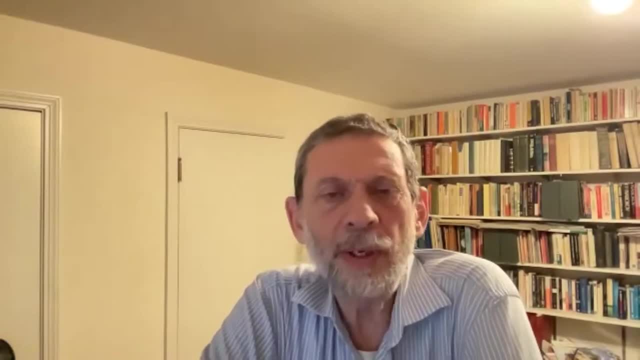 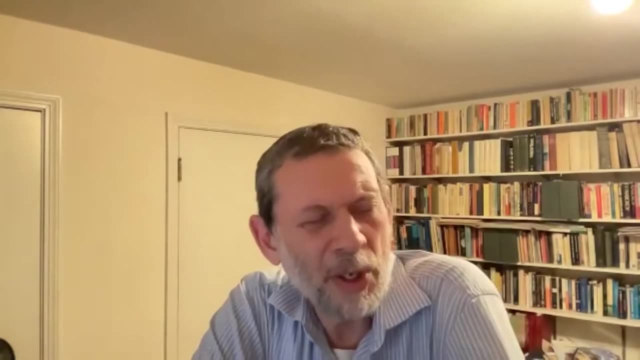 There are no prerequisites, and that's deliberate. I assume that nobody knows anything when they walk into the classroom, And part of the reason I tend to shy away from prerequisites is even when students supposedly have had prerequisites. if you ask them if they know it, they refuse to admit it. 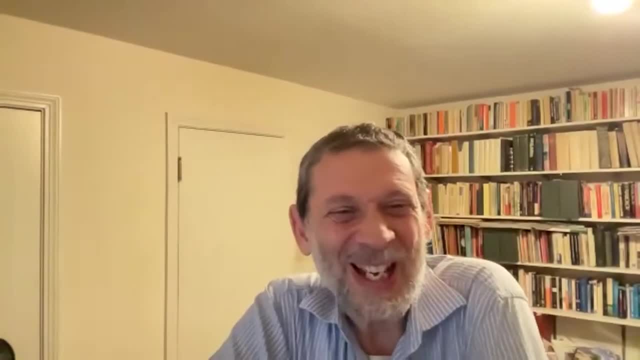 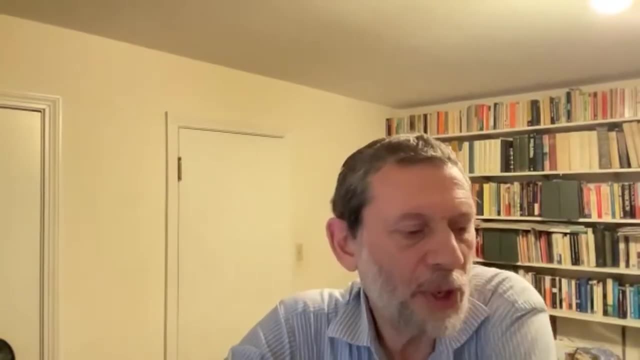 They'll recognize it. if you actually say things, They'll recognize that they actually saw it before, but they don't want to admit it. So the problem is: who would teach that course? If it was taught by computer science or math people, then they would see it as a remedial course which would 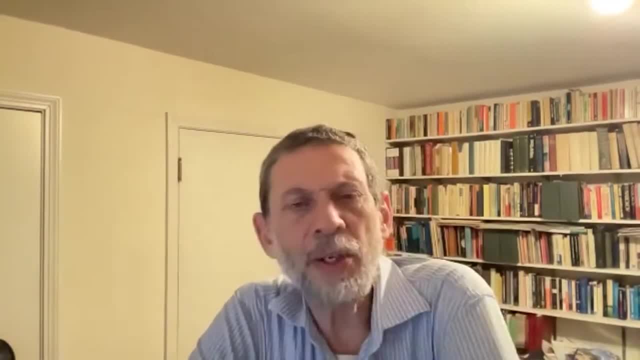 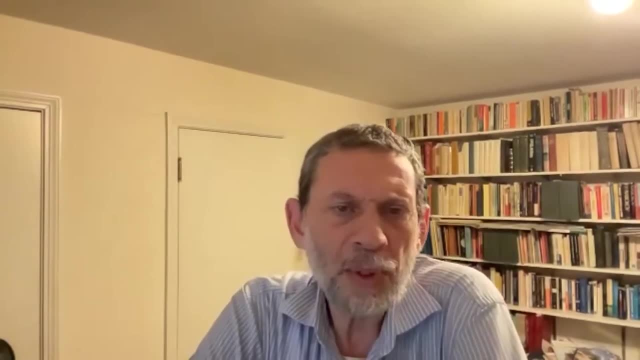 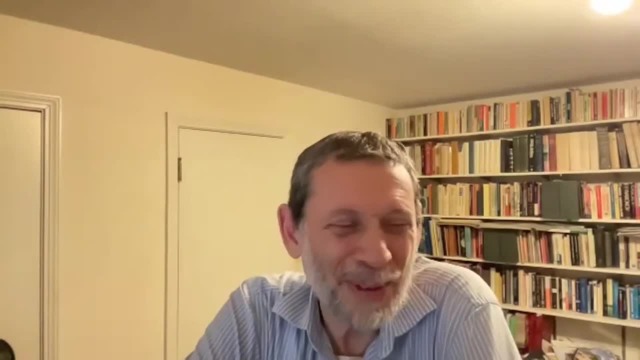 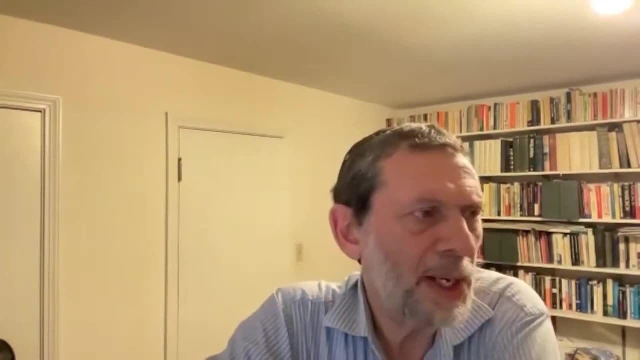 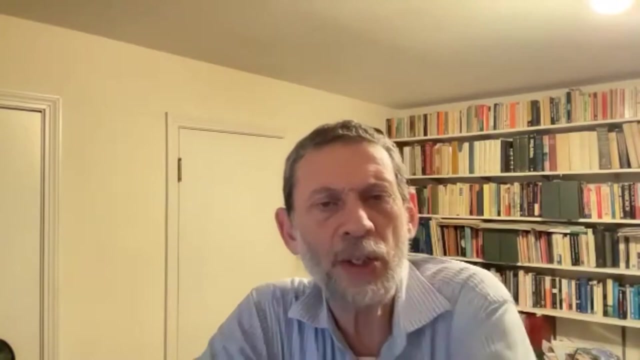 know in programming would be leery to learn about programming from a biologist Really, So it's hard to see who would offer that course. The other course that's a way in is the one that Jess Fox teaches on the design of experiments, where she teaches MATLAB and she has students actually build. 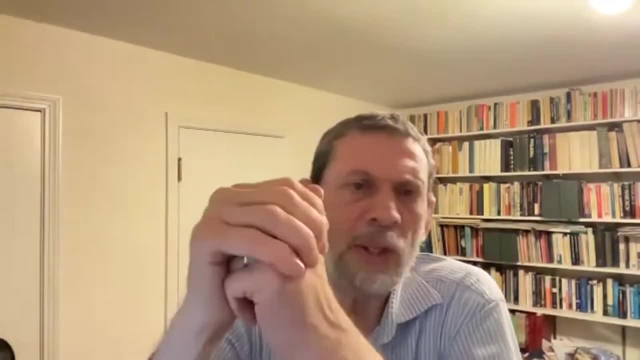 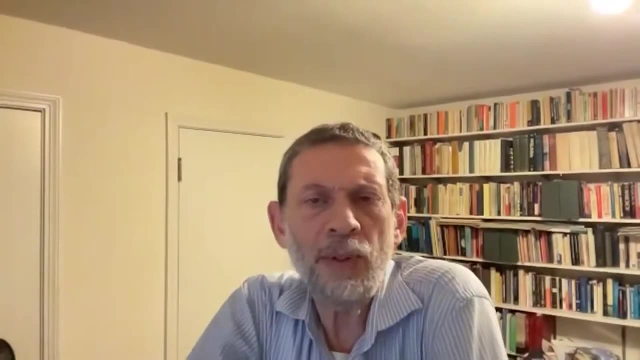 little devices and get data and analyze the data and so forth. So you're learning programming, but you're learning it in a gentle context in which it immediately gives you feedback for something that you are interested in. But, Jillian, your point is well taken. There's an